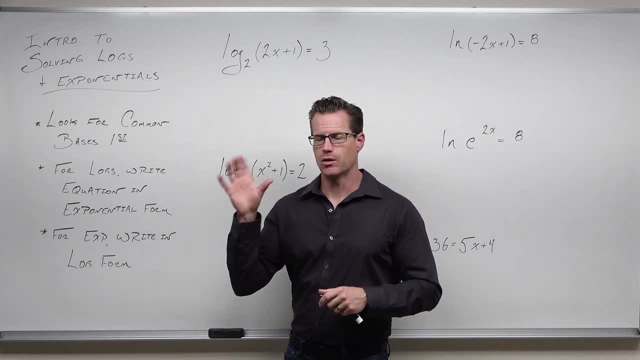 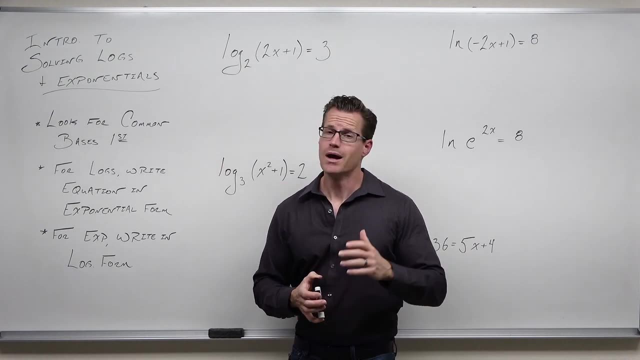 bases With logarithms. what that's going to mean for you is that you have a log on one side and a log on the other with the same exact base, and we can just set the insides or the arguments equal to one another. We're going to see that in a future video With exponentials. that means that 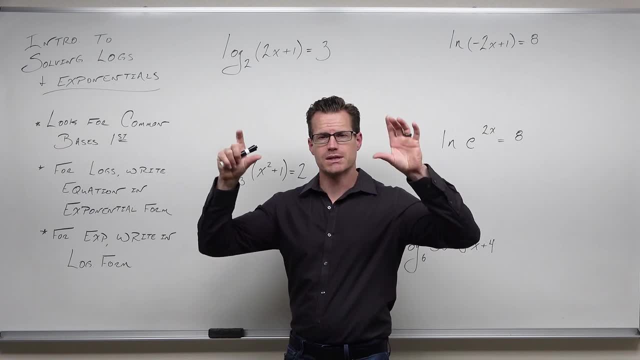 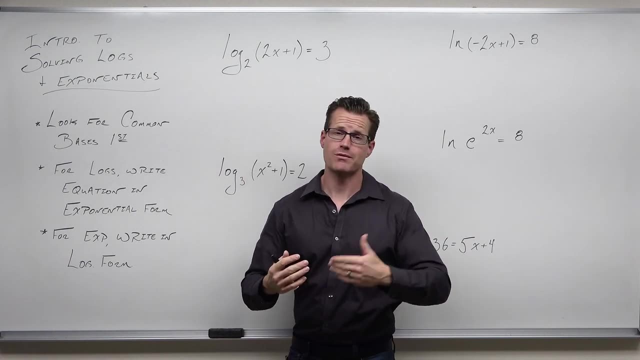 we might have to manipulate a little bit- and we've done that before- where we say: hey, this is an exponential equation, Let's get the same base and if we can, then the exponents are equal. We're not going to talk about that, because we've already. 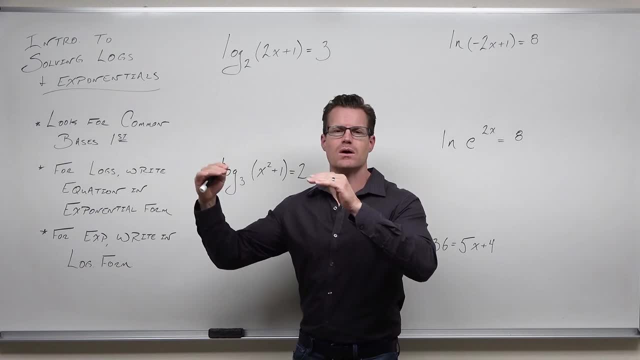 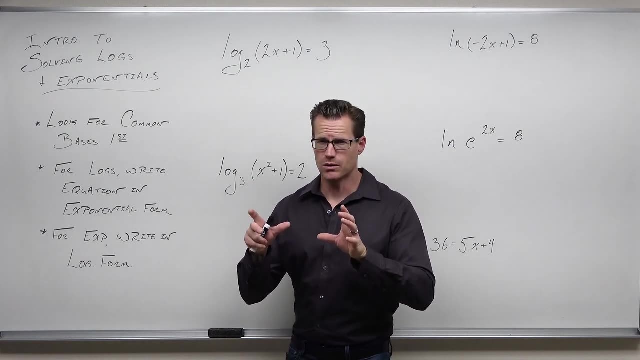 done that in a previous video Right now is: if you don't have common bases, what in the world do you do? So here's what we're going to learn in this video: If you have logarithms in your equation and you don't have two of them, you just have one logarithm and a constant. what we can know. 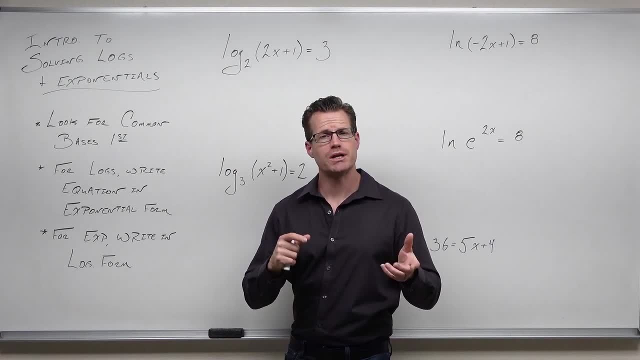 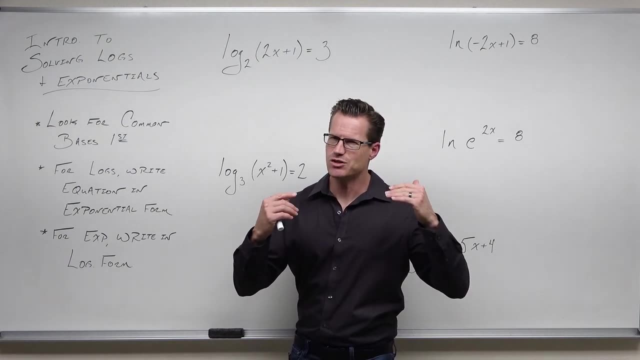 is that we can take any logarithm and change it into some exponential. It's inverse and in doing so we're going to solve that logarithm. So in your head, I need you really thinking. with the exception of common bases, 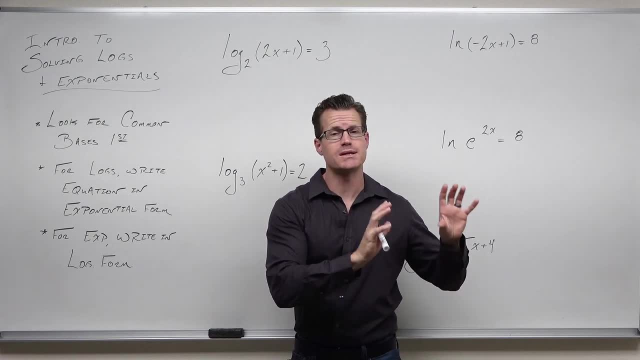 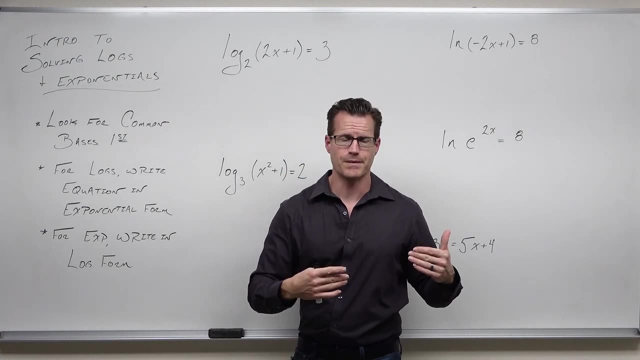 if I see a logarithm, I'm using exponentials to solve it, because that is the inverse. Just like addition is to subtraction, exponentials are two logarithms, They undo one another, and so we're going to practice that When we get to exponentials- with the exception of common bases, if you have an- 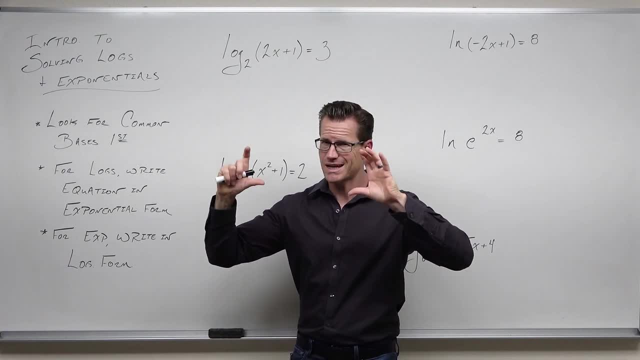 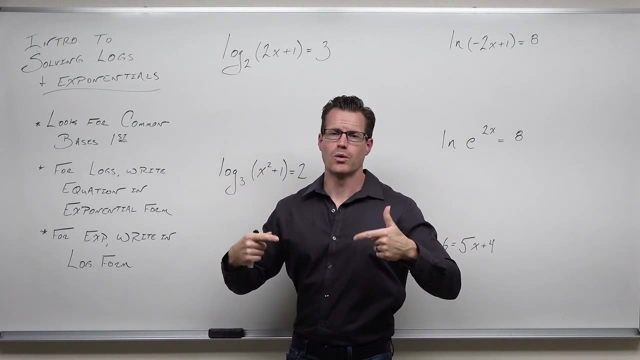 exponential, you're going to be using logarithms to solve it. So when we see exponentials, we're going to use a logarithm. It's inverse- and by writing an exponential in a logarithmic form, we're going to be able to solve that exponential. 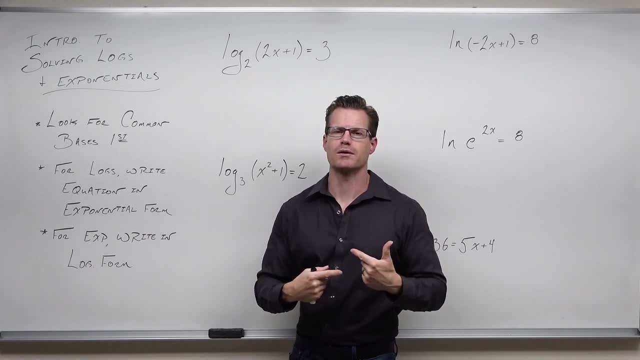 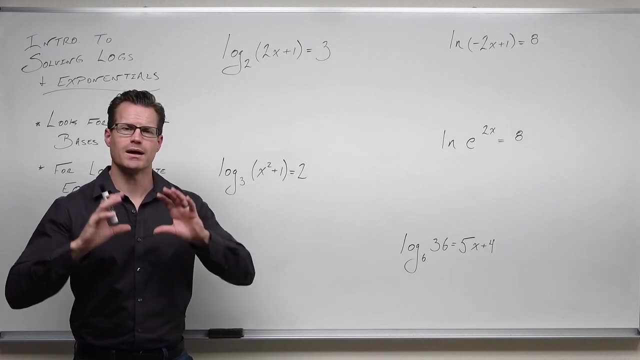 So I'm going to model this as we go through. These are going to be very, very quick. We're just getting a feel for it, understanding that exponentials are going to solve logarithms. In the next part of the video, logarithms are going to solve. 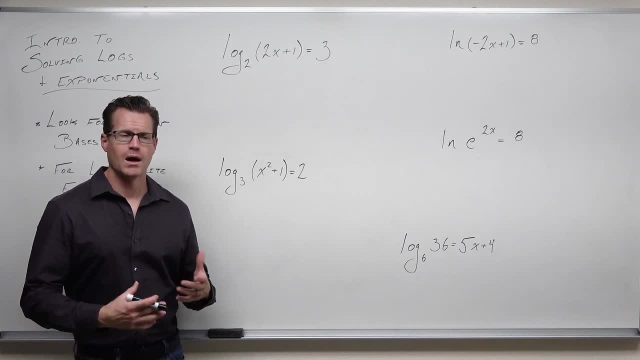 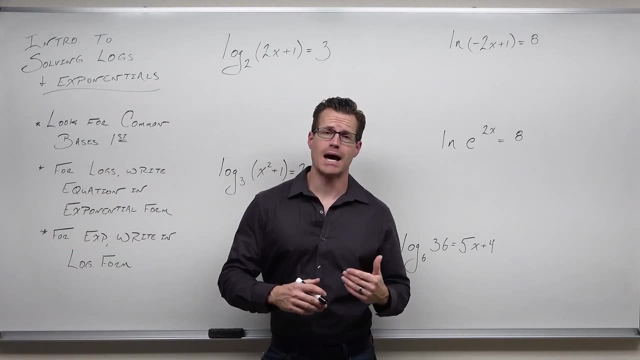 exponentials. So let's take a look at it. Log base two of 2x plus one equals three. So here's the thought process going through Number one thing we're going to check if we have common bases Now for logarithms. what that means is we need a log on one side and a log on the other side. 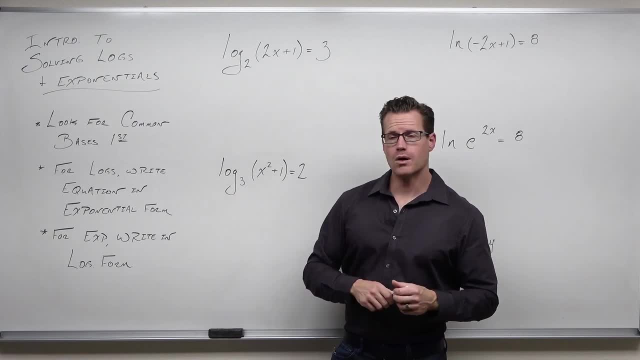 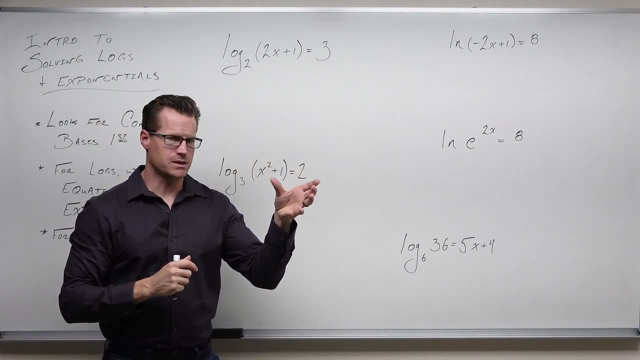 We don't have that. After that, we're going to look for logs, And if we have a log, we're going to isolate it. So we have a log on one side, nothing else around it and some sort of a constant on the other, which is what we have here. 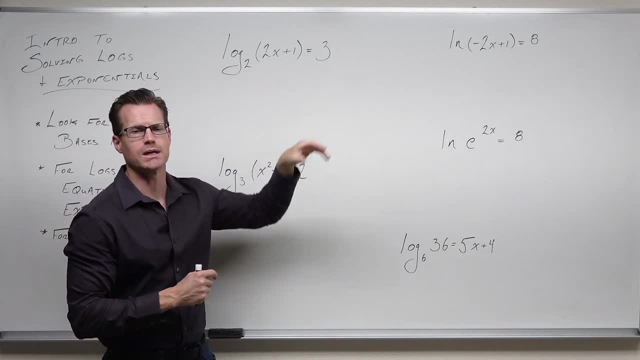 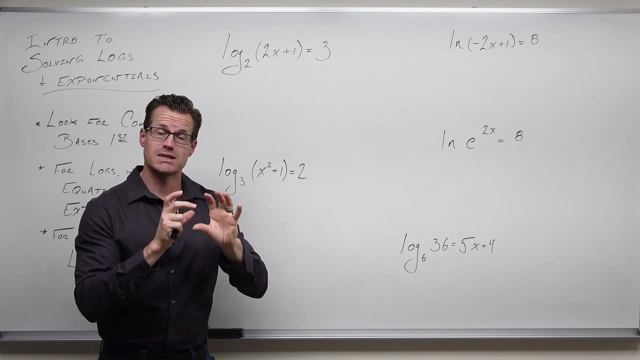 So we have a log base. two of 2x plus one equals three. Once we have that log isolated, we have our base identified. What we know is that logarithms have separated the base from the exponent. If we write this in exponential form, it will put it back together. 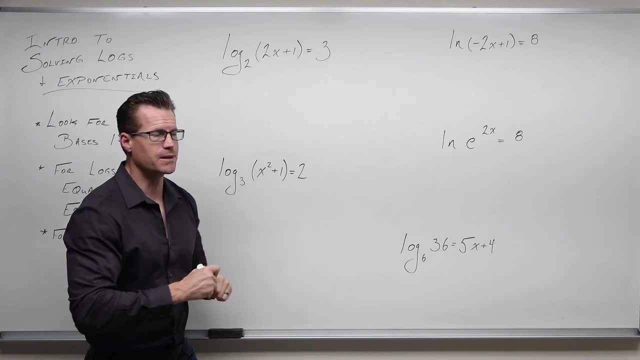 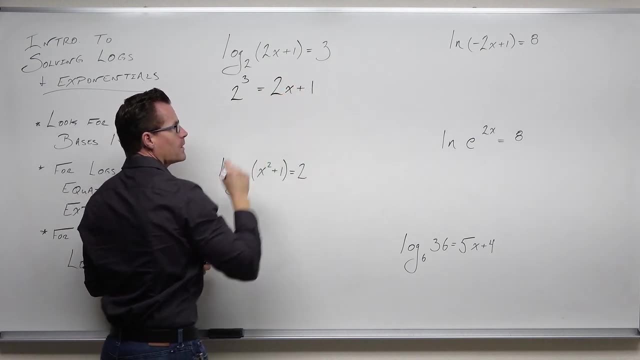 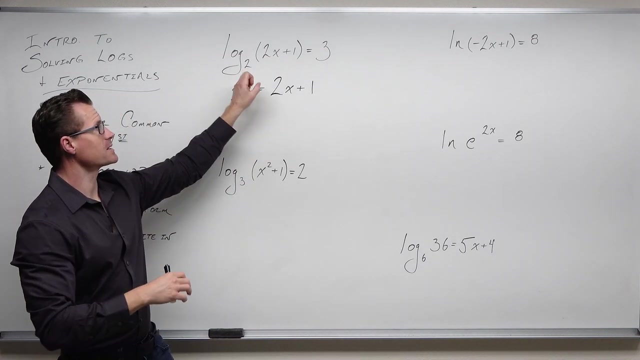 So if our base is two and our exponent is three, our exponential could be written as two to the third, power equals 2x plus one. That, in general, is how exponentials work. They look at a logarithm, they take the base and the exponent. 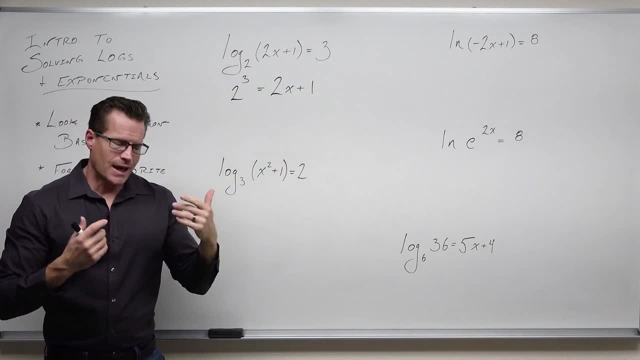 that's a logarithm that's separate of those two things and it puts it back together And notice that this is something that's pretty nice for us to solve. We can take a look at it and go: oh well, now that I have this in exponential form, 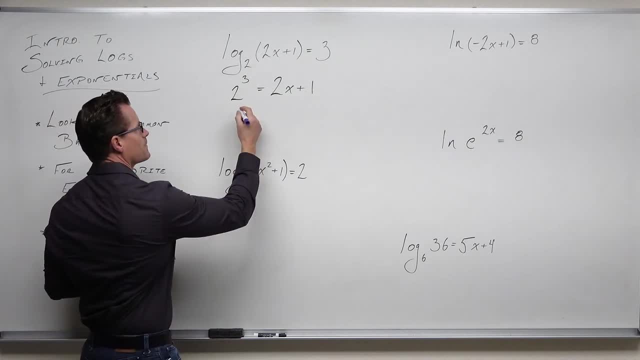 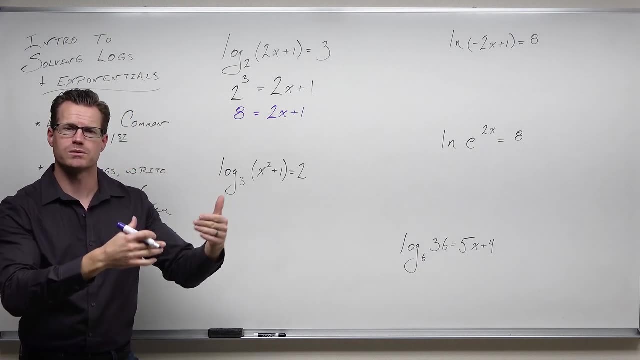 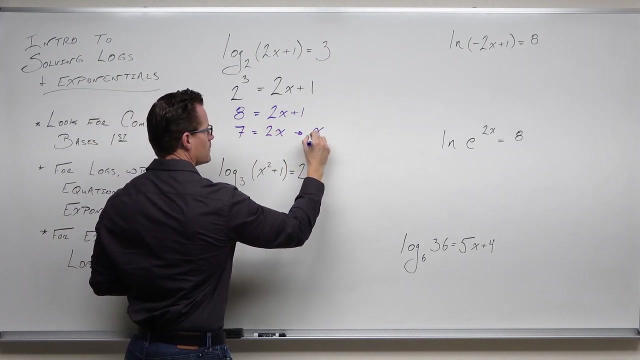 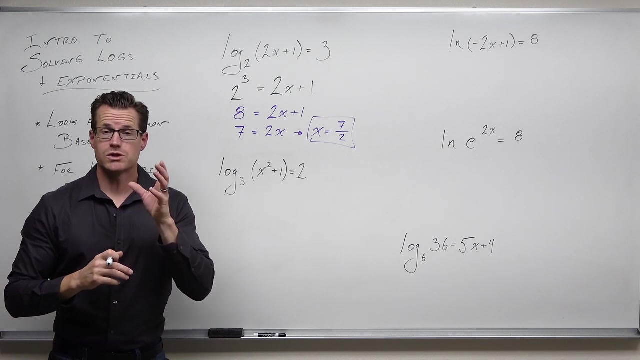 I know what 2x plus one equals two to the third is: 2 minus two is eight. 2x plus one. it's really easy to solve. we can subtract one and then divide by two. So x equals 7 halves, as long as what you solve for does not create a negative inside your argument. and you need to remember that- then our argument: ischooled, Then you're good to go. And if you just go to the cleanser not long after you do this and go to Keeley-しいles, then it's going to work okay. 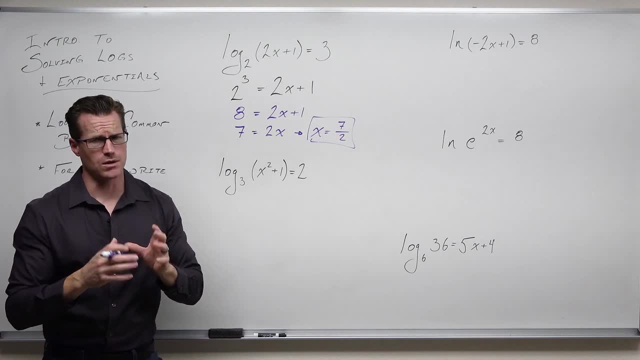 have to be positive. Our domain for logarithms is strictly greater than zero. So if we ever have a solution that causes zero or a negative when you plug it in, that's an invalid solution. Typically it happens when you have a quadratic or higher, but we always would want to check that. 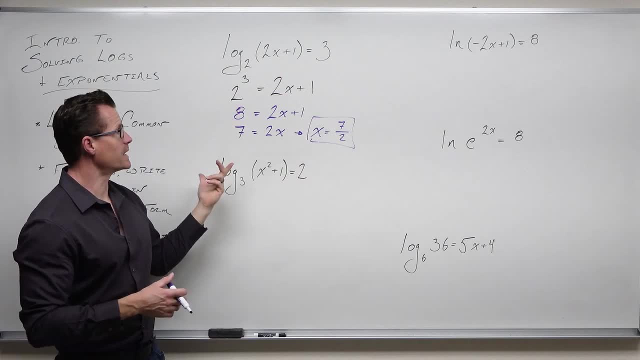 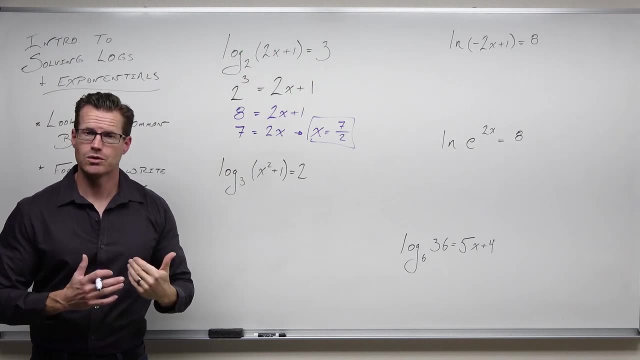 So we check. does that make this negative? No, In fact. you can plug this in Two times: seven halves is seven, Seven plus one is eight, And two to the third power would give you eight. That's exactly true And that's exactly what this is solved for. That's what we're going to do to 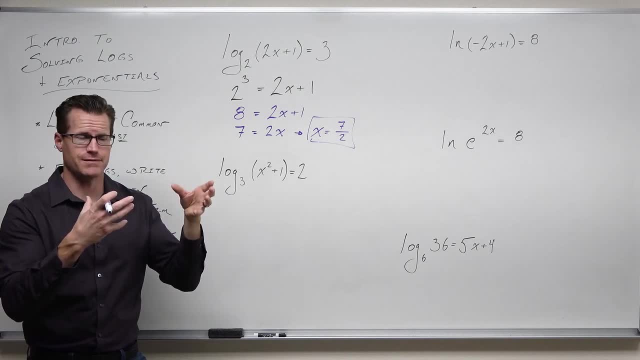 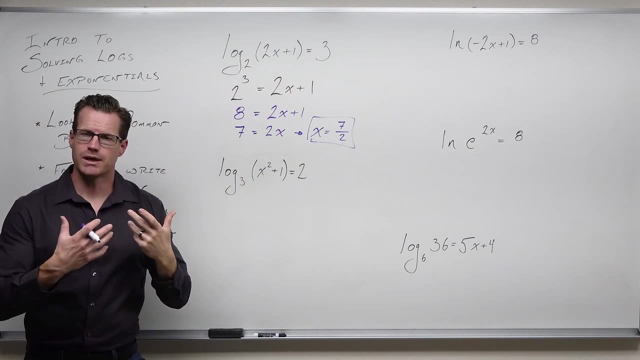 solve logarithms. You check for common basis That takes two logarithms. If you don't have that, you're going to need to isolate your log. We've got that: One log, one side constant And then use an exponential notation to solve that. It's going to be pretty easy to solve in most of these. 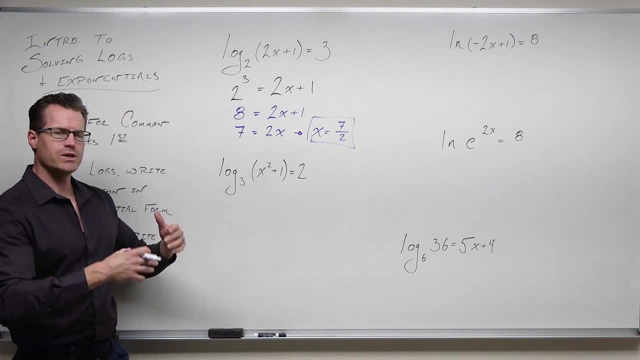 cases. Let's move on to another one. So we have another logarithm. We check for common basis. I don't have two logs, I have one log. There's one log on one side and a constant on the other. Exponential. 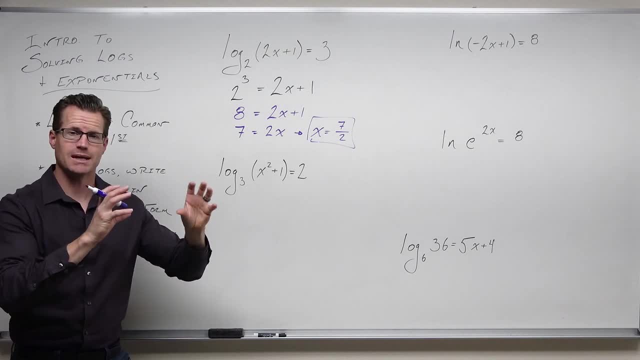 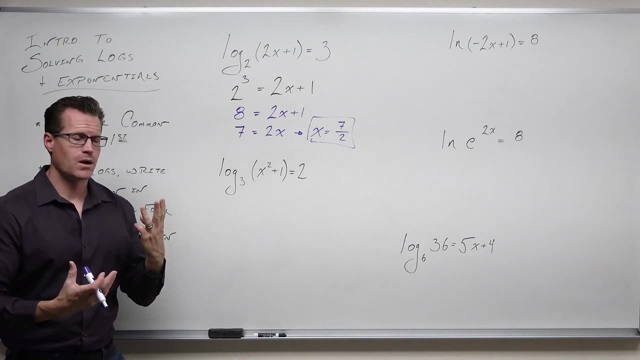 Exponential notation will solve your logarithm. The exponential is an inverse of some logarithm And so we're going to use that inverse Identify your base. So our base here is three. Our exponent is on the other side. A logarithm has stripped away the exponent and separated on different. 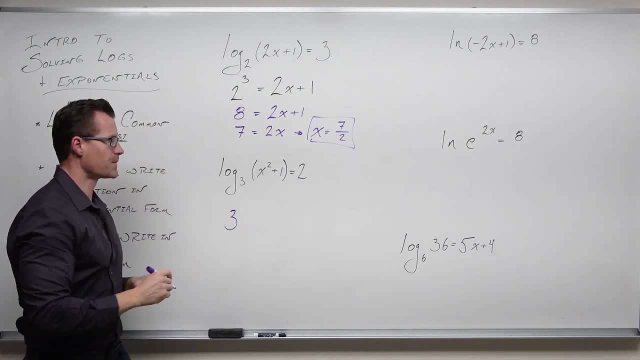 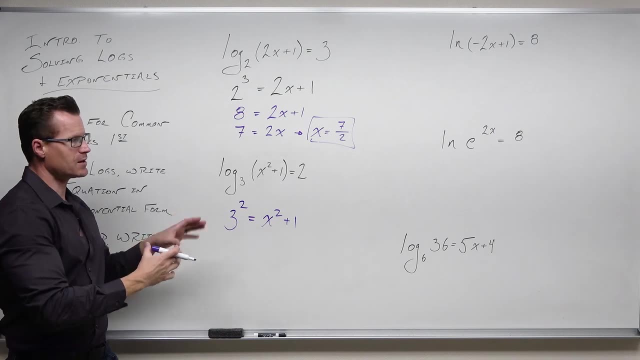 sides of the equation. So our base for an exponential is three, The exponent is two And that's going to equal x squared plus one. This is the exponential notation of the inverse of that particular logarithm, with the same base and the same exponent. 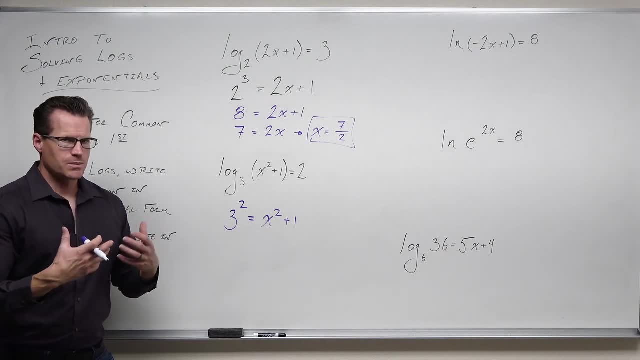 Now, if you're going to solve a logarithm, you're going to have to use a common basis. Now we're going to solve for x, So notice that we do sometimes have to rely on some techniques that we've had. So when you set up your exponential, you might have a quadratic. 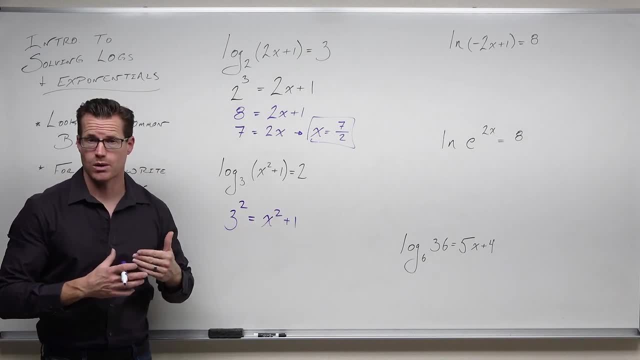 You might have to factor this. In this case we're just going to use the square root method because we can isolate that power too, But you might have to factor it, You might have to do quadratic formula for it, And that'd be lots of things to solve this. Here's the main point. 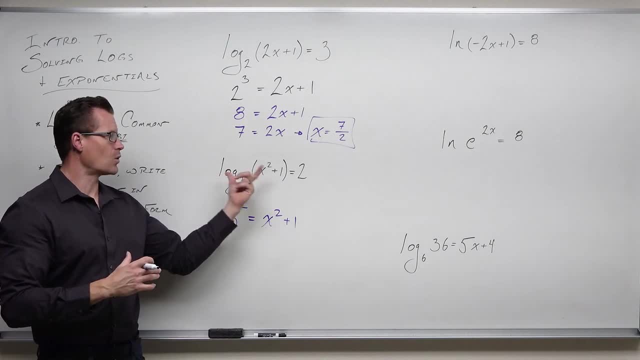 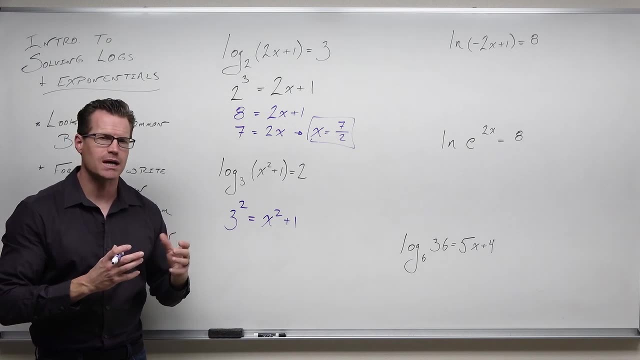 The only thing I'm really trying to teach you in this video is that in order to solve a logarithm, you're going to have to put it in exponential form. Also, this video is very basic. We have some other techniques with exponentials that I'm going to show you later. 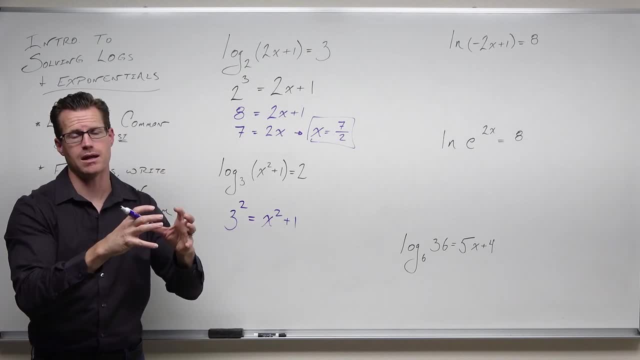 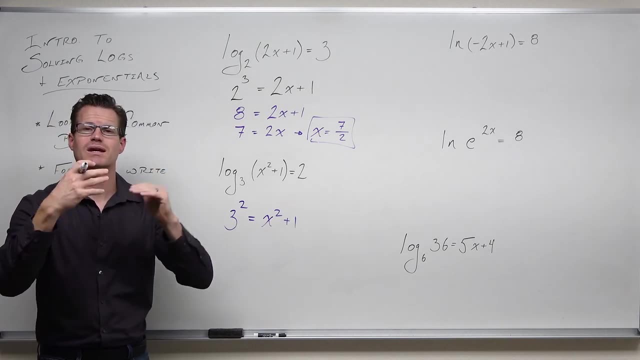 But right now it's just the idea I need to just pound in your head that exponentials are what it takes to solve logarithms. When we get to exponentials, it's going to be: logarithms are what it takes to solve exponentials, because they're inverses of one another. 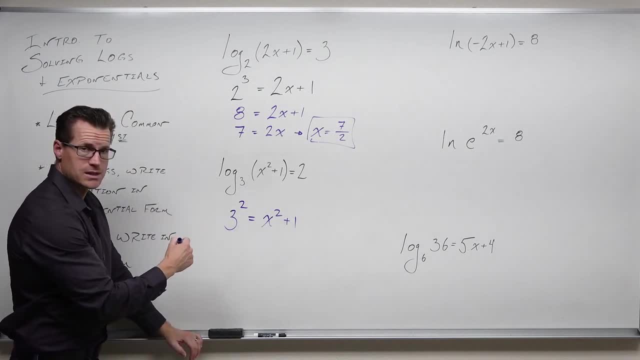 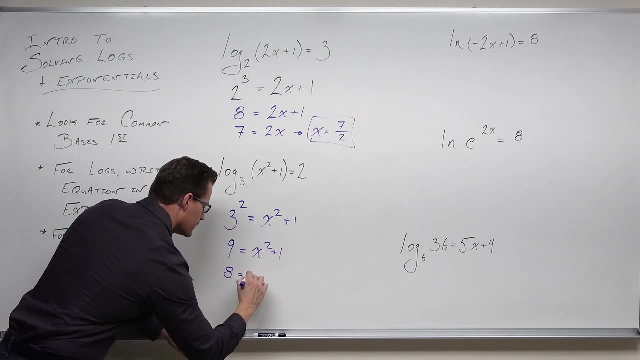 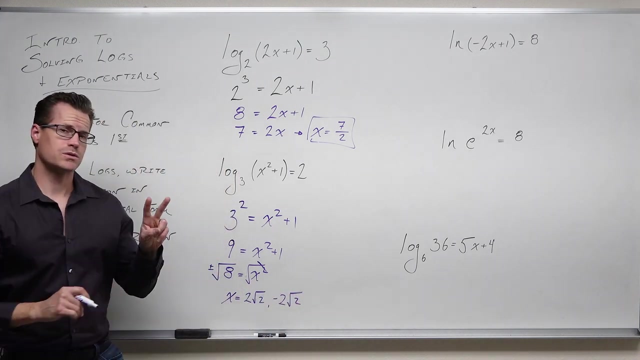 So solving this. we know that three squared is nine. If we subtract one and we take a square root, Remembering that when you take a square root, you need to have a plus and minus, We end up getting two solutions: We get plus and minus the square root of eight. 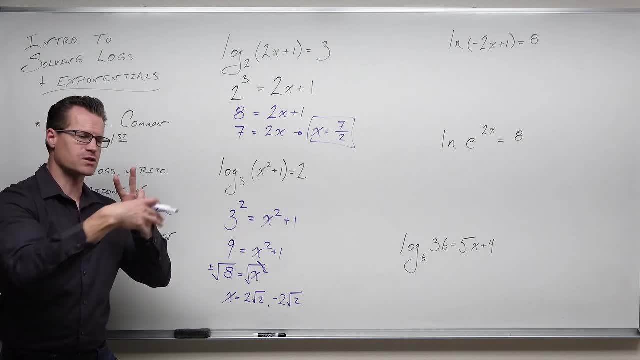 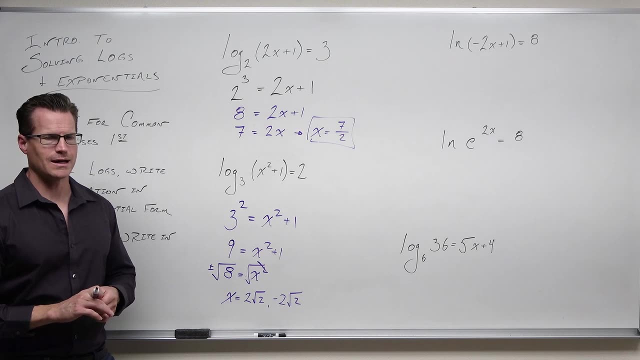 Because eight is four times two, the square root of four is two and it leaves us a square root of two. That's two root two and negative two root two. Now the common question is: wait a minute, I thought you couldn't plug in negatives into a. 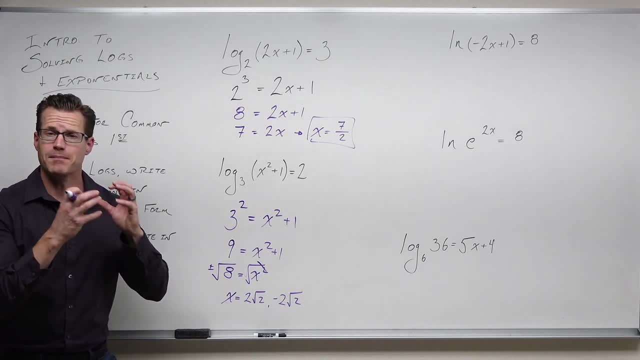 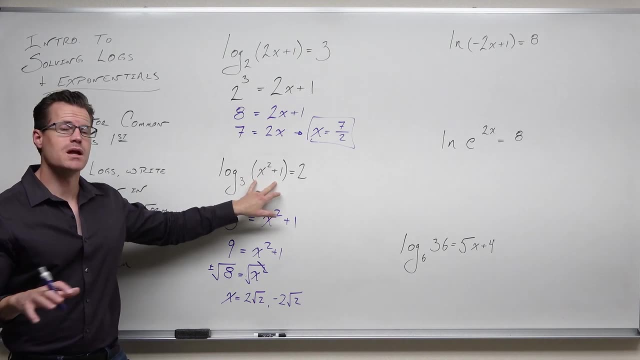 logarithm. Well, you can't plug in values that make the inside of your logarithm negative. But look at our argument here. Look at this: x squared plus one. There's nothing that you can plug in here that's going to cause that to be negative. 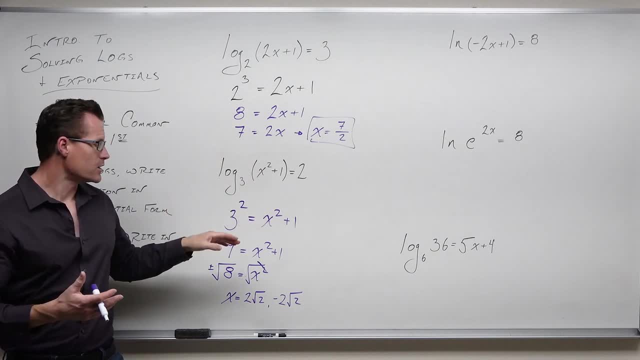 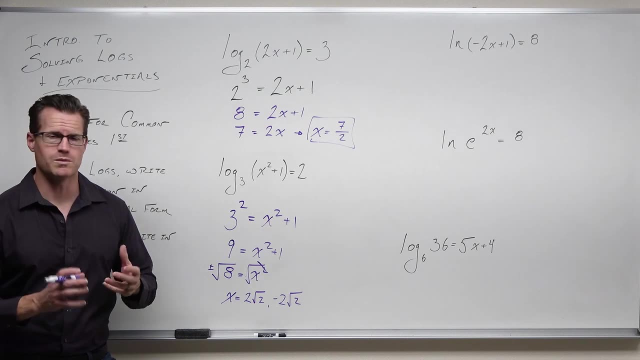 You can plug in positive numbers. Something squared plus one is going to be positive. You can plug in negative numbers: Something negative squared plus one is going to be positive. So you have two valid solutions for you, because they don't make the inside of your logarithm negative. 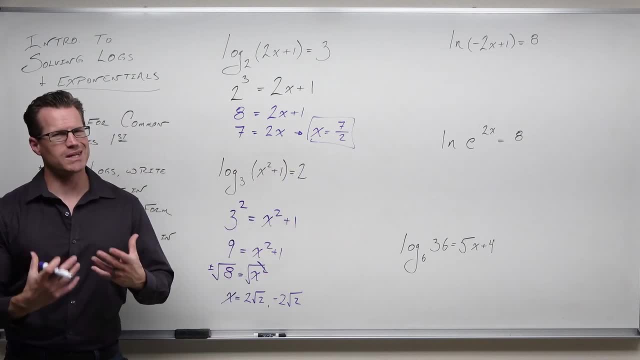 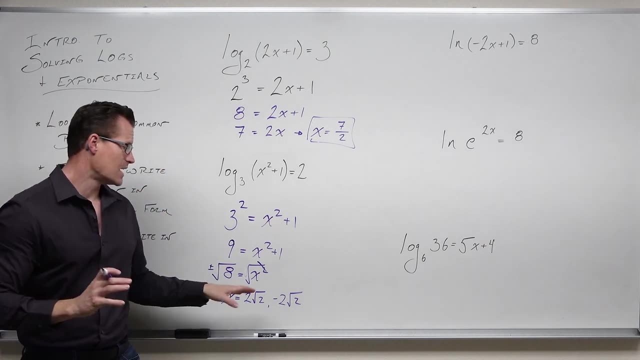 It's very common for students to look at this and go, oh, I can't have negatives. It's really easy to do that, But that's not the idea. The idea is you can't plug in values that make the inside of that logarithm negative. 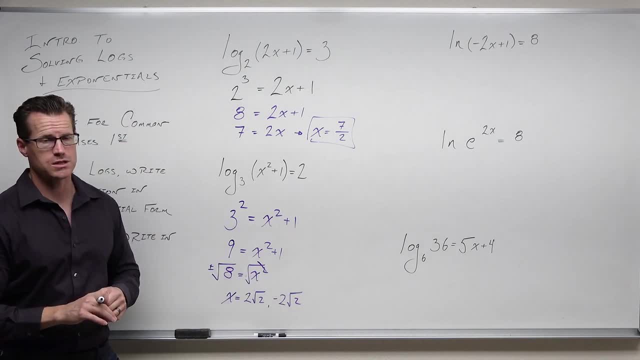 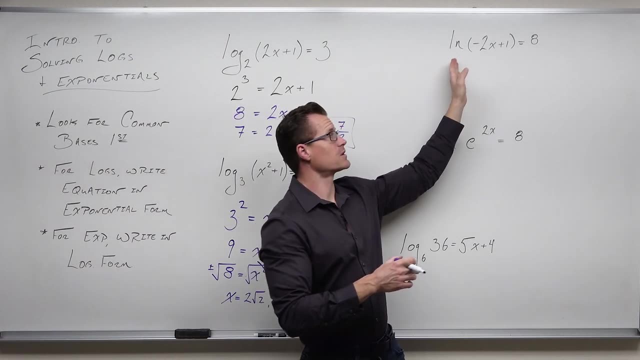 Neither of these actually do that. Therefore, they're both valid solutions. OK, moving on, Do you remember that if I have a logarithm and I've checked for both sides, both sorry, I've checked for common bases, I don't have mine. 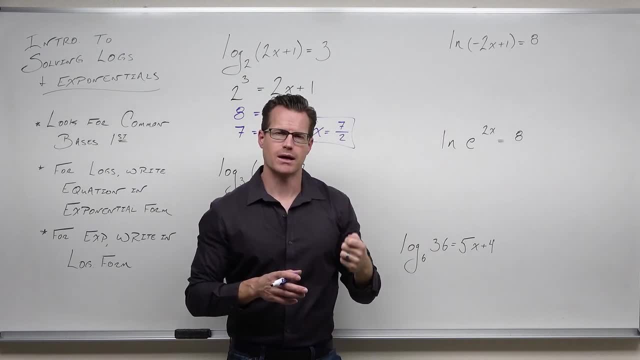 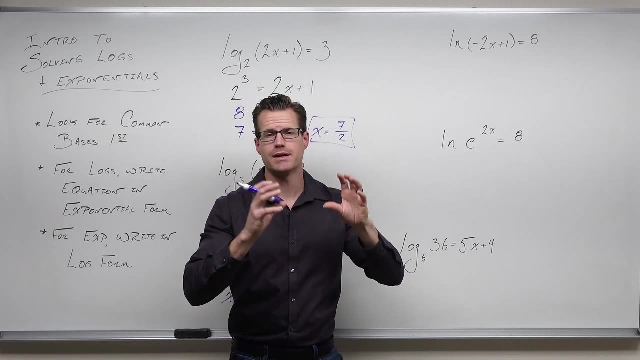 I just have one logarithm And it's isolated. Do you remember that when you have an ln it stands for a logarithm but it has a certain base, So that base would be E. ln stands for the logarithm of the natural number. 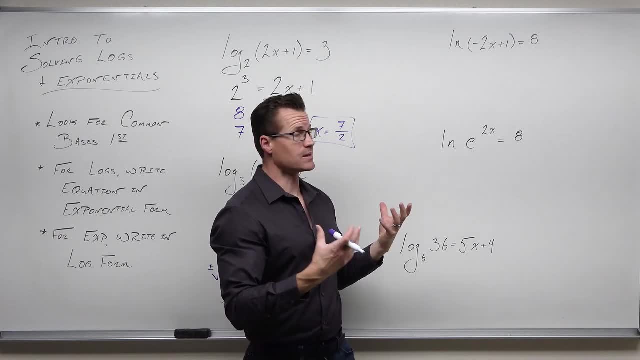 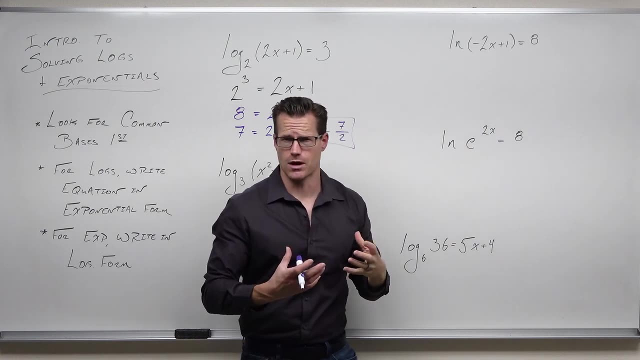 So that says it's an implied base of E here. So this is a logarithmic equation. I check for common bases, but I only have one logarithm, I don't have two. That's what you would need for common bases to work. 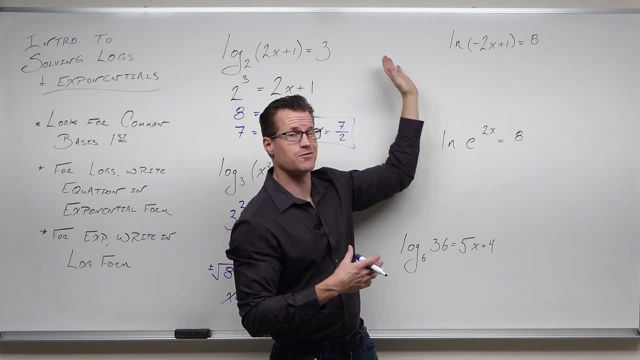 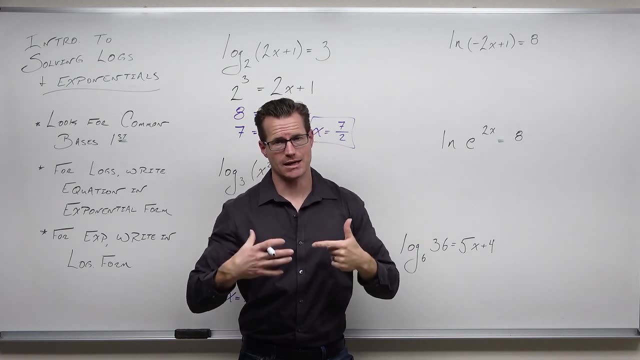 I have my logarithm isolated. There's nothing being added, subtracted or multiplied. It's very basic here What we do when we see this. So we go: OK, We've got a logarithm without common bases. You're going to need to get an exponential from that. 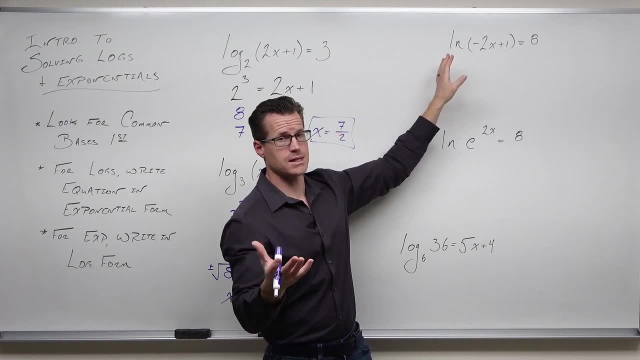 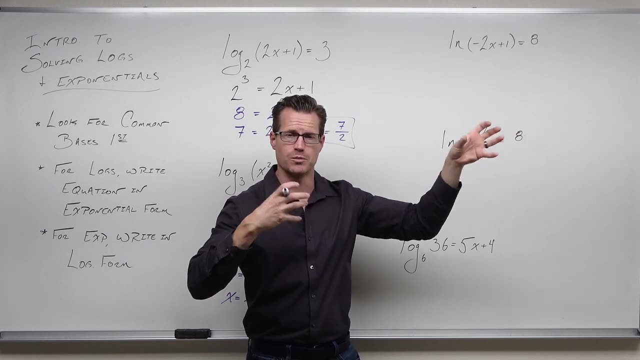 So when we look at it, we are right. Our base is E, Our exponent is 8.. Remember a logarithm? all of them has separated the base from the exponent. Put them on different sides of your equation. So we're going to put it back together in something called exponential notation. 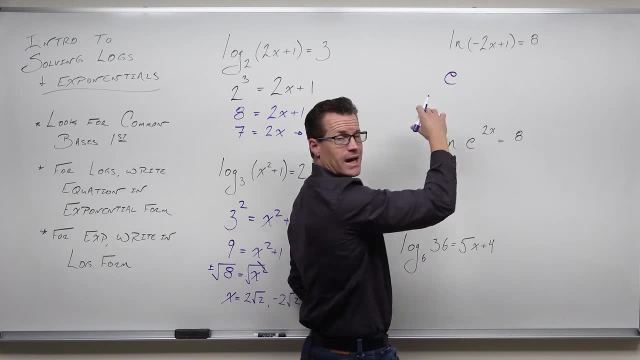 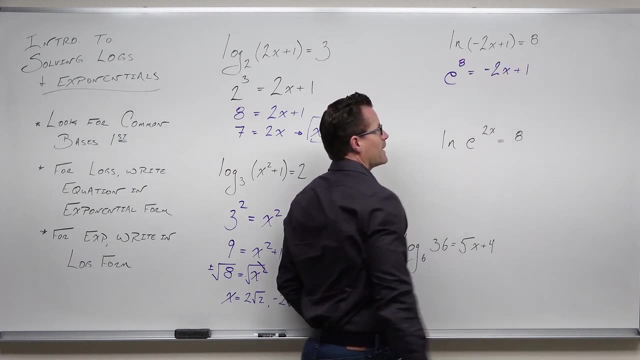 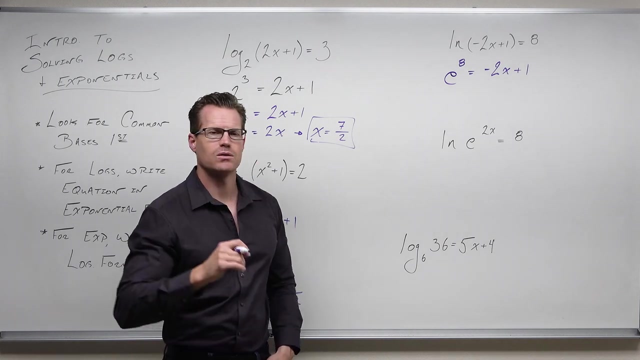 So our base is E, Our exponent is 8. And that's going to equal the argument negative 2x plus 1.. It looks a little weird, but we can certainly solve this. If we solve for x, go through the same exact steps that you would with any other equation. 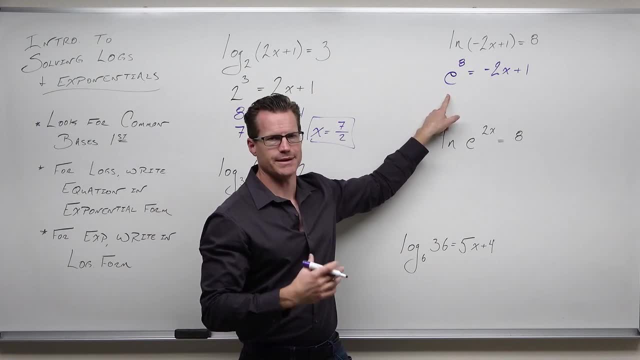 If that's our variable. remember that's a number, That's like 2.7-ish. It goes forever. It's a transcendental, You can't really get to the end of it, but it is a number. It's sort of like pi. 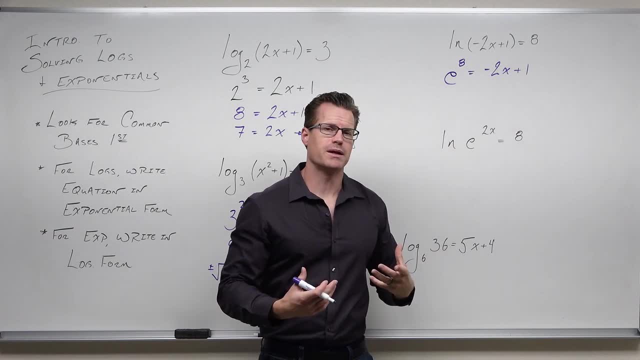 If we're solving for x, you're just going to subtract 1, and then we're going to divide by negative 2.. Do exactly the same thing here, but don't approximate either. But don't approximate either, So we're going to divide by negative 2.. 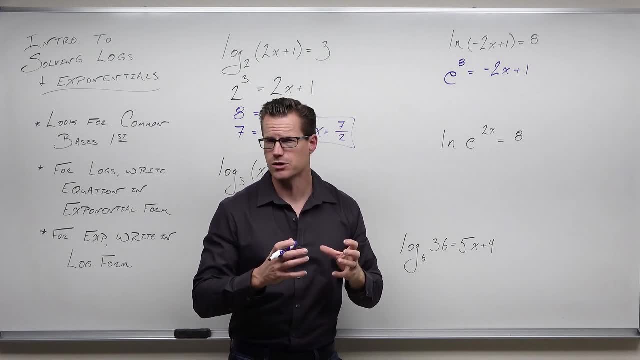 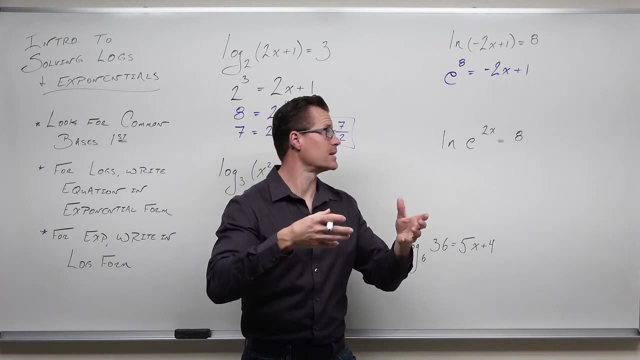 We're going to subtract e to the 8th. What we want is something called an exact solution. So an exact solution hasn't used your calculator to say, well, e's about this. therefore, e to the 8th is about this. and then we subtract 1, it's about this- divide by negative 2,. 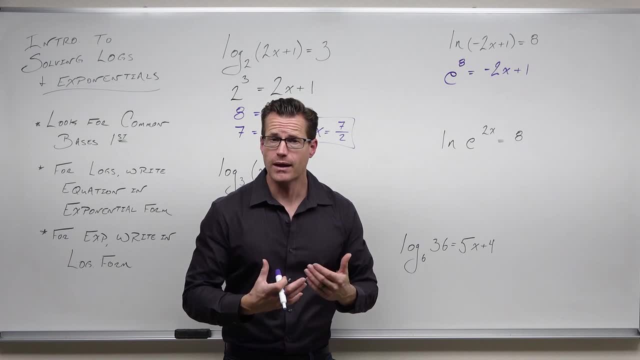 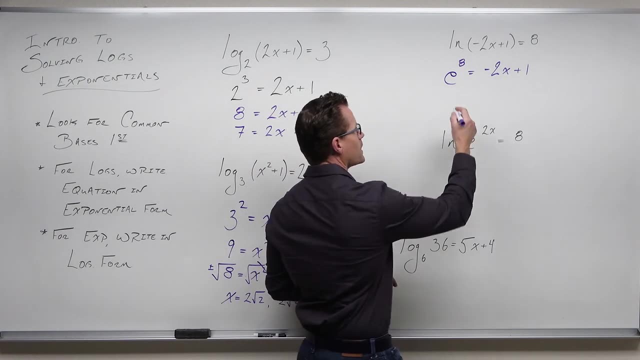 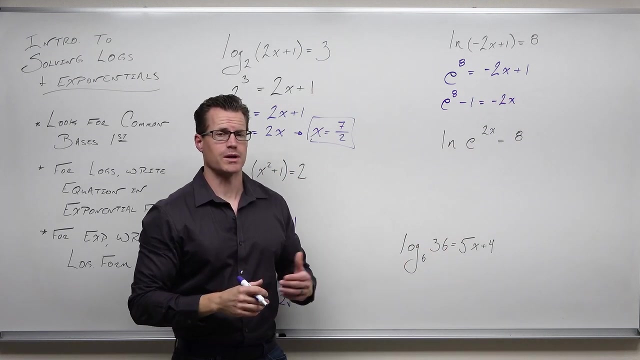 it's about this. That's an approximation And those are valid sometimes when they ask you for it. But if you need an exact solution, this is the process you go through. Subtract 1 from both sides. Notice it's not subtracting from the exponent, it's subtracting from e to the 8th. 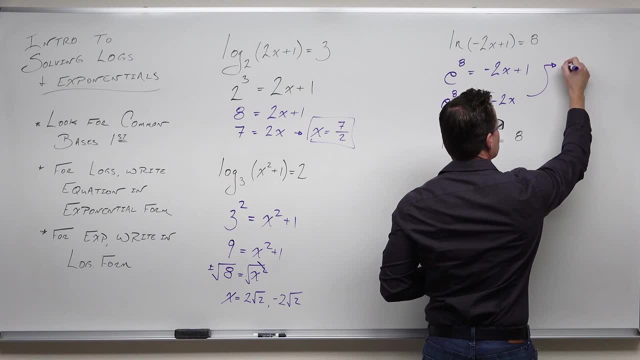 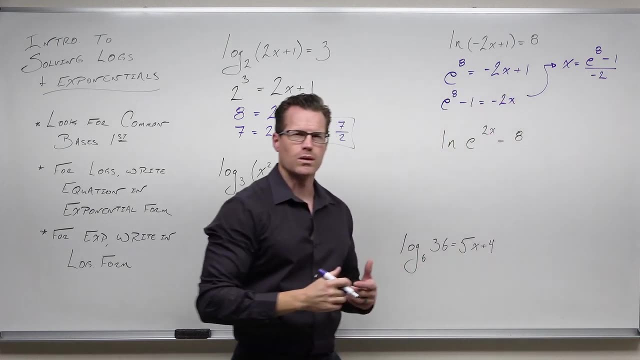 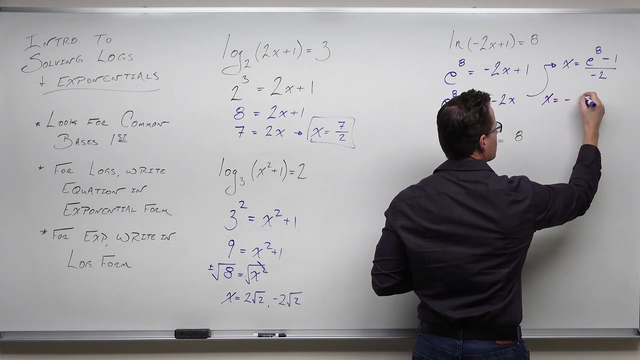 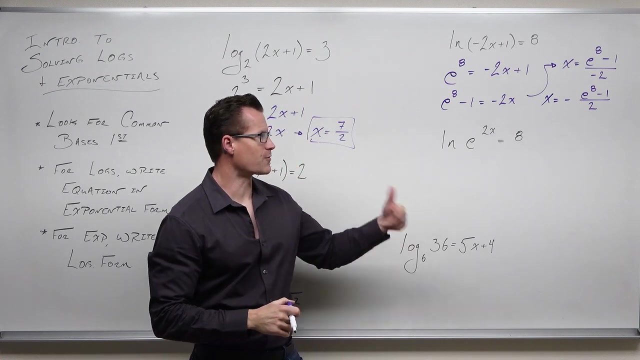 And then we would divide by negative 2. And we typically don't like to see negatives on the denominator, so we can move that out front. that's appropriate. We don't like to see them on the denominator. move them out front. Or you can run it through the numerator as well. 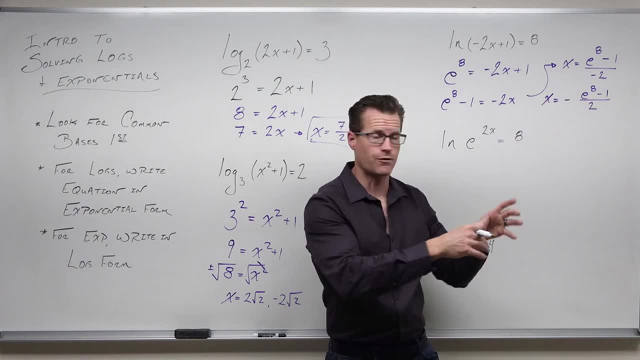 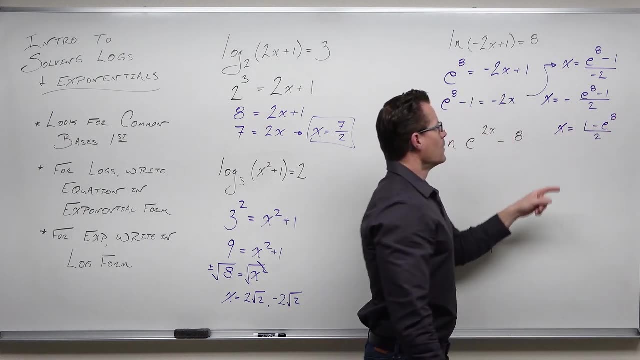 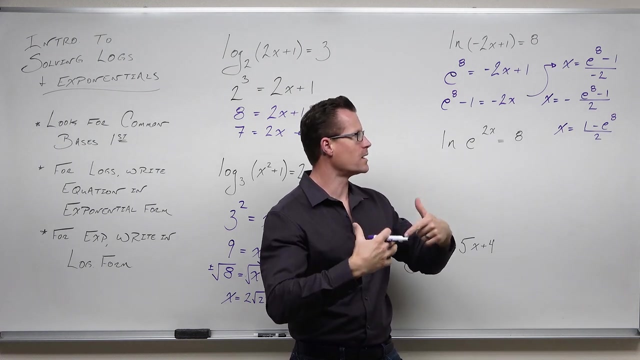 So negative e to the 8th and then plus 1, or we can reverse that. One of these two solutions is really what you should end with, Something with a negative e to the 8th minus 1 over 2, or 1 minus e to the 8th, just distributing. 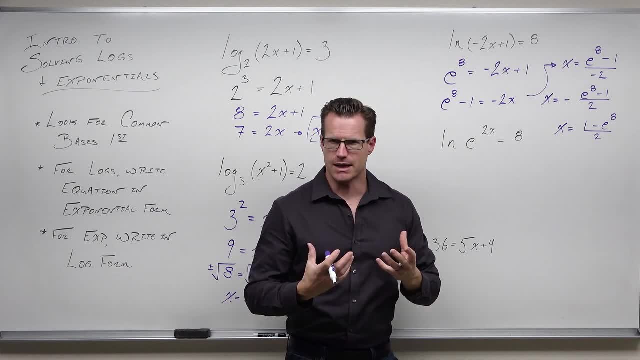 that negative through your numerator over 2.. This is what's called an exact solution. We have not approximated. Now, if you want to approximate, what you can do on your calculator is put perimeters. You can put them on your calculator. 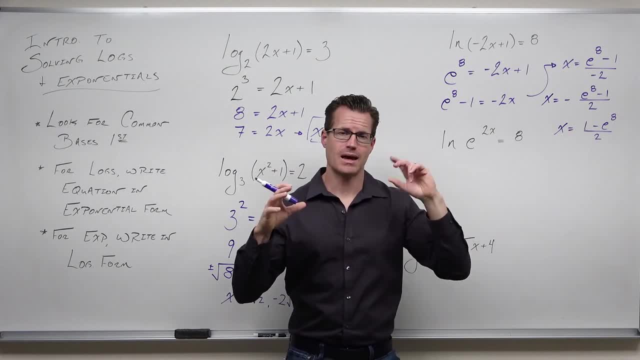 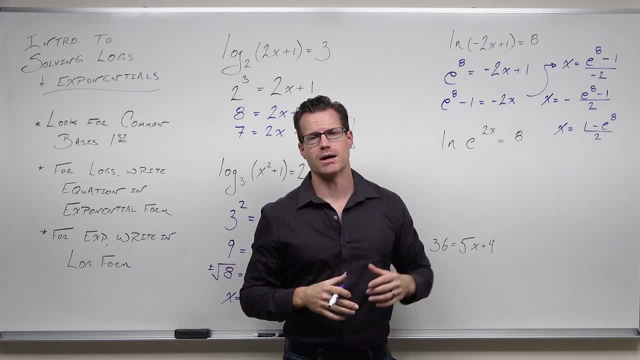 minus 1 minus 1 minus 1 minus 0, that's minus 0. So that would be in parentheses. Plug in 1 minus e to the 8th. End that parentheses, Because you need to tell the calculator that that's my numerator. 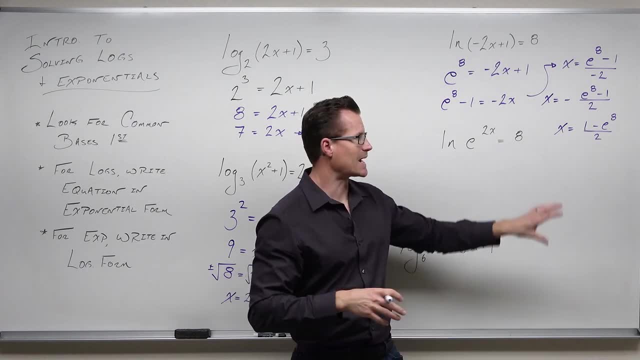 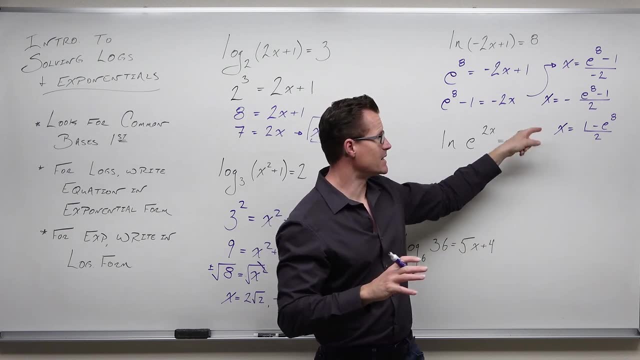 And then divide by 2. It will give you a decimal approximation, And that's sometimes useful for us. but if you're asked for exact, that's what we do. Also, when we are doing math and we need an approximation, don't approximate until you. 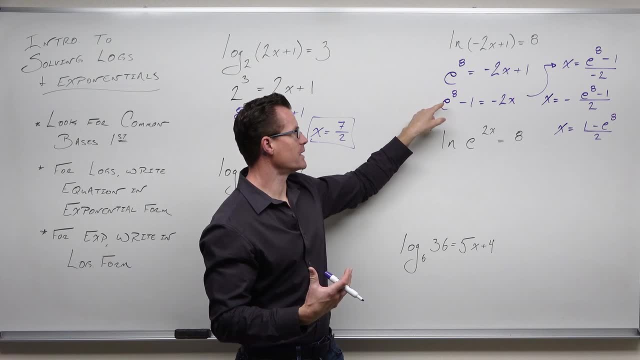 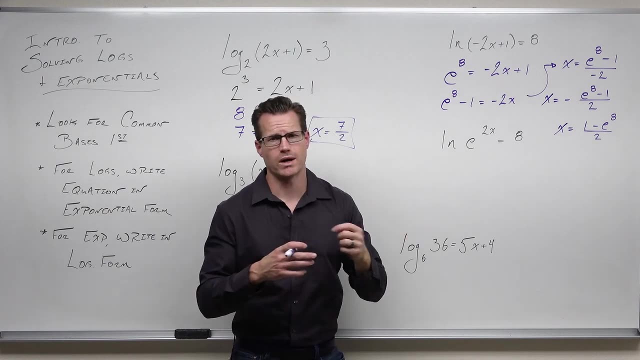 get here. So what I don't want to see. I don't want to see plugging in 2.7 or e and then getting eighth and writing down a decimal and then subtracting one and writing down a decimal, then dividing by negative two and writing down a decimal. You're starting to round your. 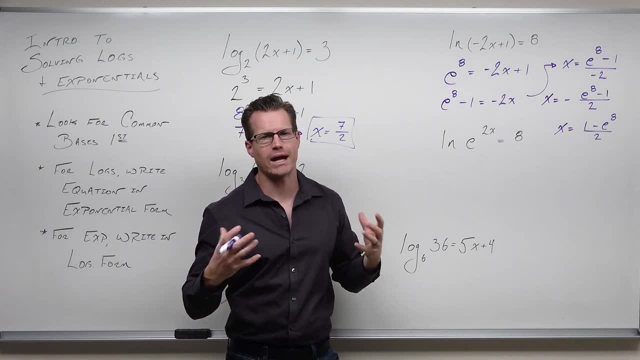 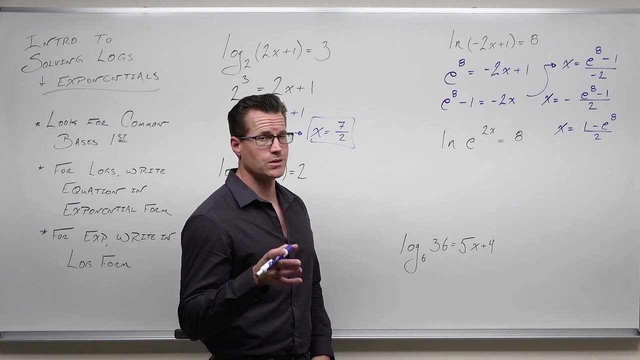 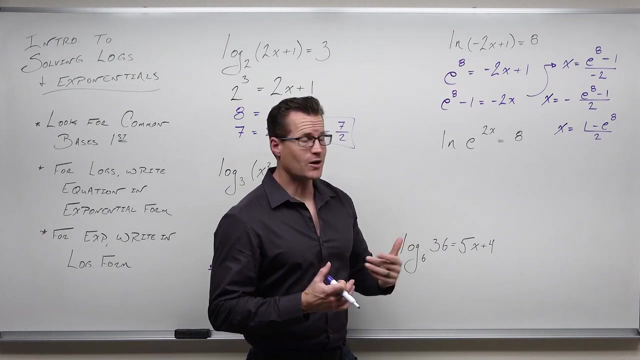 approximations, and if we approximate approximations they get more and more error in them. It's not really appropriate to do so. don't do that. Now, it seems kind of awkward to check, but you still could check this answer If you plug this in, and you plugged it in right there. well, it's really. 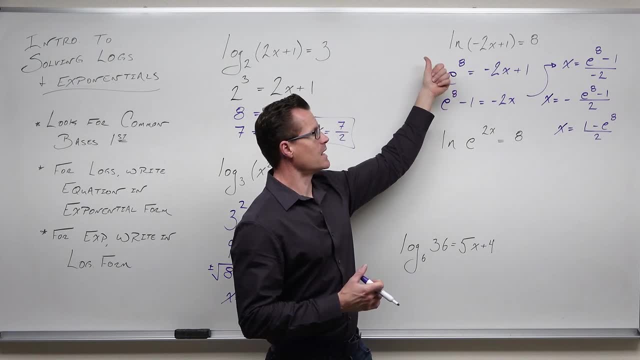 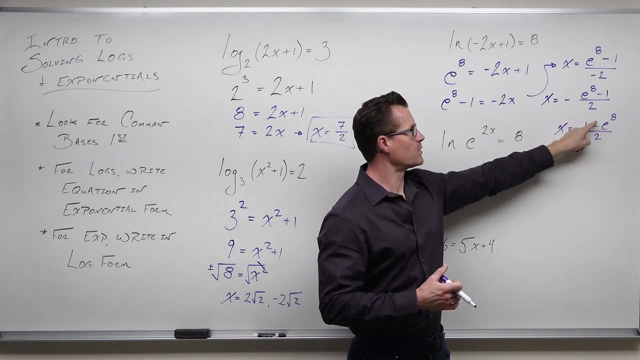 weird. but think about how this would take the place of x, Negative two times something over two. those twos would cancel That negative, would distribute here and give you negative one plus e to the eighth. Negative one plus one would give you zero. You would end with e to the eighth. 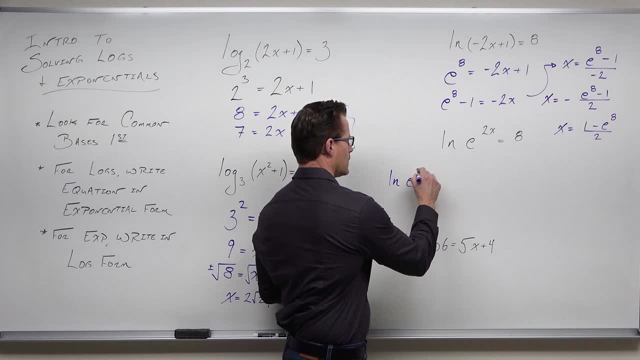 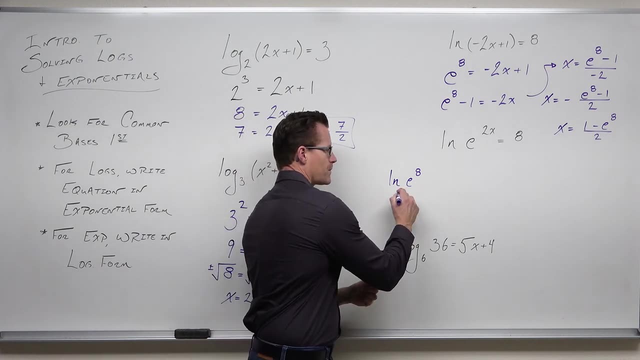 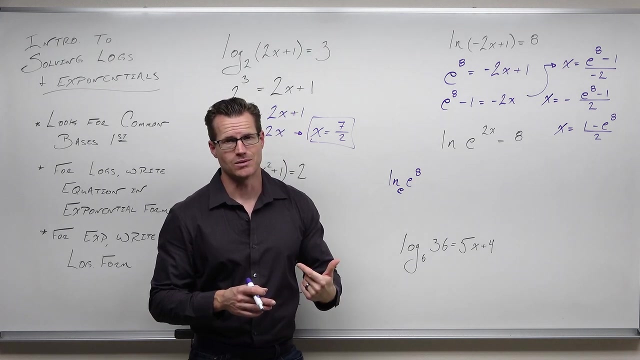 Now wait a minute. ln of e to the eighth. We're going to see this right here. but whenever you have an exponential composed on a logarithm or a logarithm composed on an exponential, we're going to see them. Proposal logarithm is a very nice video. These things cancel This right here. says this is going. 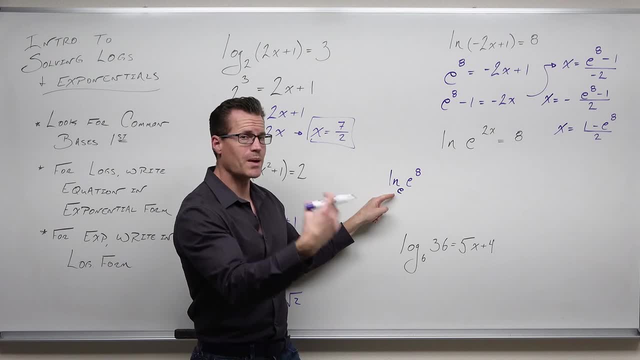 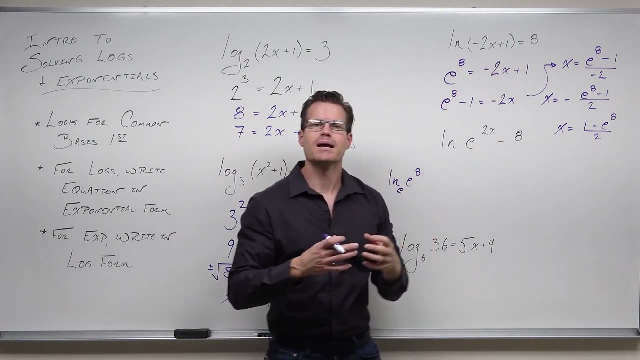 to give you eight. So in other words, it says: e raised to what power gives you e to the eighth? Well, e to the eighth power would give you e to the eighth. Oh, hey look, it's eight. It makes. 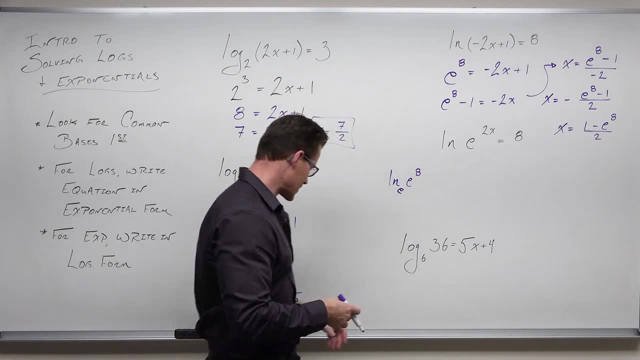 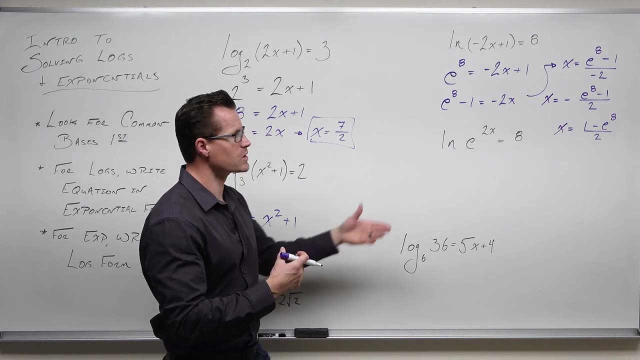 sense It actually works, So that we can check- and it becomes a little more awkward- What you can't do. you can't check an approximation. It's not going to work out because you just approximated the decimal, which is another reason why we want to leave it in exact answer form. 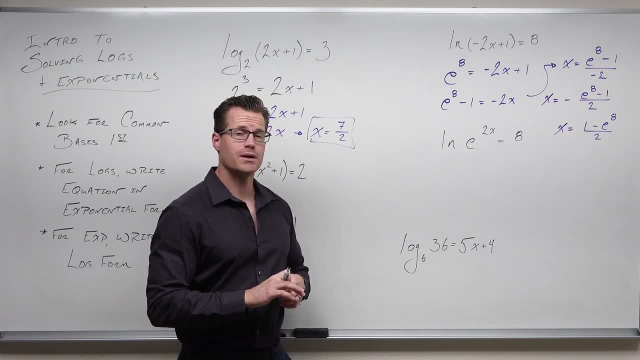 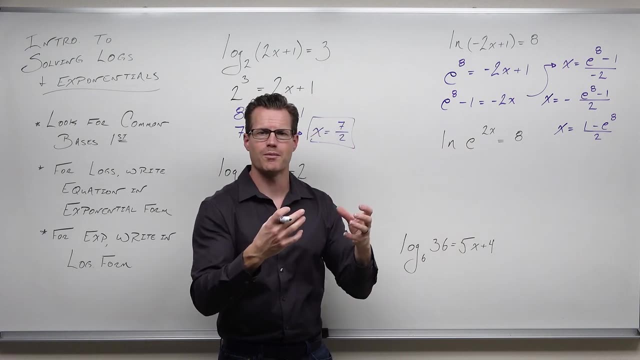 So, moving on here, a couple of special cases where you don't necessarily need to write an exponential, but you still can. So I want to show you this. So we check. Do I have two logarithms where I can make common bases? No, not really. What am I going to need? Oh, I'm going to need. 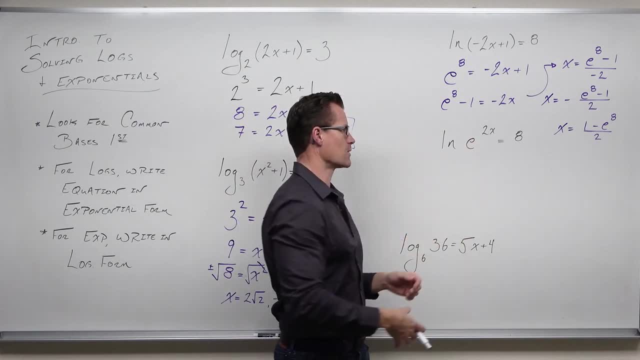 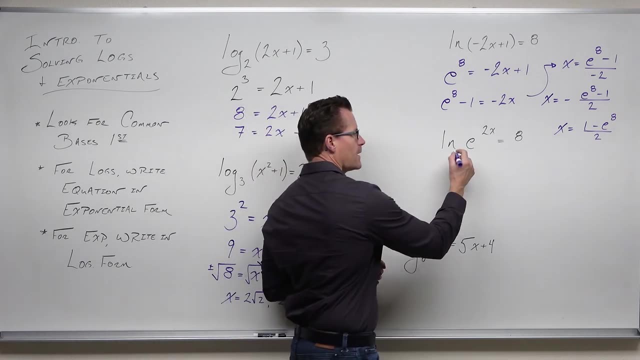 an exponential, but I'm going to need a logarithm isolated. We have that right here. The base of this particular logarithm is e. So notice what happened. It's just what we talked about. If this has a base of e, which we never really write, here's what is actually going to happen once we. 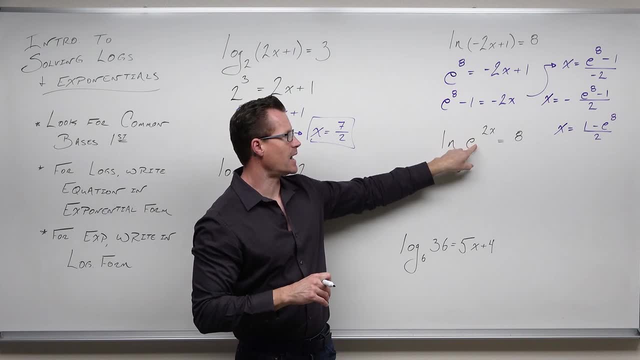 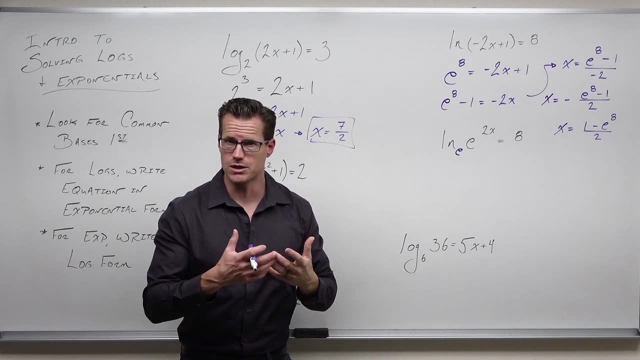 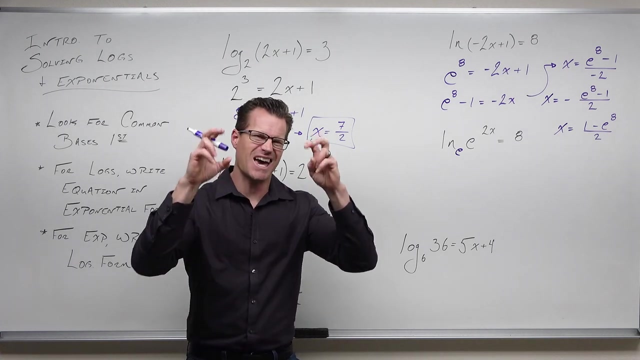 learn about the properties of logarithms. You have now composed an exponential onto a logarithm. You've composed two inverses. The reason why we talked about compositions and inverses is so that you would learn that when I compose two inverses, they cancel and you get x- The x here in this. 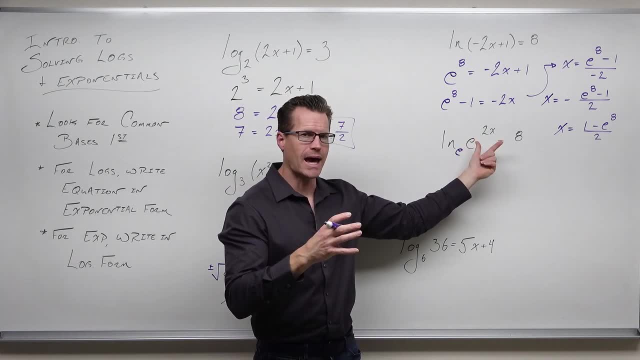 case is 2x. It's your exponent. So what's going to happen? I'm going to show you this. I'll prove this to you with the exponential notation. What's going to happen? You're going to end up going. 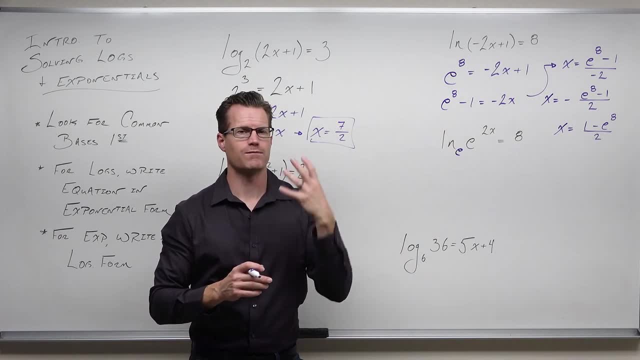 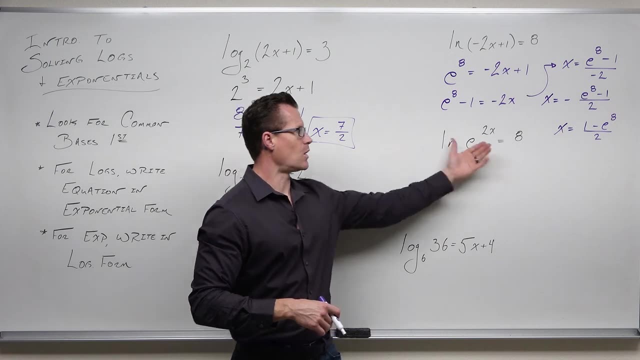 ah, that's going to be: 2x equals 8.. Your solution is going to be 4.. Now can we see it a different way? Sure, If you understand that that base is e and that this is a logarithm, it's isolated. 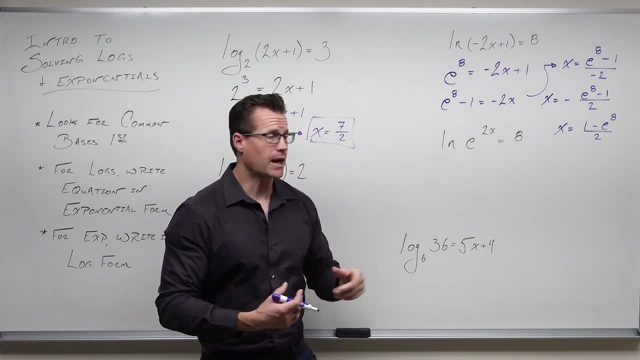 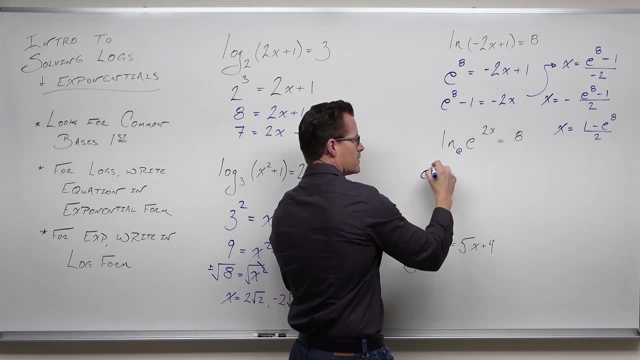 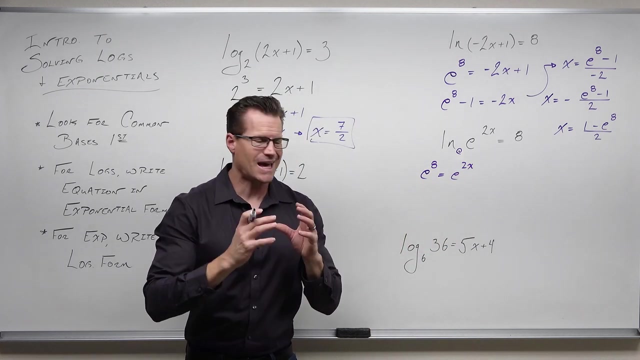 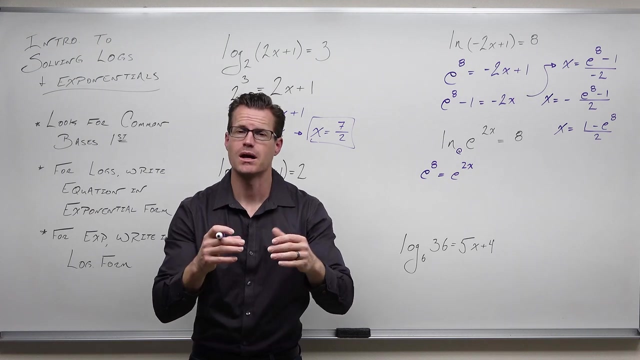 can you write it in exponential form? Well, yeah, we can. Our base is e, Our exponent is 8.. So base to the exponent equals our argument. This is what happens every time you compose an exponential onto a logarithm with the same base- This is the key: the same base. What would happen is that: 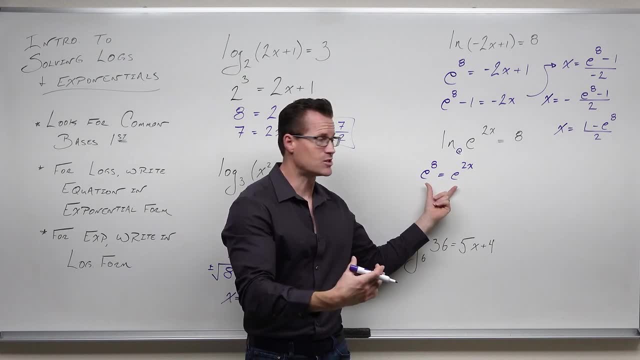 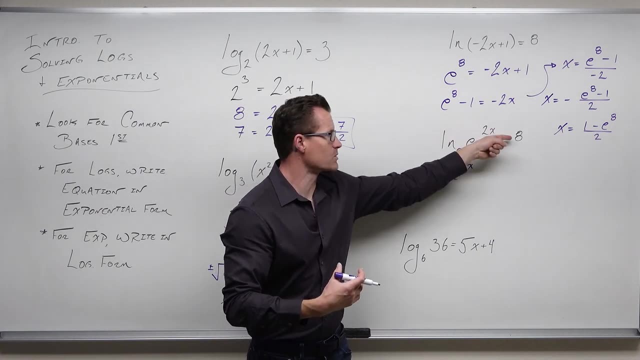 your exponential that you create will have the same base. You can see it right here: Same base means same base. That's why it's so trivial. That's why it says: well, yeah, you can just go, 2x equals 8, because those things cancel out, because these e's practically cancel out. 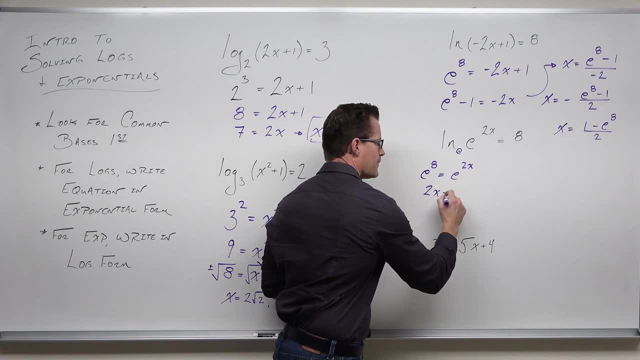 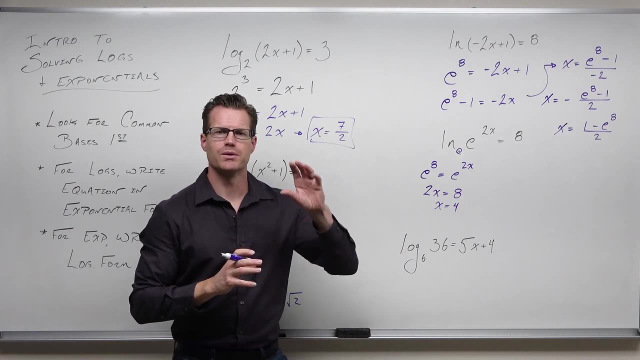 If my bases are the same, then my exponents have to be equal and, sure enough, I get just 4.. That's going to happen. You compose an exponential with a logarithm. If the bases match, then the bases will cancel. 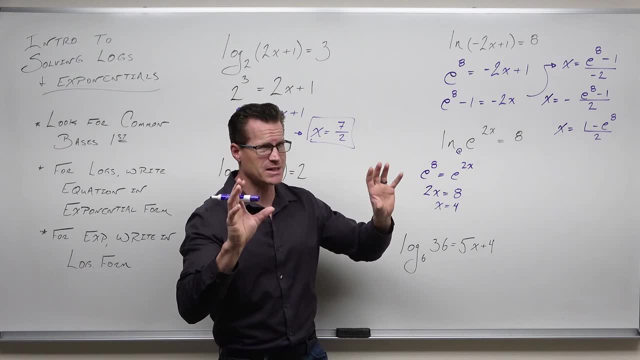 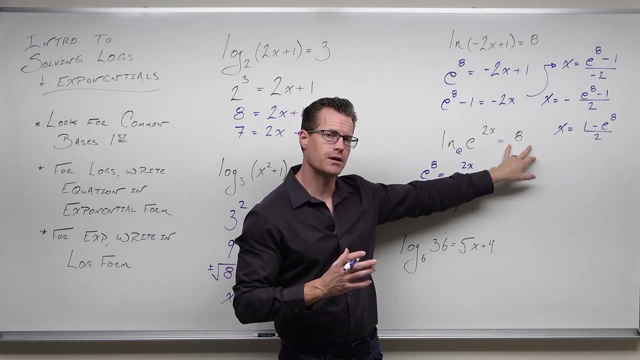 and you're going to get the exponents equal, and that's exactly what we have. Keep this in mind. This is a big deal. This is an exponent, right, But this is also some exponent of an exponential. That's what logarithms have done. They separated the base from the exponent. Our exponents will. 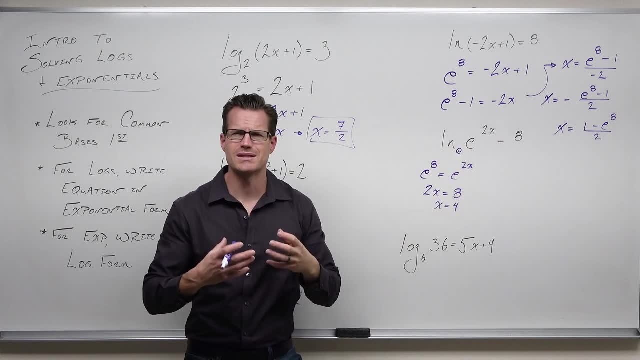 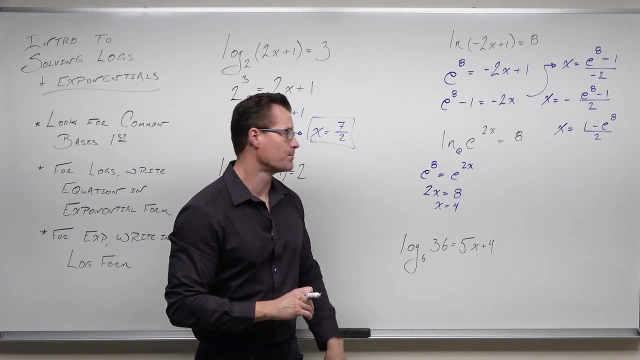 get set equal if our bases are the same. That's the reason why these inverses undo each other. It's because of that They have the same base. They're going to undo each other- Kind of cool, All right. last one's also a special case. I'm going to show this to you. You'll hopefully. 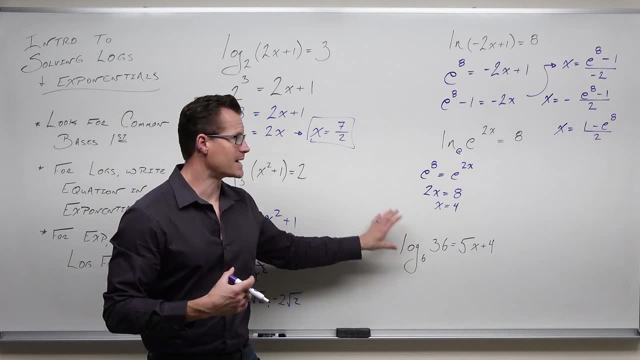 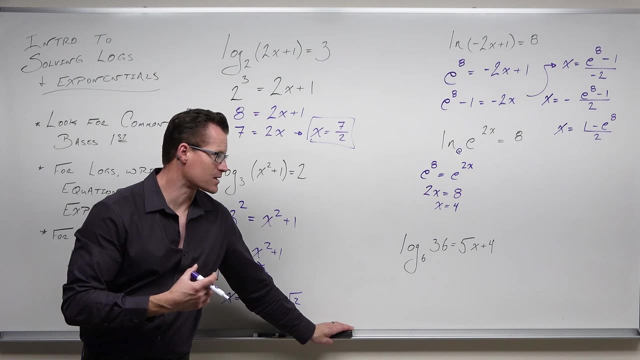 understand the same concept that you're seeing here, with just a slightly different base, and then I'll show you the exponential notation. So if you were to think of log base, 6 of 36 equals 5x plus 4, you're noticing right away that your variables are here. Wait a minute. 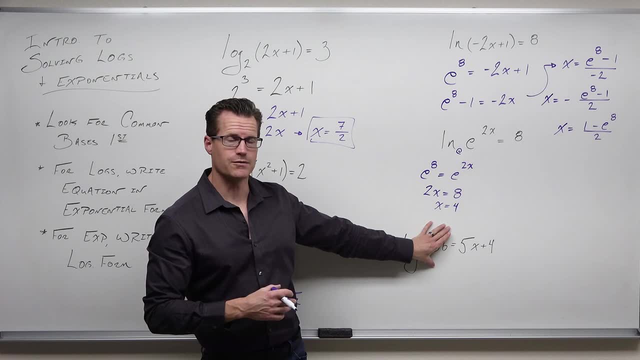 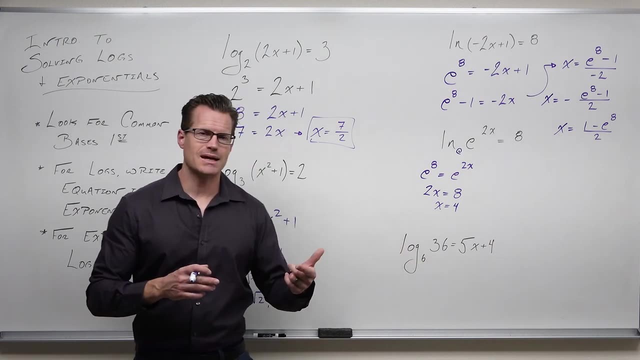 Couldn't you just subtract 4 and divide by 5?? Yeah, you could. There's no variable over here, which means this is already a constant. In fact, it's a constant that we can simplify. Think about this: 6 raised to 2.. What power. 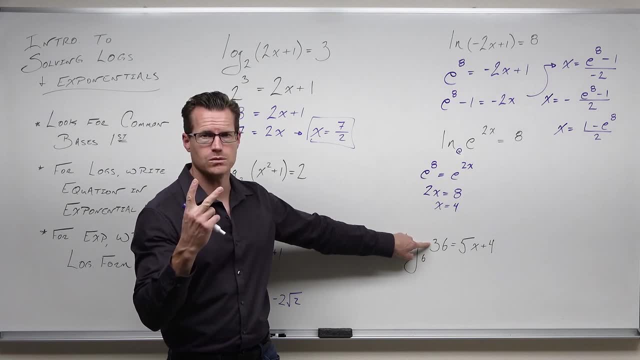 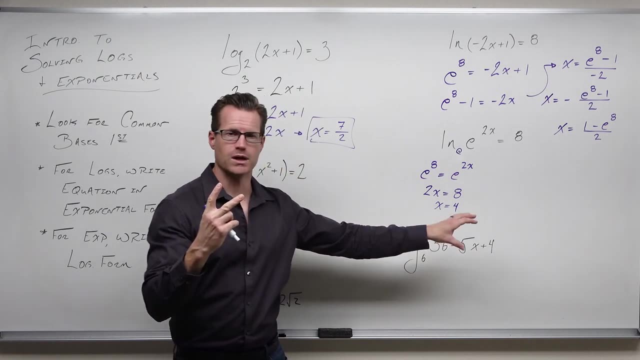 will give you 36? 2. This stands for 2.. I promise you, no matter what you do, you're going to end with 5x plus 4 equals 2.. A couple ways you can see that. Well, what if we thought about it? 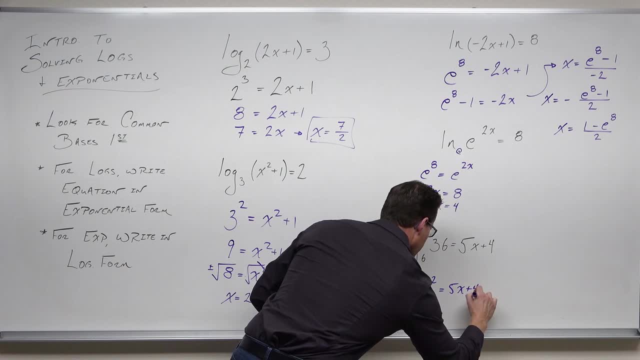 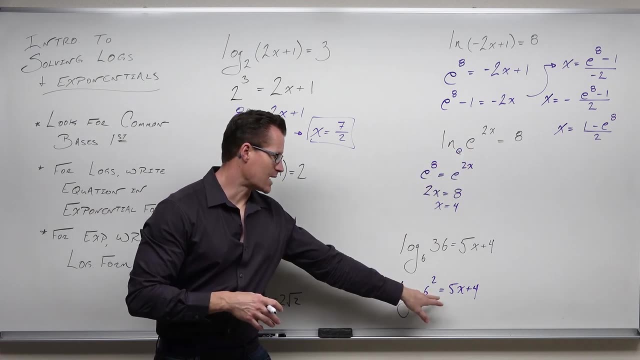 As log base: 6 of 6 squared. 6 squared is still 36.. Oh, but what I've done is the same thing I've done here. I've written this as an exponential and a logarithm with the same base. Well, 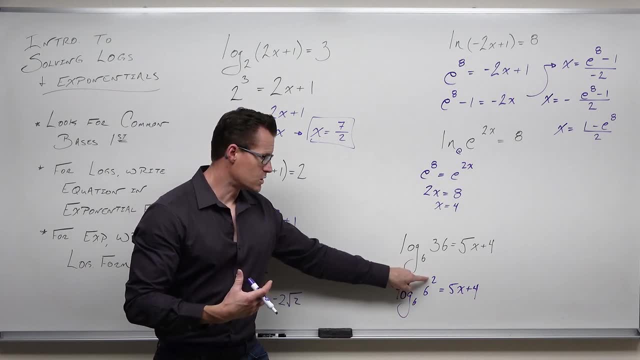 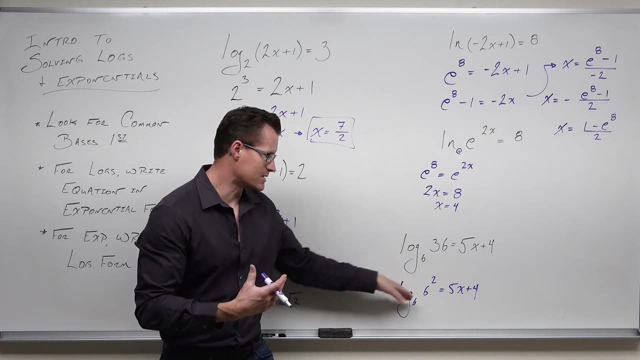 what's going to happen with that? The bases will cancel. You will end up getting 2 equals 5x plus 4.. That's possible to do and we can show it. just this way We can say: hey, that's going to cancel. 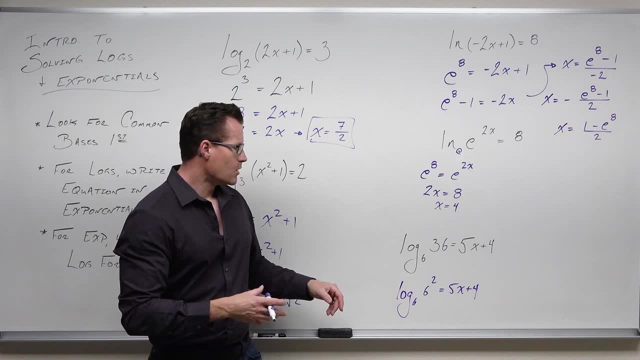 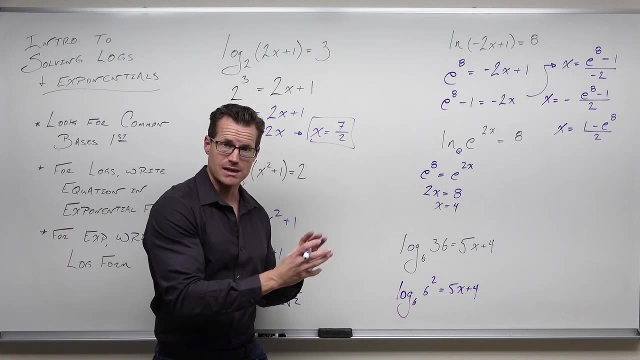 You get 2 equals 5x plus 4.. Or if you need the exponential, we can think of this as if this is a logarithm. it's isolated, It has a base of 6.. I know that if I were to write this, 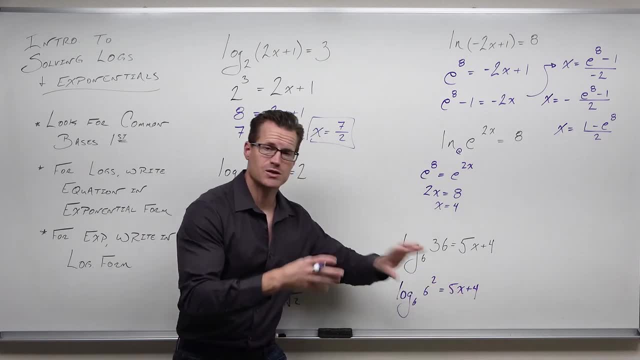 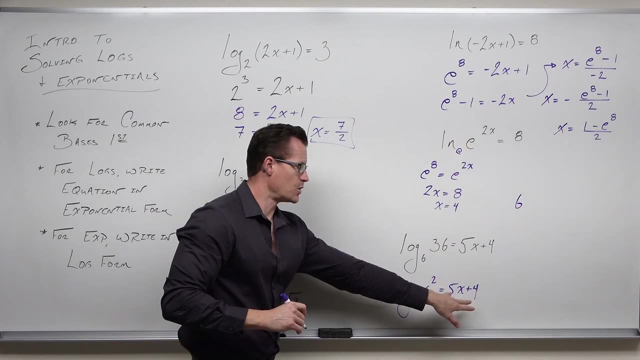 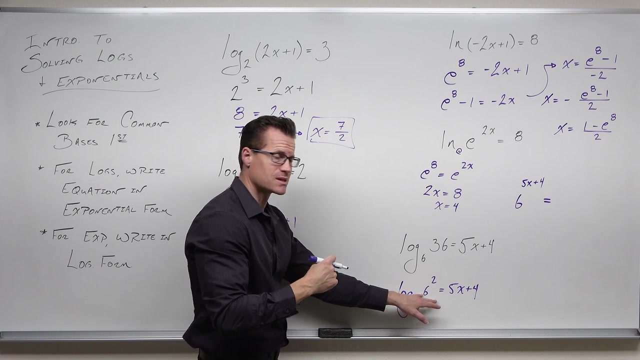 in exponential form. that's my base, That's my exponent. that's been separated. So writing this back in exponential form would say: base of 6 to an exponent of 5x plus 4 must equal whatever's here in the argument: 6 squared. 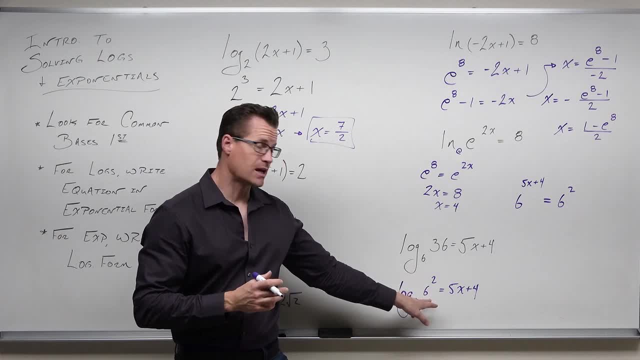 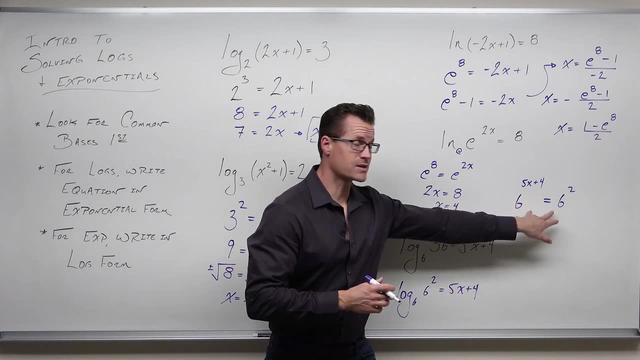 And now it's really, really clear that if your bases are the same here, they're going to be the same in your exponential. If your bases are the same here, you're going to set your exponents equal. If your bases are the same here, you're going to set your 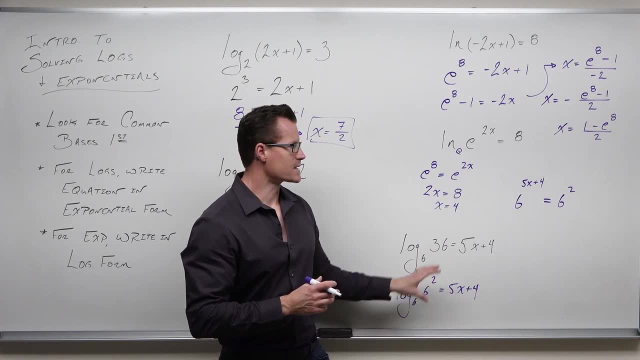 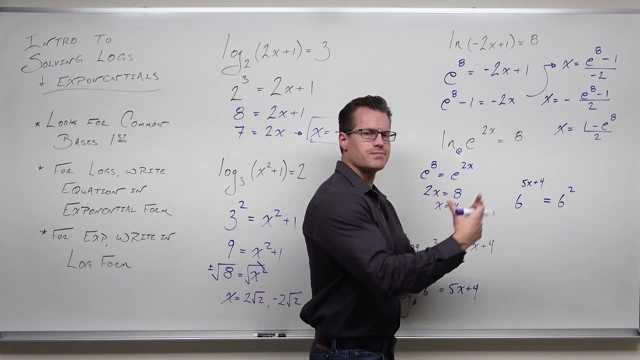 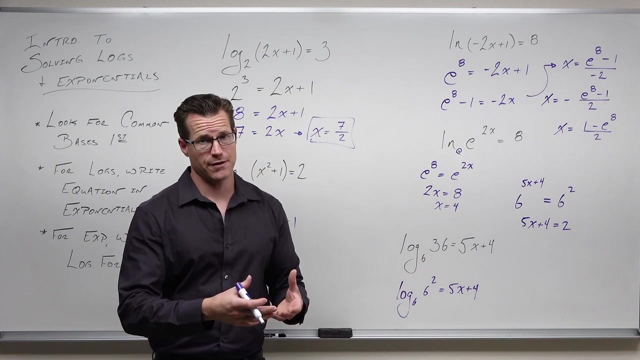 exponents equal. This models a little more concisely what this is saying to you. It's just saying you've composed a function with its inverse It's going to cancel out. Same basis it's going to cancel out. So if we have those bases the same, the exponents also have to be. 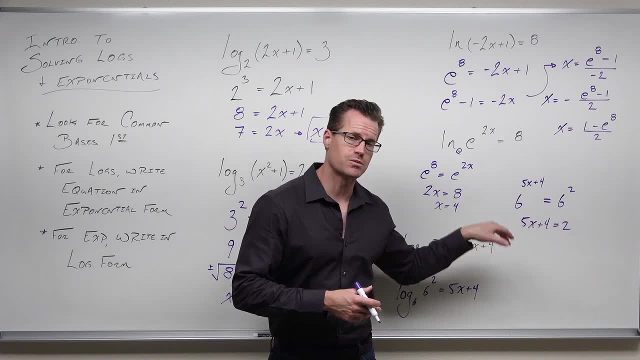 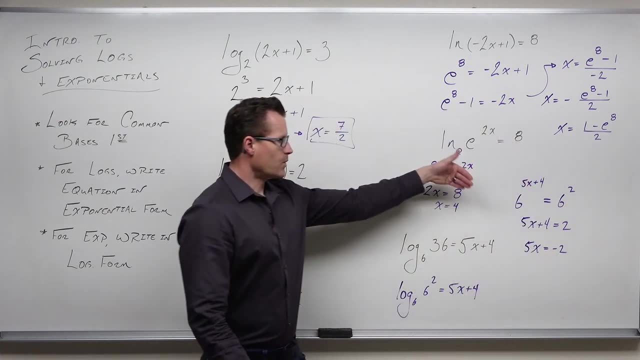 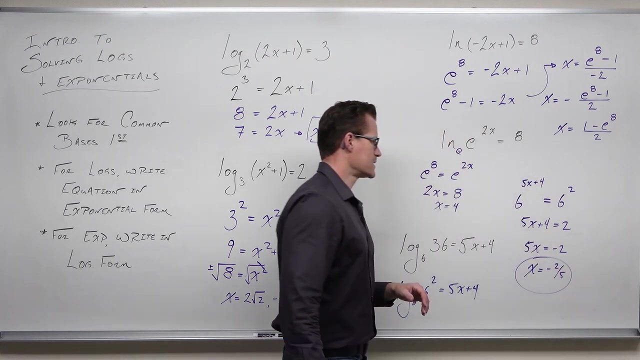 equal, And then we can solve this as exactly what we thought would happen. If we subtract 4, and we divide by 5,, we get x equals negative 2 fifths. Negative 2 fifths times 5 will give you negative 2,. 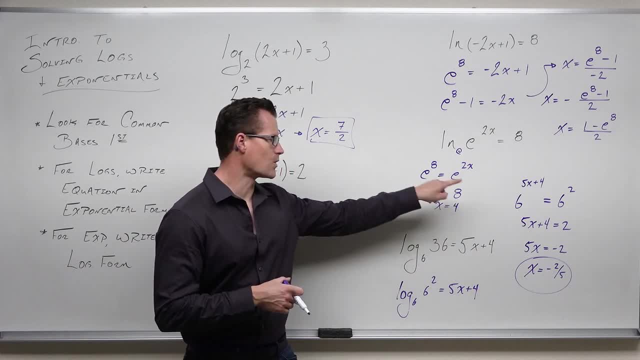 plus 4 will give you 2.. And, sure enough, 6 to the second power is 36.. We can check our work on that. I hope that makes sense to you. I hope you're seeing the necessity of writing a lot of these. 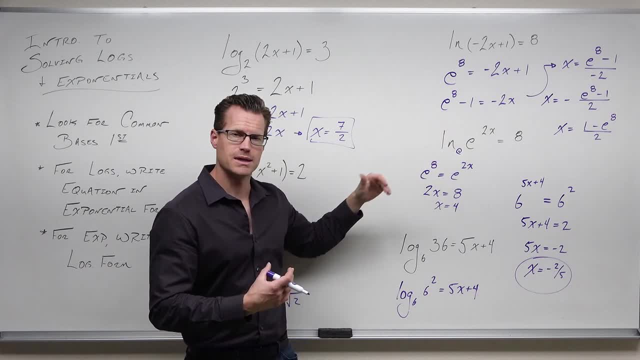 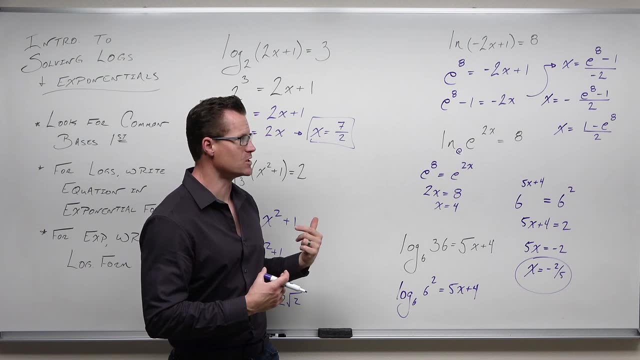 in exponential form. That's how we're going to solve this. So, if you're going to write this in exponential form, that's how we solve logarithms in general. Yes, there are some shortcuts. if we can find common bases somehow, That's true, We can simplify this a little bit easier, But without 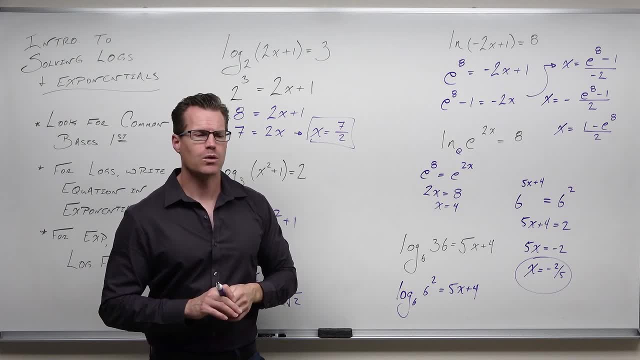 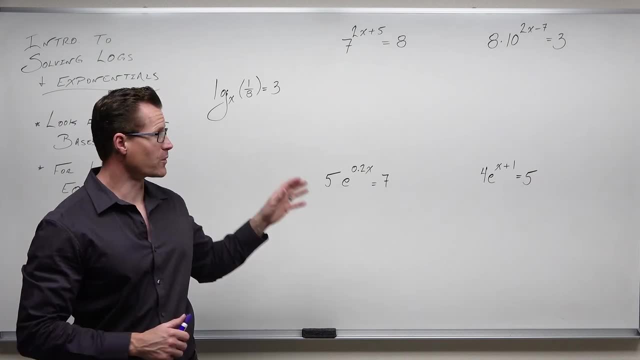 that you are going to need an exponential for logarithms in general. We'll come back, we'll talk about exponentials and then we'll be done. Okay, I guess I lied a little bit. I want to do one more logarithm before we jump into these exponentials. Sometimes you get a little bit of 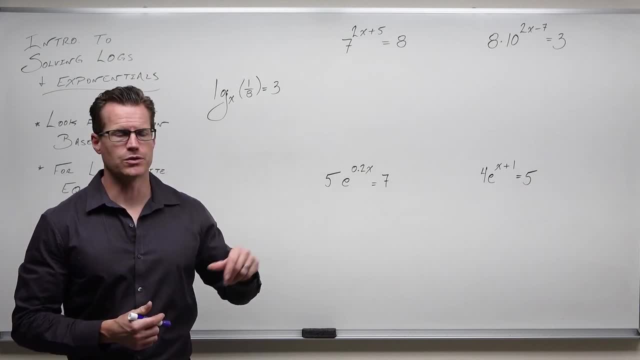 awkwardness like hey, can you solve for a base that would make this logarithm true And it's not that bad. Just remember that with your exponentials you're going to solve for a base that would make this. You check your common bases. I do not have that because I don't have two logarithms. 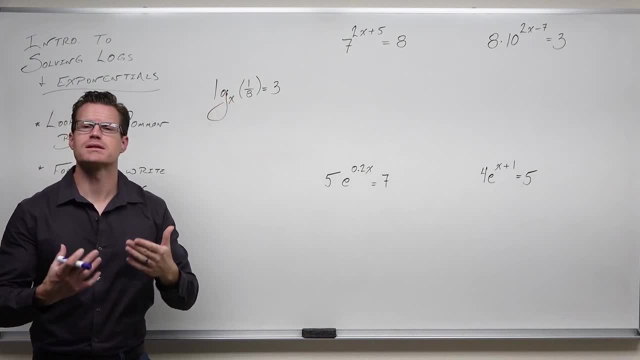 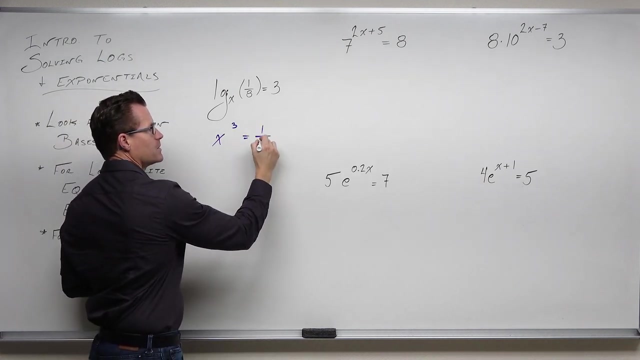 What I do is I have one logarithm, isolated and equal to a constant. This is the setup for solving with an exponential. We look at this and say: can I write this as an exponential? Well, identify what your base is. A base is x. Identify what your exponent is, In this case, 3.. And that's going. 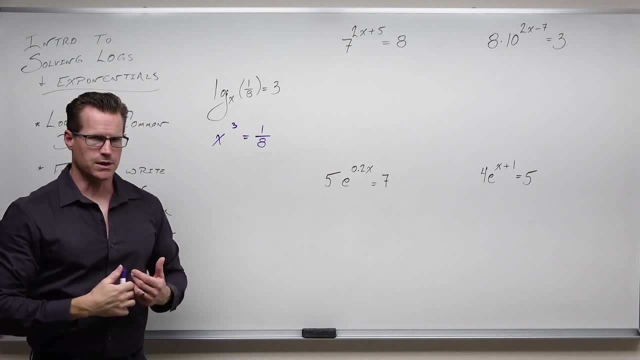 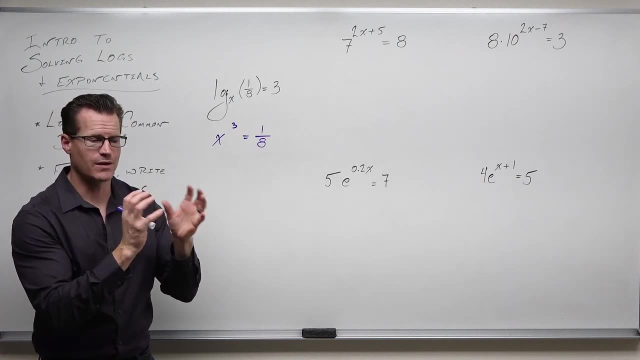 to be equal to your argument. When you solve these, just be careful, Remember that your argument has to be positive. Your domain for logarithm is positive numbers, So whatever you plug in must keep that or make that positive. But your base also has to be positive. It can be fractions, That's. 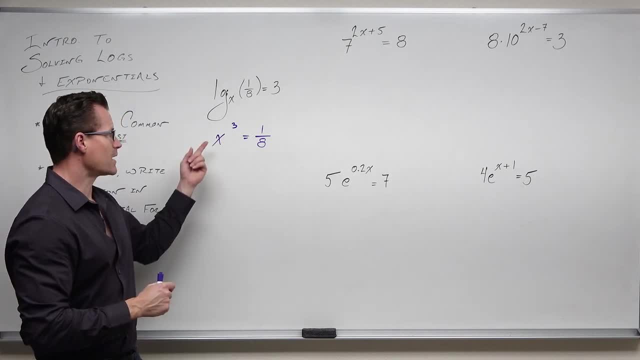 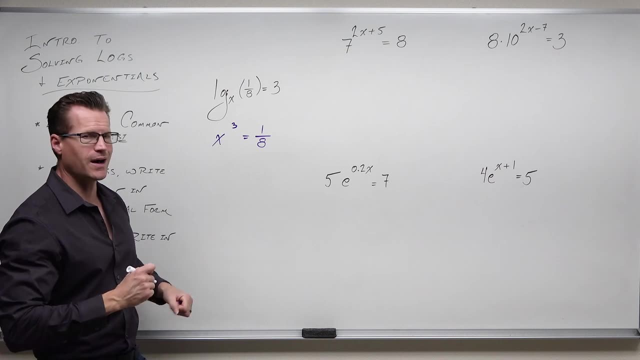 okay, but it has to be positive. So if you had a square root here and not a cube root, when we took a plus and minus, you would have to omit any negatives. Cube root's fine, You can take this and take a cube root and not get any negatives here, but you'd have to watch that Just remember. 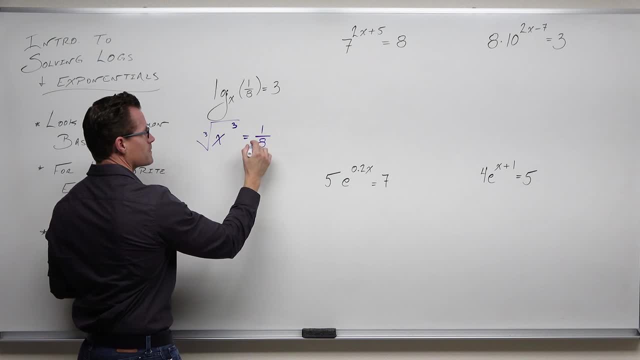 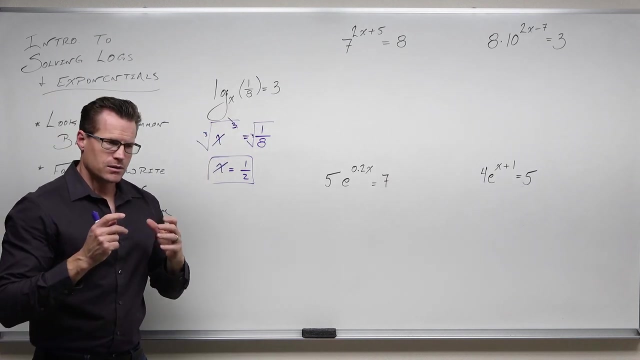 your bases can't be negative. So take a cube root of both sides. Cube root of 1 is 1 and of 8 is 2.. So the base that makes this work is 1 half And, sure enough, 1 half to the third power is 1 eighth. That's what this would say Again last time. just be careful. 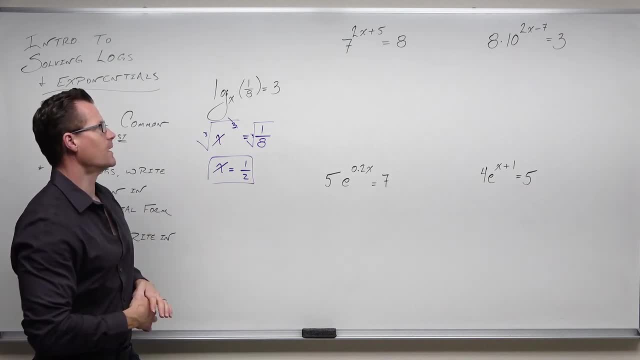 that you don't allow any bases to be negative. So this works. You still write this as exponentials. That's how logarithms are solved in general is with its inverse of an exponential. Now let's move on and solve some exponentials. So the same logic applies. 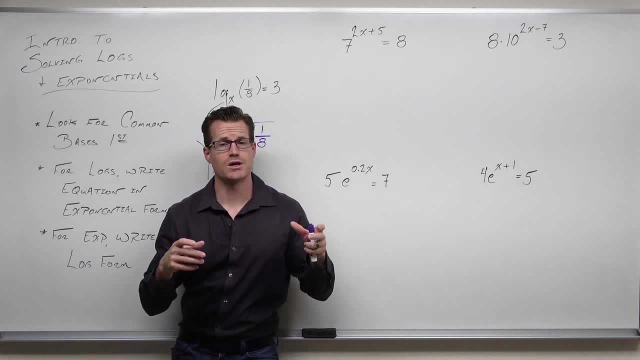 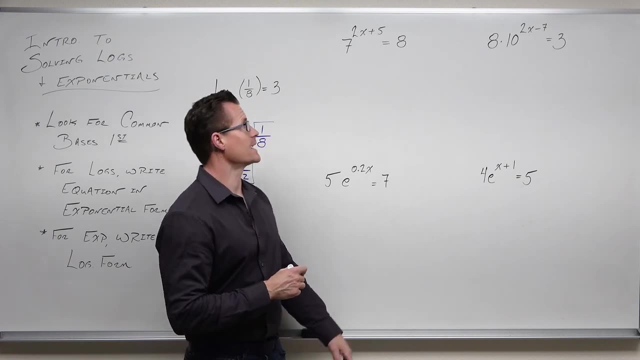 It's just that we're going backwards. You see, logarithms and exponentials are inverses of one another. It means that it takes one to solve the other. So we would check for common bases, And here's what I mean by that. You look at this and say: can I write this as this base, If you can? 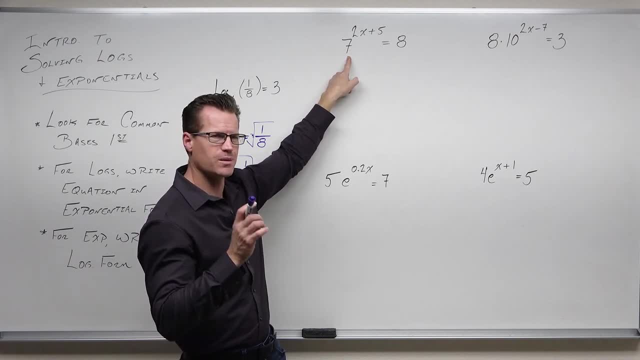 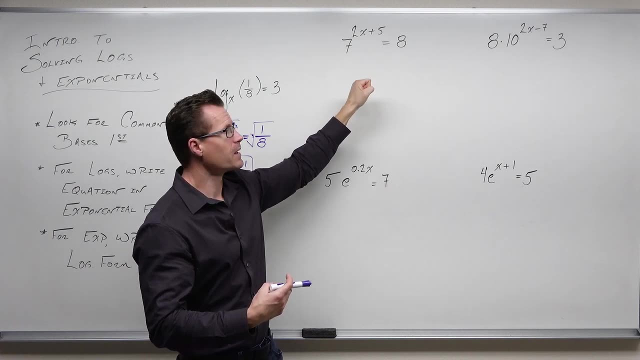 then you do it because it's a little bit nicer, You don't have to use any logarithms. You'll get a more easy to understand solution. But if we don't have that, then we're going to have to find a logarithm And we're going to have to use that to solve our exponential. So in each of these, 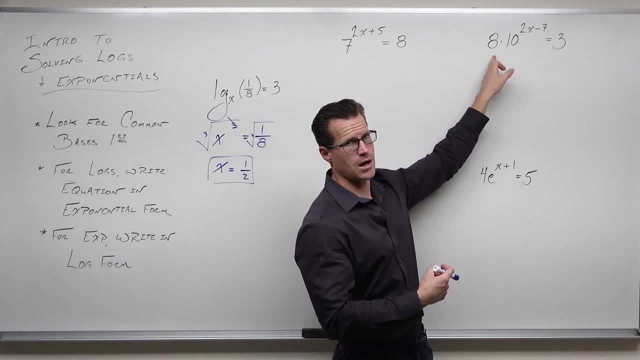 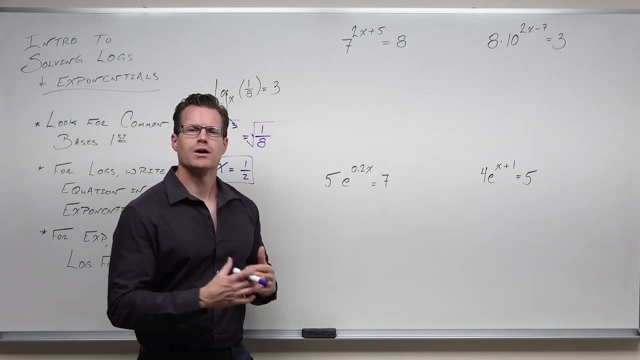 7 and 8, you can't find a common base. 10 is your base, not 8 and not 80.. 10 and 3, you can't find a common base. E and 5, definitely no common base. E and 7, no common bases. So we would check. 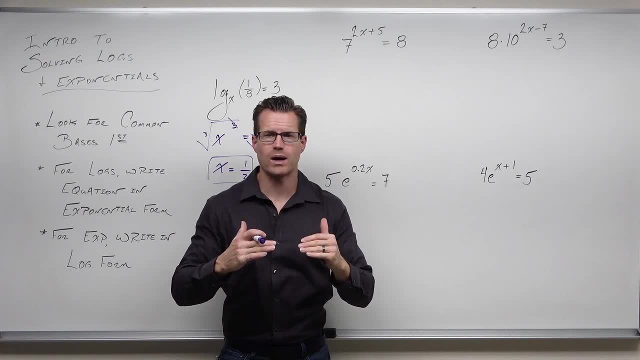 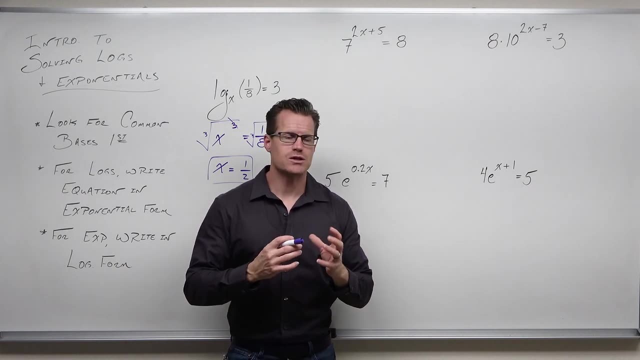 that. first, though, Once we've determined there are no way to write these exponentials as a common base, we're going to have to use a logarithmic form to solve the exponential. It's not too bad When we get into a little bit more detail. I'm going to give you at least three, possibly, if I 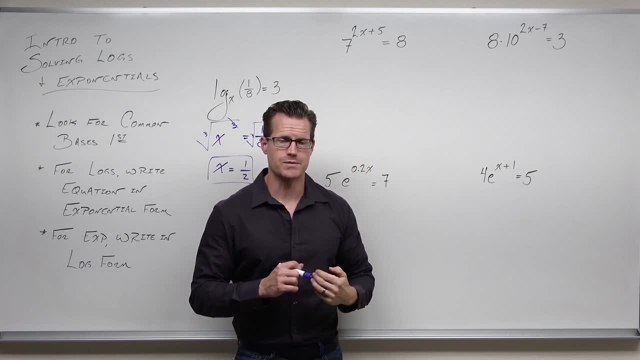 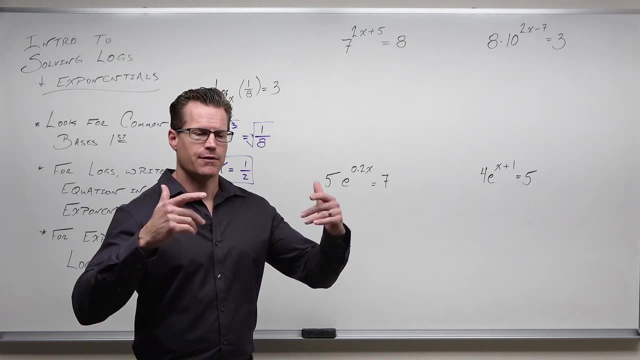 feel like it, four different ways to solve exponentials with logarithms. So we've checked common bases and we don't have any common bases in any of these problems And I just need you to know that if you do not have common bases with exponentials, it is going to take logarithms to 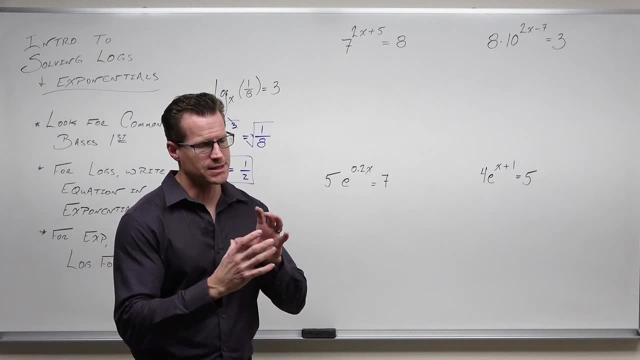 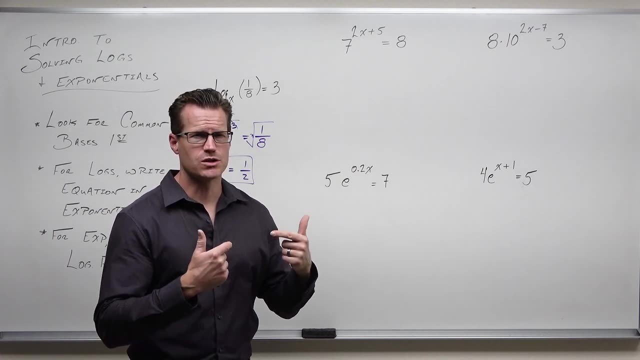 solve them. We're going to isolate the exponential. What that means is get the base raised to an exponent by itself, and then we're going to solve. As I was saying a little earlier, I will teach you some other techniques when these become a little more difficult, Like: what do you do if? 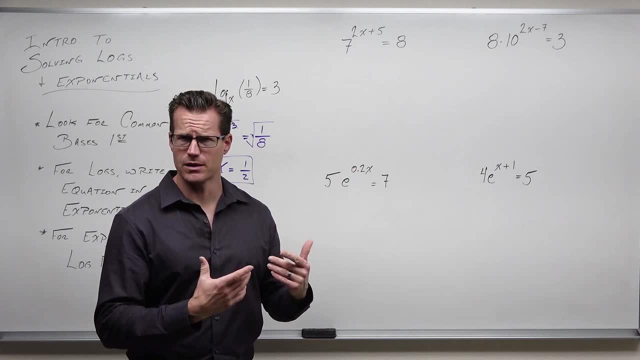 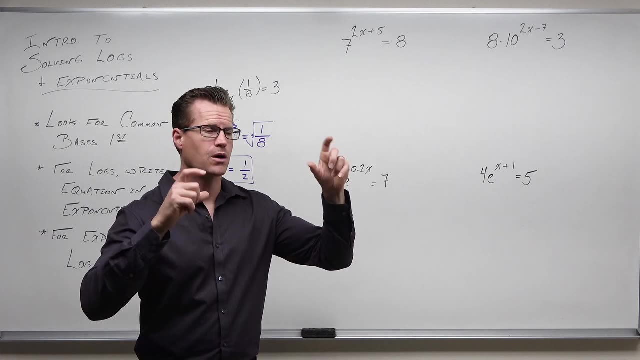 you have common bases. Well then, writing this as one logarithm is not going to work, And so I'm going to show you that in another video. This is very basic, Just the introduction of: Hey, if you have exponentials, check for common bases. if not, write them as a logarithm, and then we can solve. 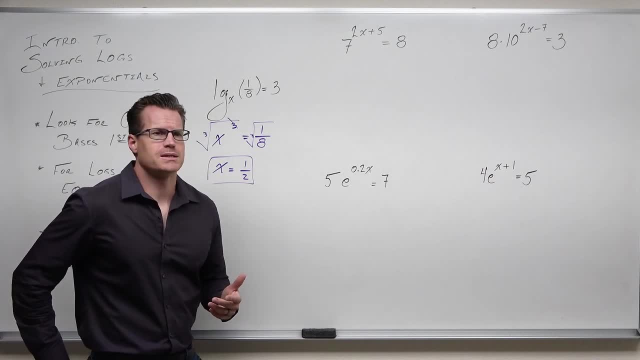 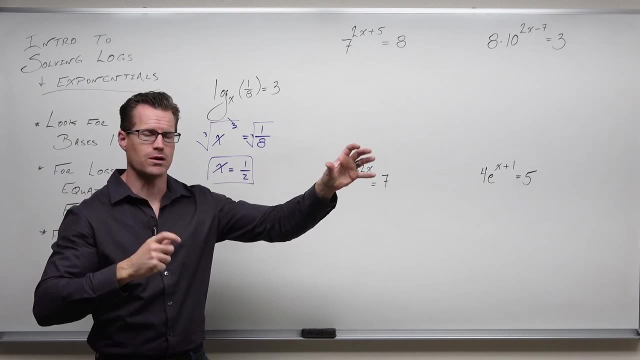 that. So let's practice that here. So this is an exponential, It's got a base of seven, It's got an exponent of two X plus five. What a logarithm does? a logarithm takes that exponential and breaks it apart. It takes the base and says: this is the base of some logarithm, some inverse. 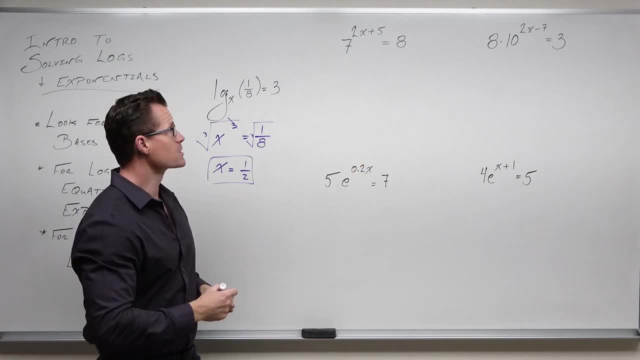 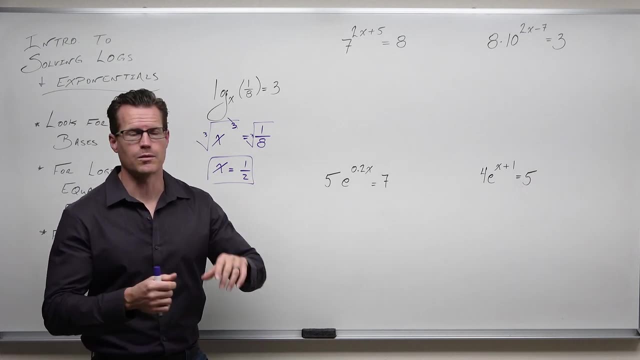 function of an exponential, And then it's going to be equal to your exponent. So we can take this and say: all right, so seven to the two, X plus five equals eight. can be written as some inverse function, a logarithm, with the: 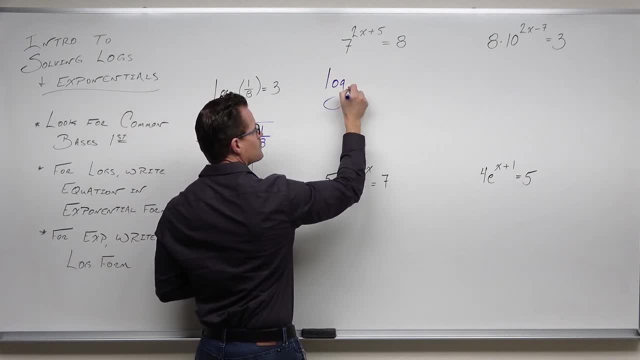 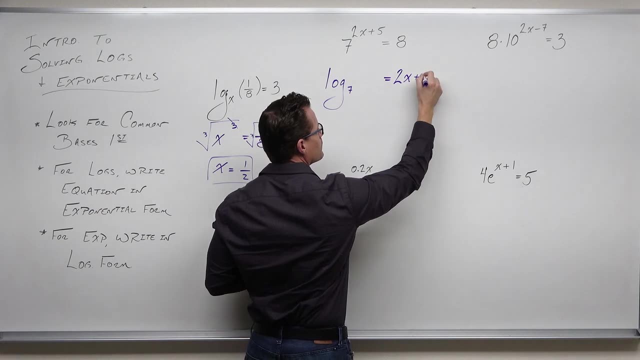 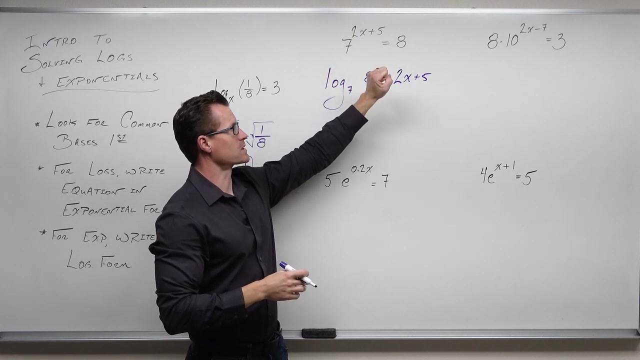 same base, equal to the same exponent, but just separated. It just says the same thing. a little bit weird. It says seven to the two, X plus five equals eight, And it says, in order to get from seven to eight, it's going to be equal to the same exponent. So we can take this and say, all right. 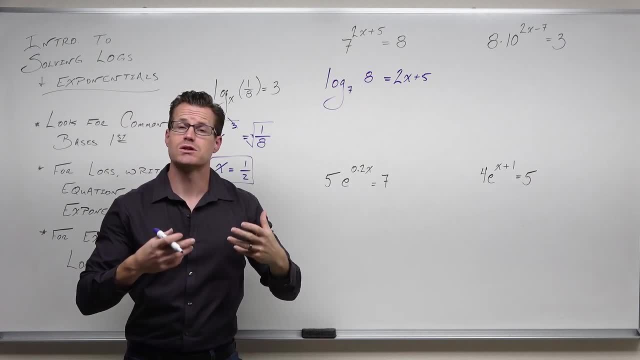 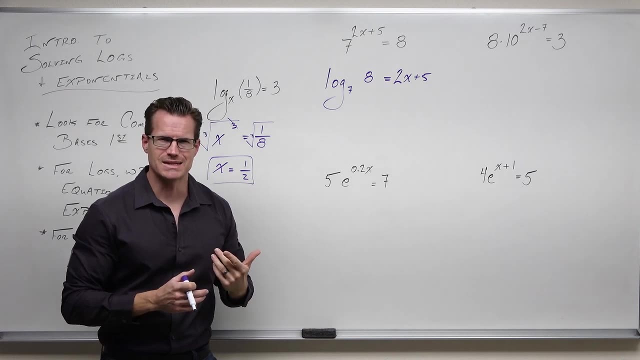 so seven to the two X plus five equals eight. you need an exponent of two X plus five. Now this allows us to solve for that variable X. Don't try to figure this out unless you have some sort of common base idea. If you do, then you can, but in general you wouldn't need a logarithm to do that. 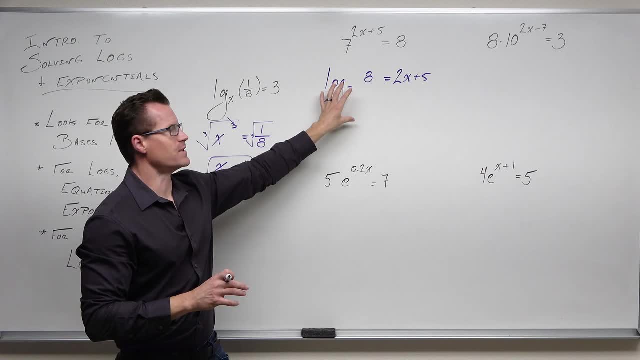 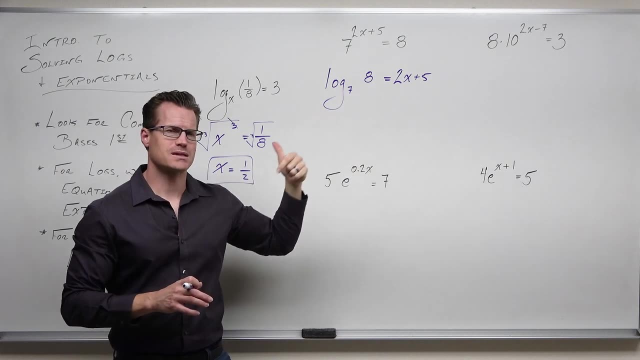 It would show up right here that you can get common bases. Just leave this. This is going to be what's called exact answer. If you, if you, approximate this on a calculator, yeah, we can get something out of it, but it's you're going to lose a lot of the um, the exactness of it. It'll. 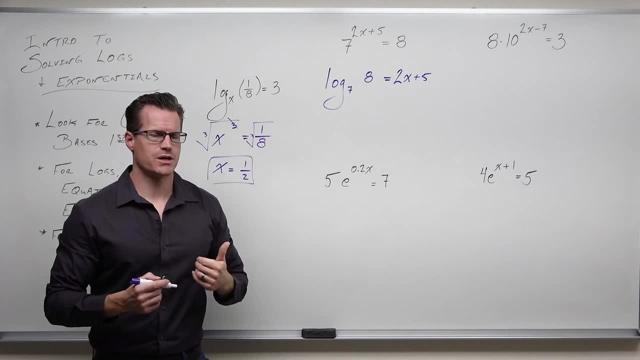 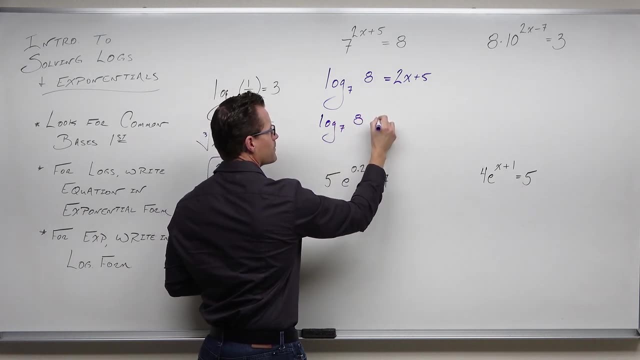 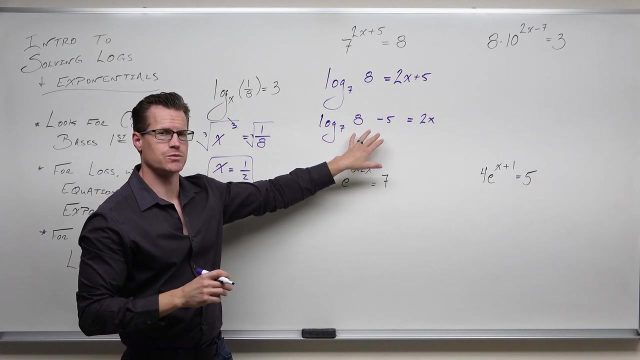 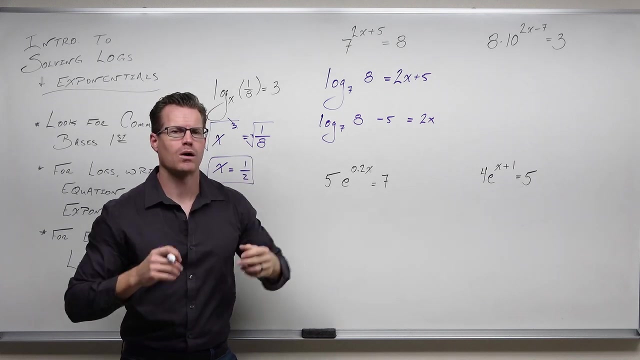 just be an approximation. So when we solve for X, a couple of features to understand. when we subtract five, it is really important to not actually subtract the argument of your logarithm minus five. This is inside a logarithm and this is not in order to get inside the logarithm. 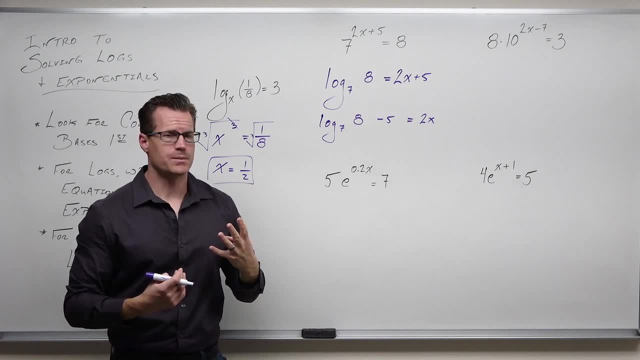 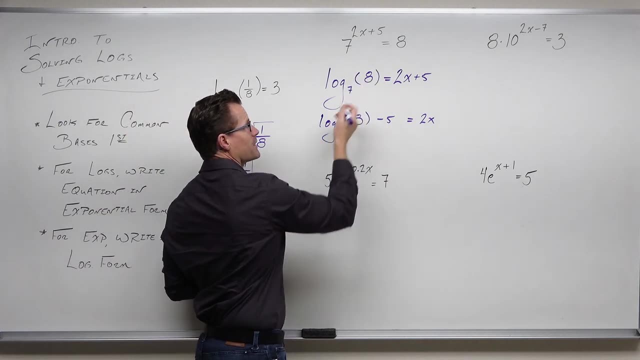 You need properties of logs to do that, And there's really only four of them. Uh, so we cannot just subtract, even though we want to. it's best to put a parentheses around that argument almost all the time. I can only think of a couple of cases where you wouldn't want to do it And you 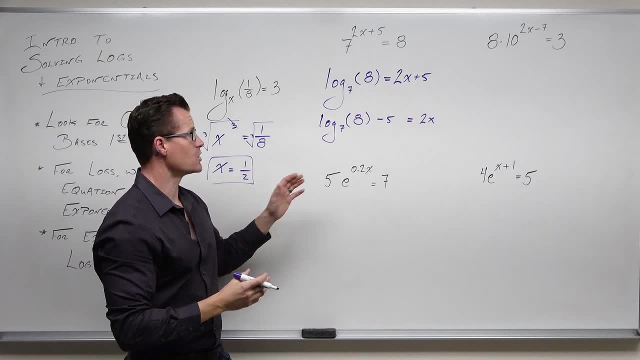 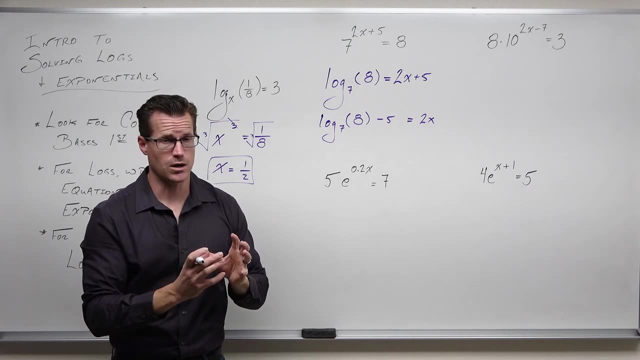 can't really overuse the parentheses here. with this logarithm It's going to show you: this is log base seven of eight, and then you subtract five. It is not log base seven of eight minus five. That's not appropriate. You can't do that. Lastly, if we divide by two, 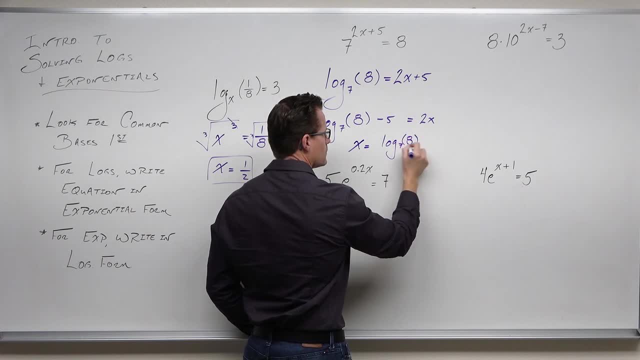 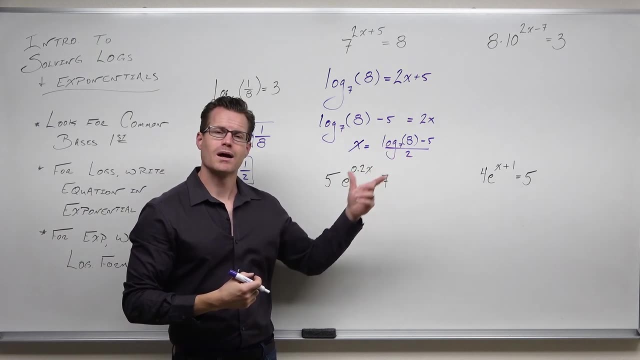 the whole entire expression is divided by two. This, even though it's awkward, that is an exact solution And it's also a constant. This stands for one number. It just has a weird logarithm in it. Your calculator will approximate this If you have the ability to plug in a base of seven. 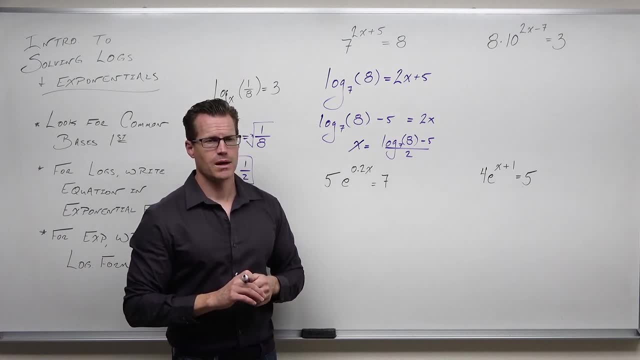 a lot of calculators don't. Most Texas instruments don't do that. They either have a log base 10 or a log base E, that's the log and the L. Some of them do have that base where you can plug it in, but a lot of the ones I've seen 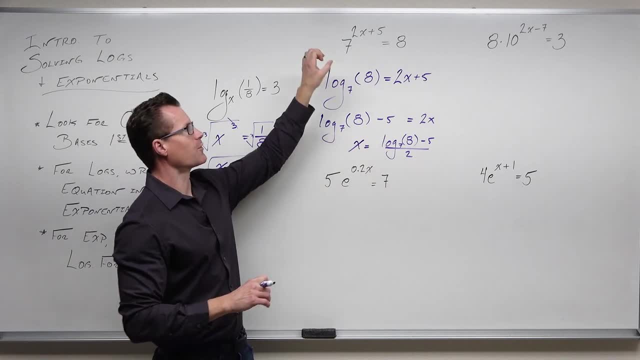 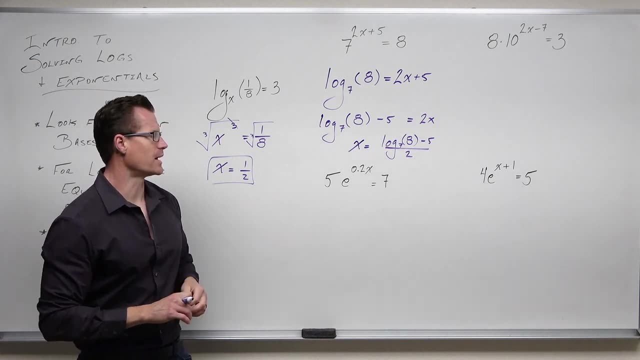 don't have that. So this is an exact solution for that exponential and we had to have logarithms to do it. Let's move on to this guy. So when we move on and we take a look at five E to the point two, X equals seven. there's a lot going on, but at its root, at its heart, it's an exponential. 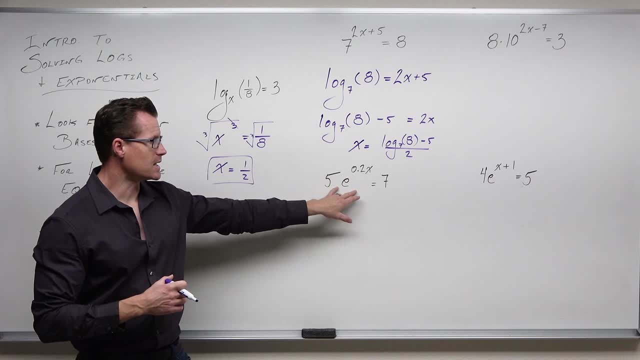 Now, can you get a common base? Well, the base here is E and the base here is seven. There, no problem. So you can get a common base. So you can get a common base. So you can get a common base. There's no way to make a seven into an E, So we're going to need a logarithm to undo this. 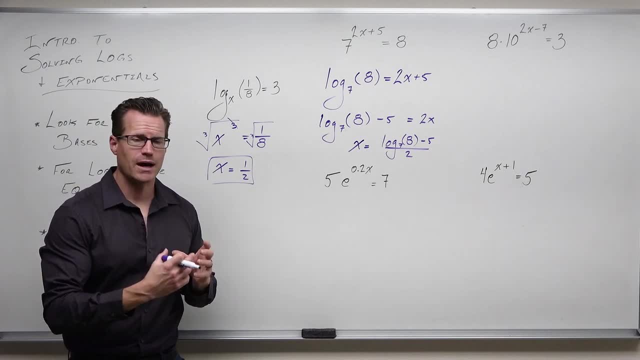 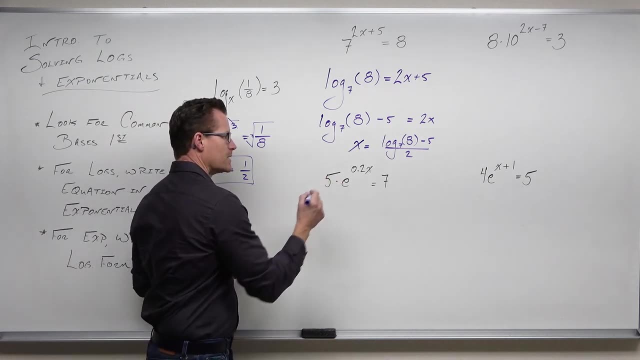 exponential. When you look at an exponential and you don't have common bases and you need a logarithm to solve it, you need to get that exponential isolated. What that means is get everything that's been added and subtracted and multiplied from that base to an exponent. 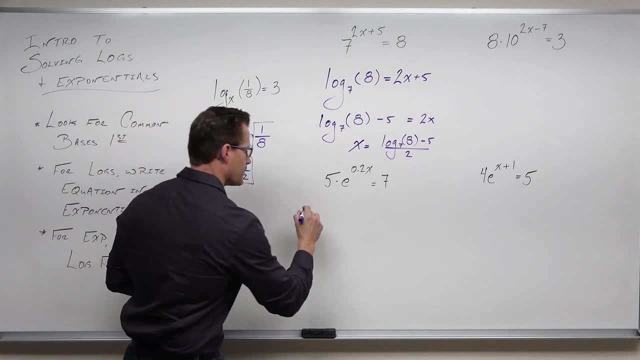 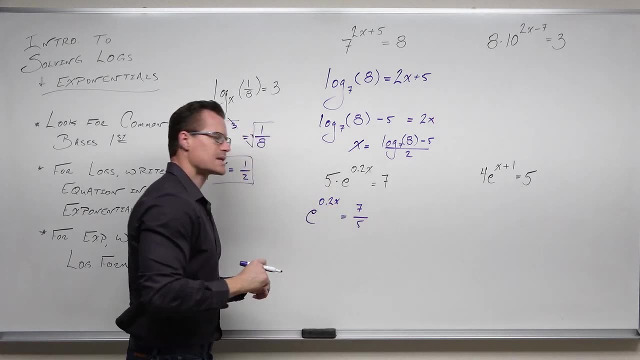 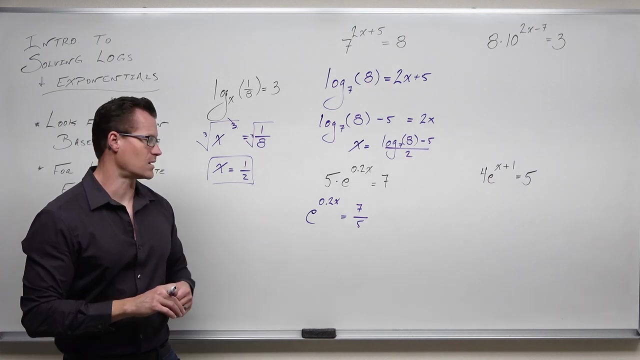 get that away. So we're going to have to divide by five here. So this is how we're going to do it. So this is how an exponential should look before you start using logarithms: Nothing added, nothing subtracted, nothing multiplied, just like this. Now, what we're going to do is say: 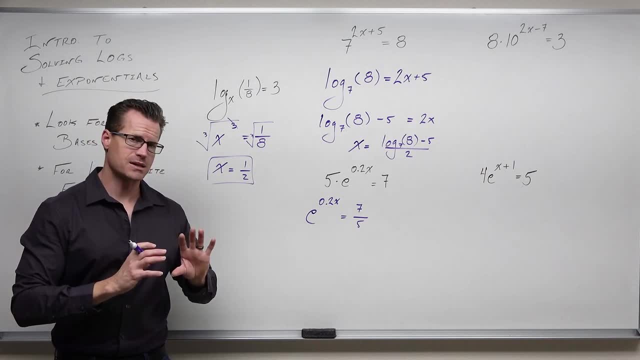 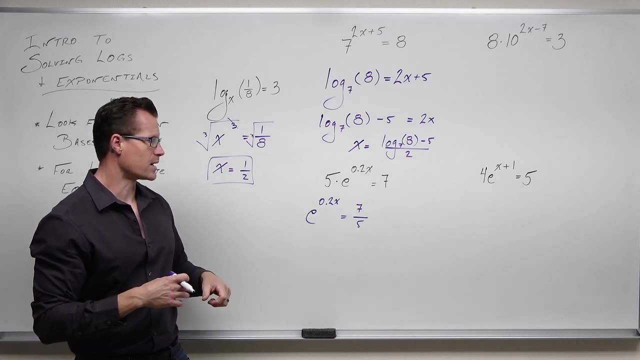 because I can write this as a logarithm. we're going to identify the base, the exponent and let the logarithm separate those things. Our base here is E and our exponent is point two X. The argument of our logarithm is going to be seven fifths. So with a base of E we'd say 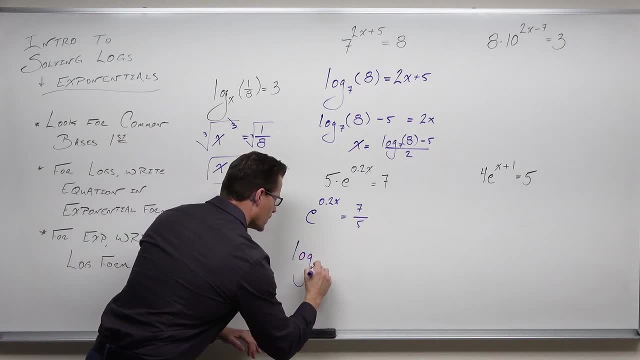 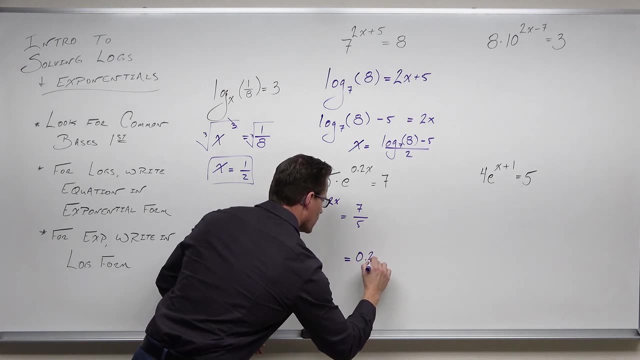 this can be written as a logarithm with a base of E. I know this incorrect notation. we're not going to use it. I'm just showing you how this works. That's going to separate our exponent. So here's our base and our exponent written as a logarithm. 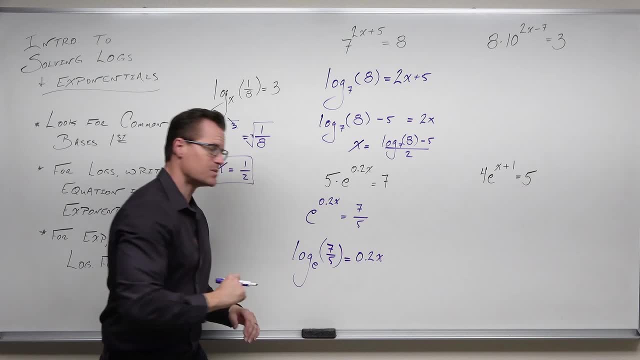 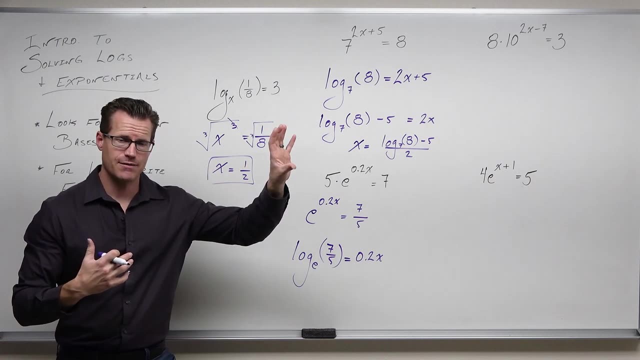 and this will equal seven fifths. I'm going to keep this in parentheses because that is appropriate to do. We're showing that this fraction is inside the logarithm. That's different than having a log of seven over five. We don't want to have that, unless it's actually what the problem's. 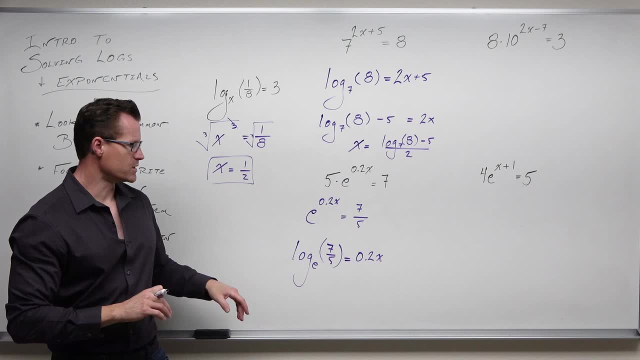 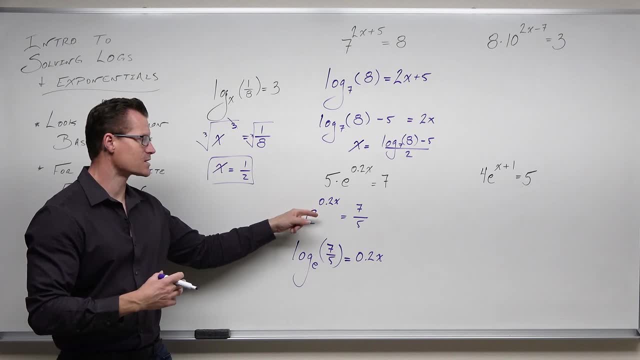 So we're going to divide by point two. So we're going to divide by point two. So we're going to always written as a natural log: LN. So when you see this, we really should be going: oh, that's. oh, this is going to be a logarithm of the base of E. I would normally just go straight to. 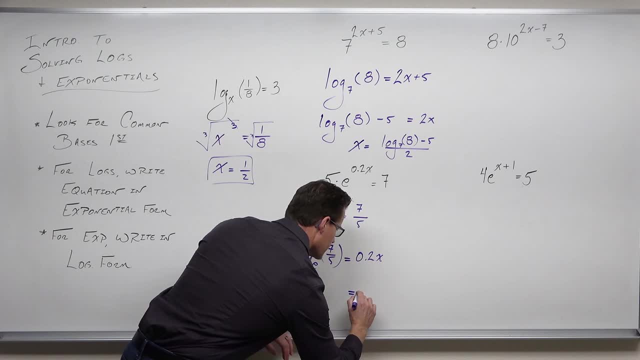 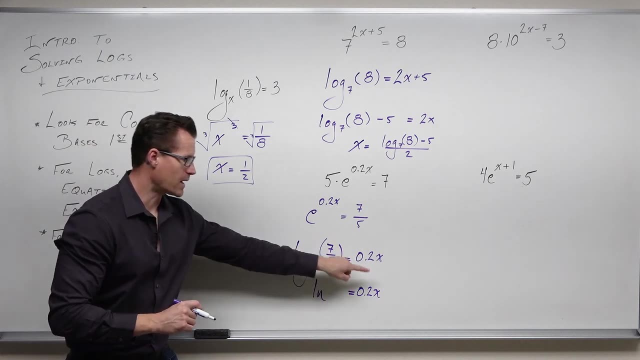 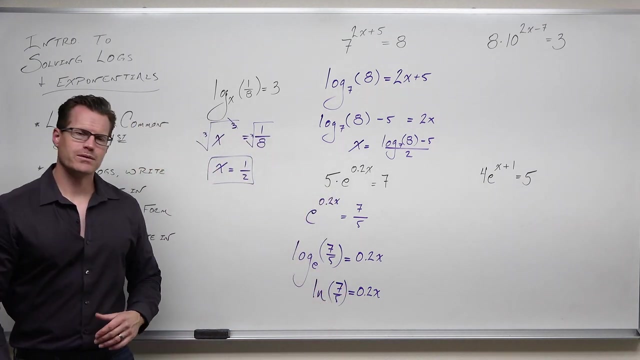 the LN. So this is log base E. So I've separated my base in a logarithm equal to my exponent and then put the seven fifths inside that natural log. And then when we divide by point two, the reason why we want to divide by point two is because we're 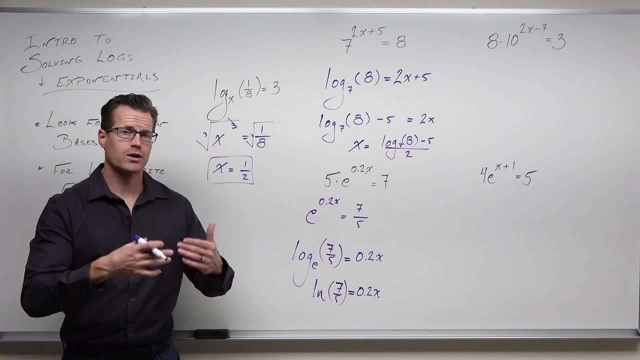 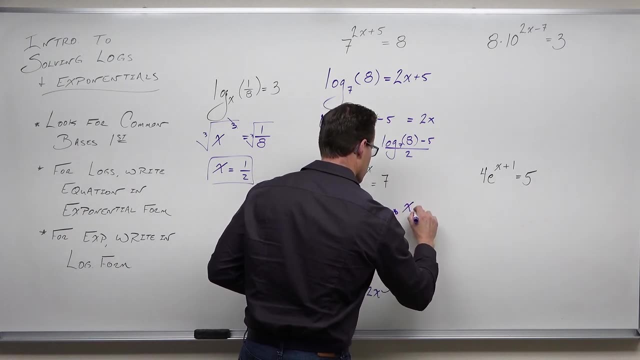 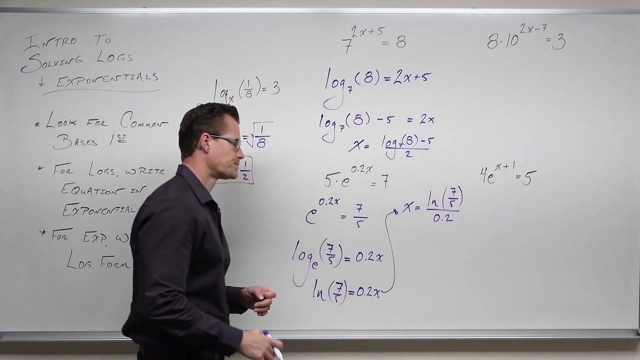 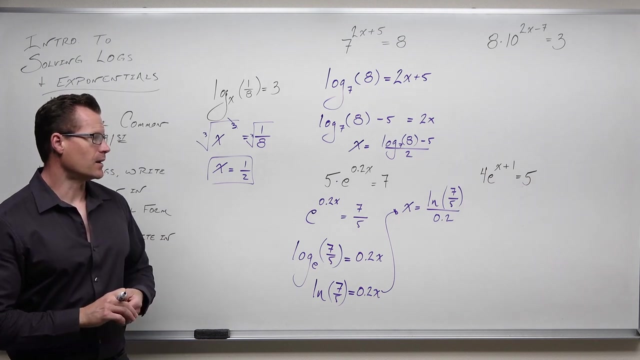 going to put that fraction in parentheses So you don't get confused on where you're dividing by point two. You're dividing this entire thing by point two. We can do a couple things to modify the look of that, like multiply by 10 over 10.. If you want to get rid of that decimal, 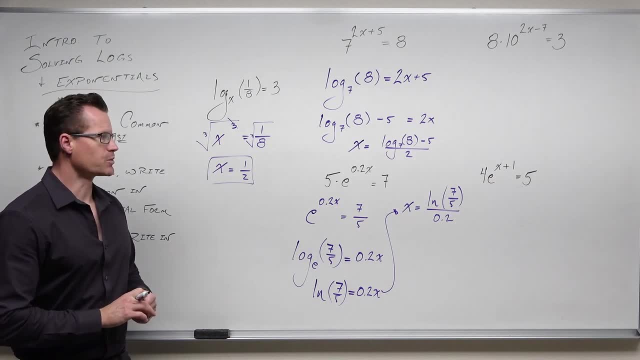 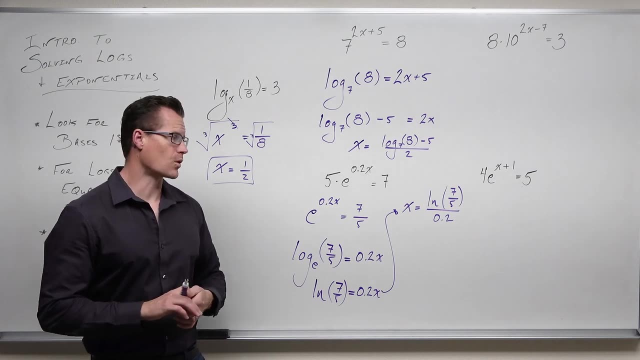 that's, that's that's appropriate. You can do that. I wouldn't say it's super necessary, but sometimes you're required to do it. So multiply by 10 over 10, you get 10 LN of seven fifths over two, or you can. 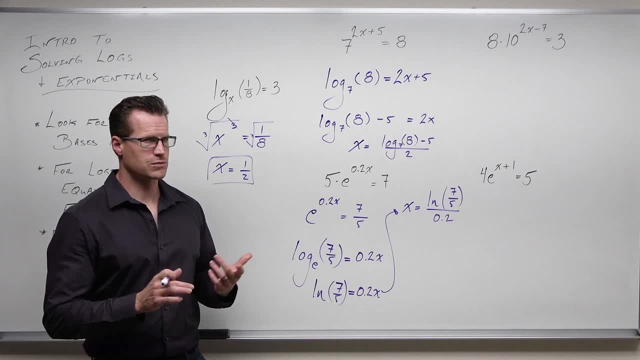 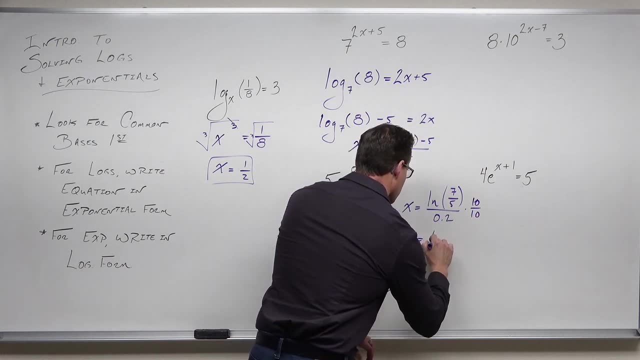 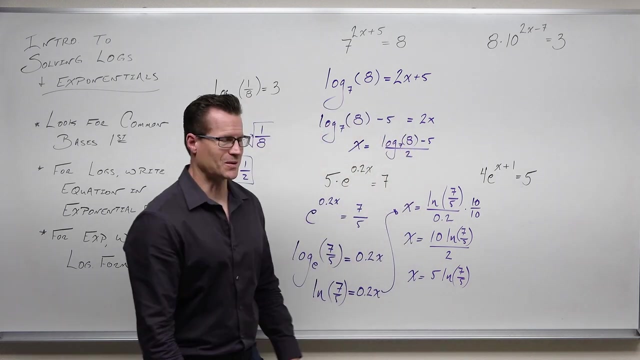 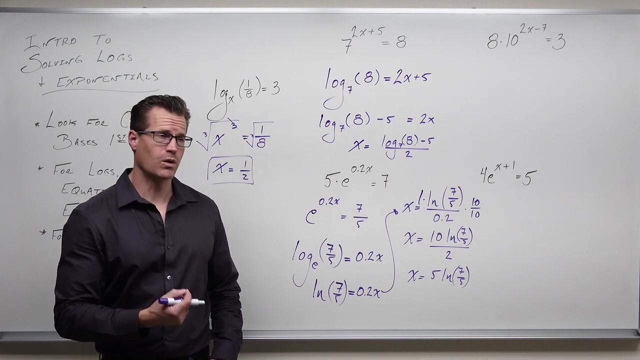 reduce that five LN, seven fifths, So that might look a little bit nicer. You could do something a little simpler, I suppose. I kind of think I made that as hard as humanly possible. If you think about that as one, one divided by point two: one divided by point two is: 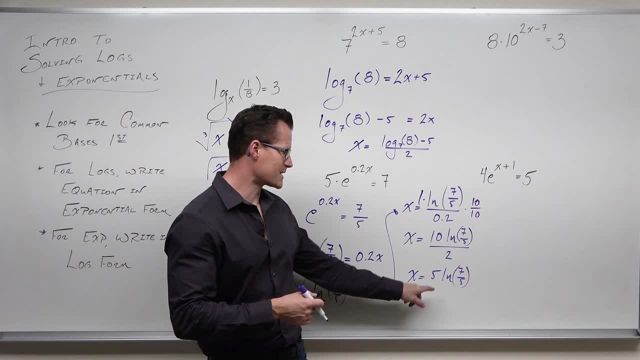 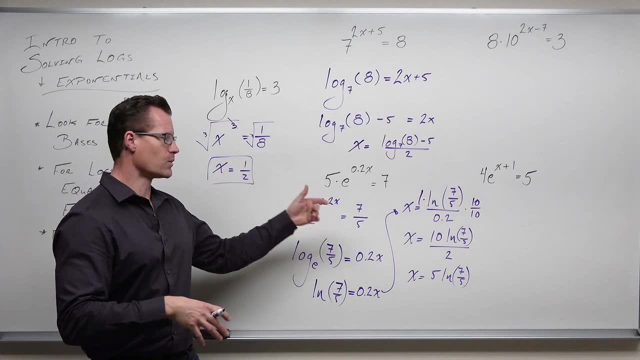 five. Point two goes into one five times, So you could do that as well, But this is a nicer look than than that is, So I hope that's making sense. I hope you're seeing that. hey, exponential is going to require a logarithm. There's another way to solve that besides using a logarithm, with a. 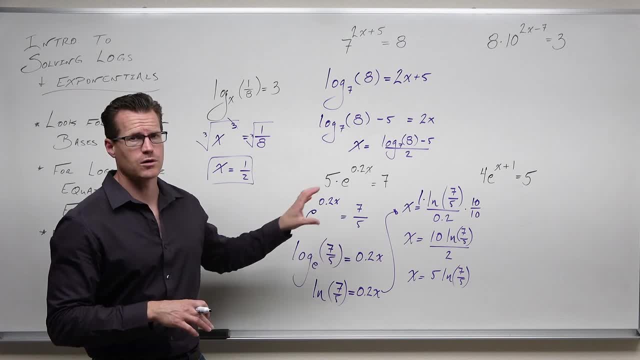 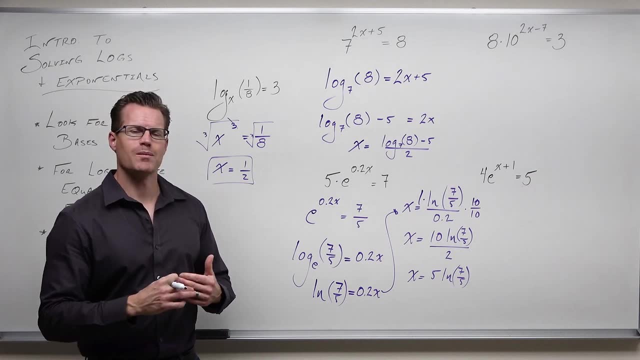 base of E. There's a couple of ways we can get to that point, but a logarithm is necessary. So I'm to solve exponentials. if you do not have common bases, Let's move on to the last two. At this point, I'm hoping that you could solve this on your own. Can you see? that's a base of 10?? That's. 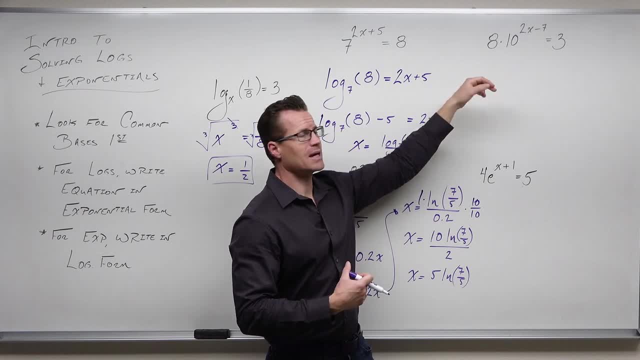 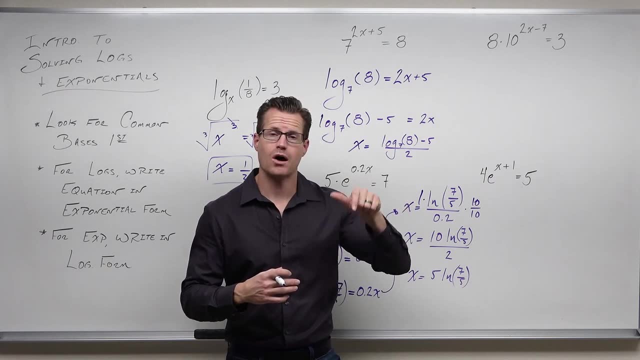 a. this is three. There's no way to make this as a base of 10.. Can you see that with this exponential without common basis, I'm going to need a logarithm. Can you also see that that logarithm is going to be a common log? It's going to have a base of 10 in it, but I need to get that eight. 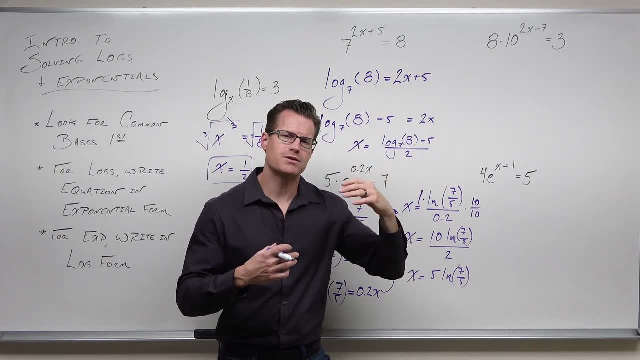 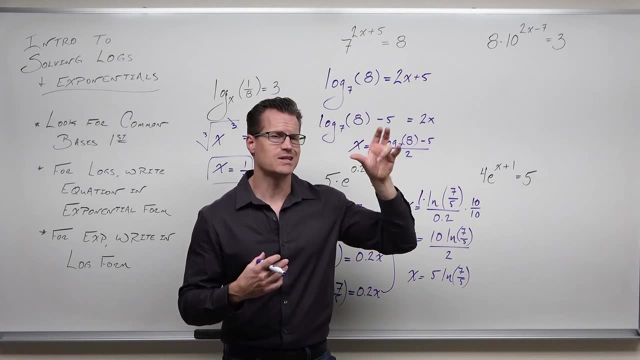 away before I write this in logarithmic notation. So I'm going to have to divide both sides by eight. So I'm going to have to divide both sides by eight. So I'm going to have to divide both sides by eight. This is not 80. You're breaking order operations if we do that. Order operations say you have to. 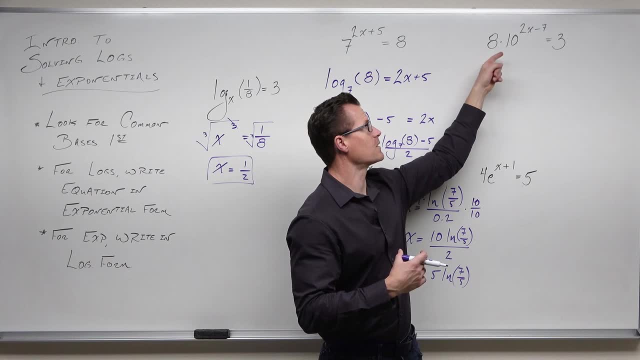 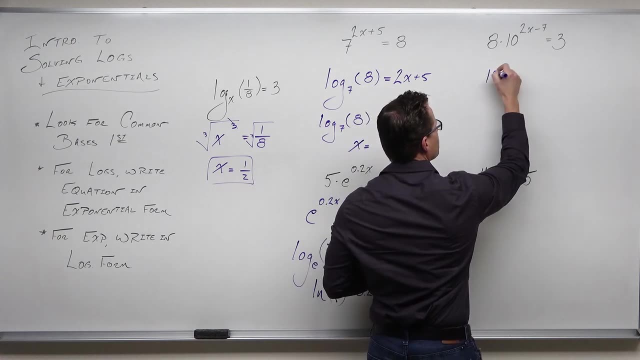 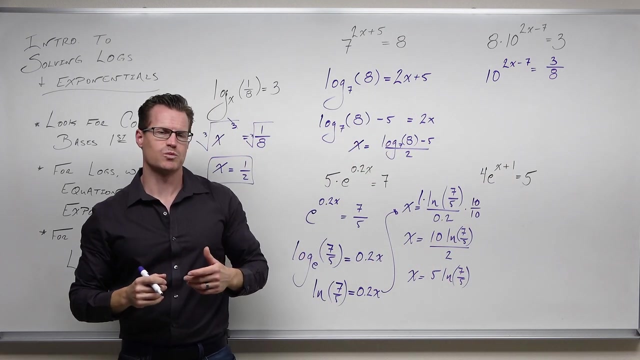 deal with the exponent before you start multiplying. If you start multiplying here, you are really messing up that exponent. We don't want to do that, So we're going to have to divide both sides by eight. Now, that's how we like to see an exponential before we make it into logarithm. 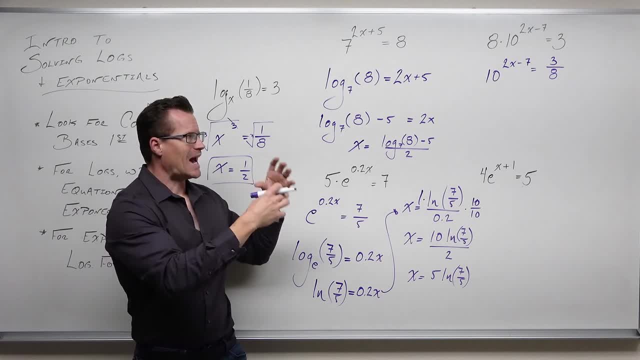 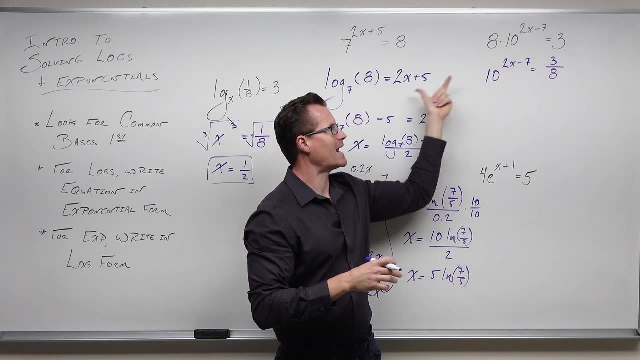 We got a base, We know it's 10. All by itself, nothing added, subtracted or multiplied onto that exponential. This is okay because it's in the exponent. but what I mean is multiplication here, or added, subtracted, somewhere outside of that base, to an exponent idea. Now that we know, a logarithm is: 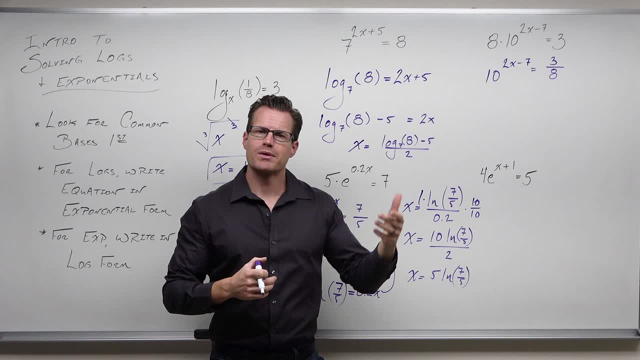 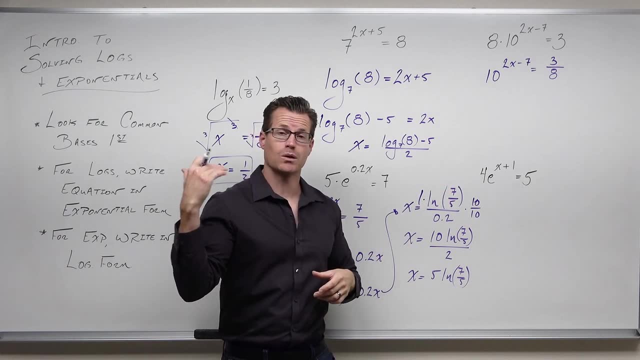 going to be necessary for us. if we have a base of 10, remember that a log with a base of 10 equal to the exponent of 2x minus 7, that log should be written, just log. If we write log with no base, 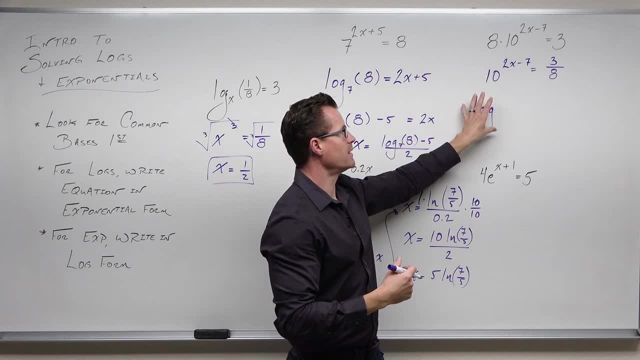 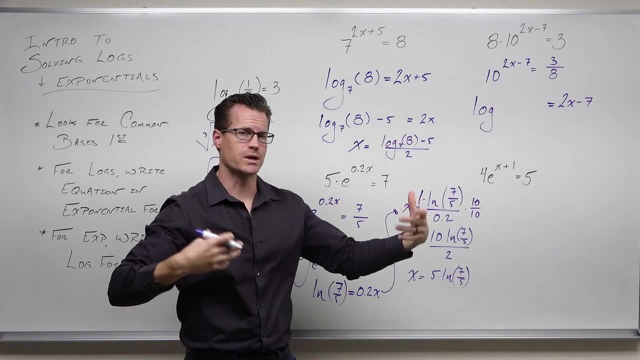 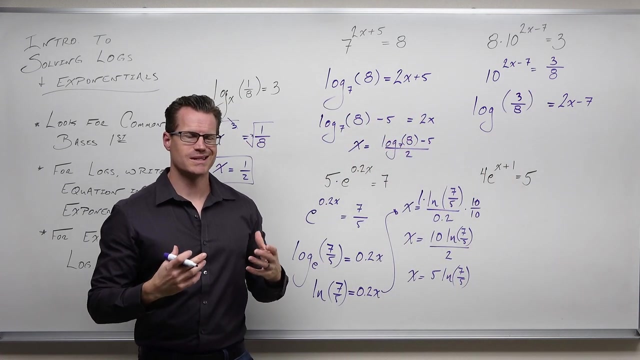 it's implied that that base is 10.. So I have a base of 10, an exponent of 2x minus 7, and a logarithm separates those. I'm going to make sure that my argument is in parentheses. That's a really good form to do. 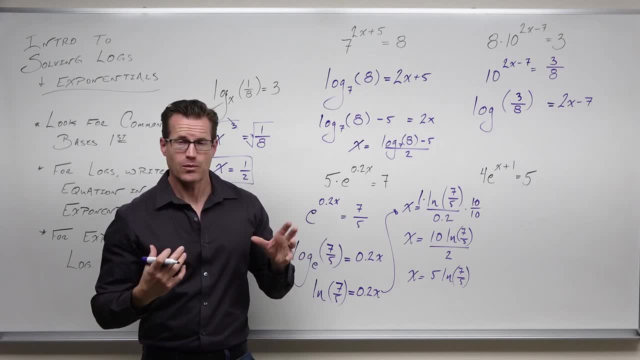 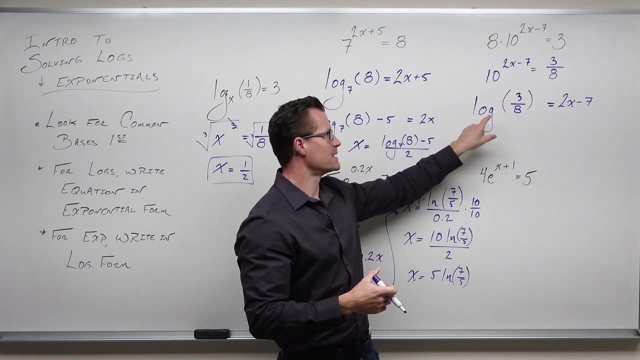 That way you don't accidentally add, subtract, multiply, divide anything inside of that without meaning to by some sort of property of logarithms. And then we solve for x, because this is actually a constant. This says 10 to what power gives me 3 eighths. That is a number It represents. 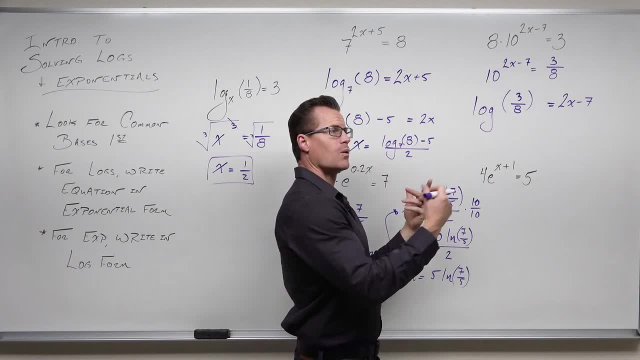 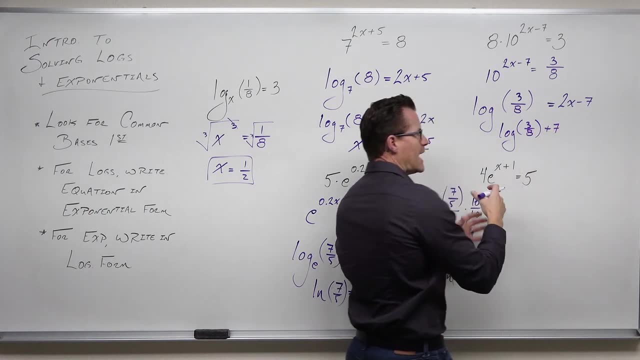 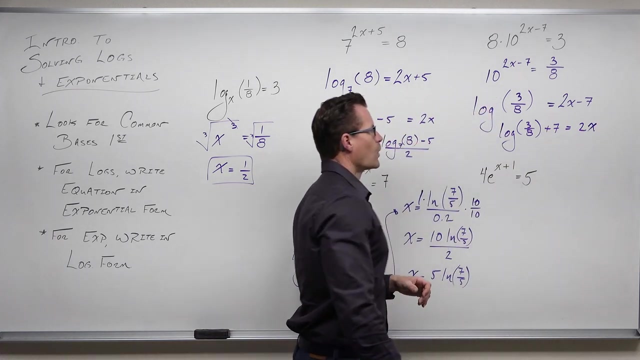 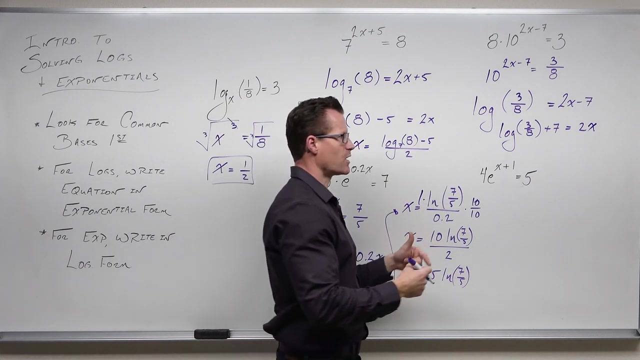 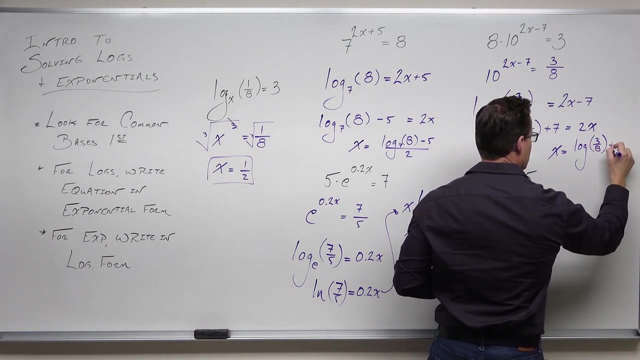 an exponent, but I can solve by adding 7 and dividing by 2.. Where we add 7 is after that parentheses, and where we divide by 2 is that entire expression. So divide the entire log of 3 eighths. we know it's the base of 10, plus 7 and I'll divide by 2.. That's as good. 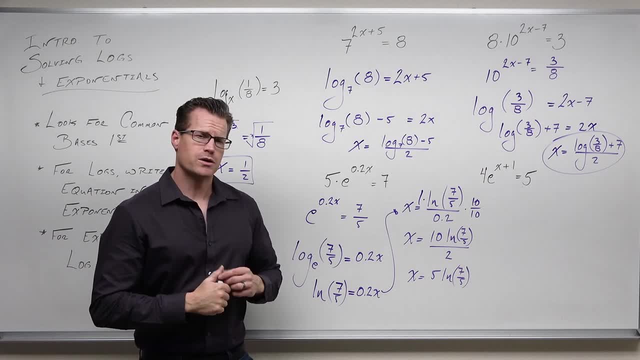 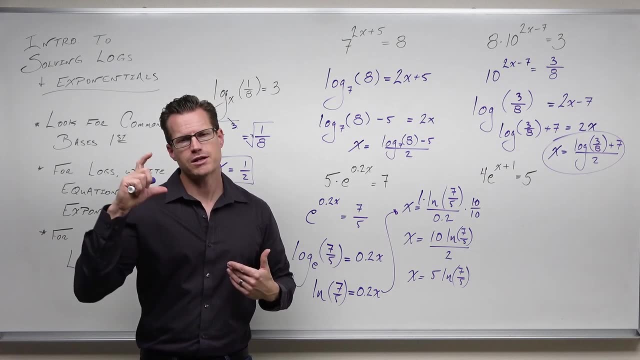 as we can get for what's called an exact solution. If you wanted to approximate, your calculator will do this. Just press the log button on your calculator. That is a log base 10. And sure enough, it has parentheses there, doesn't it? So when you press it it goes log parentheses. 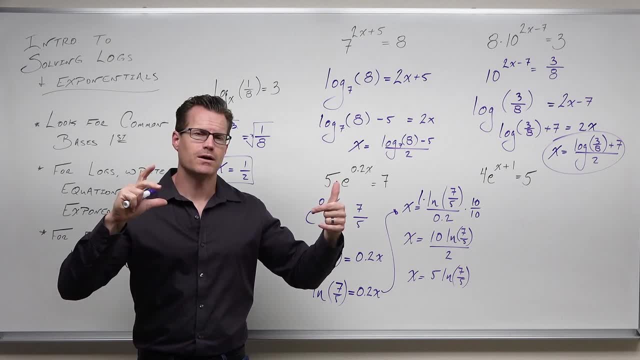 plug it in, and you're done So. when you press it, it goes log parentheses. plug it in, and you're done So. when you press it, it goes log and 3 eighths end parentheses, add 7.. Now, if you do it correctly, you might. 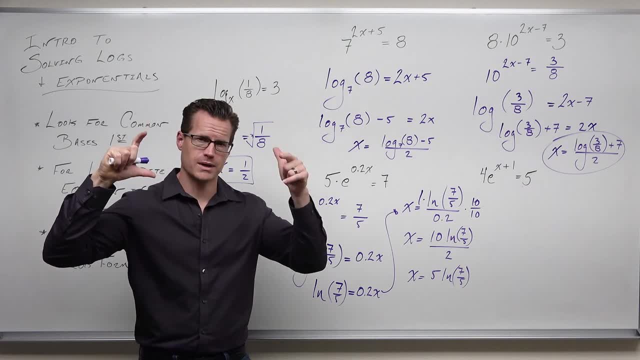 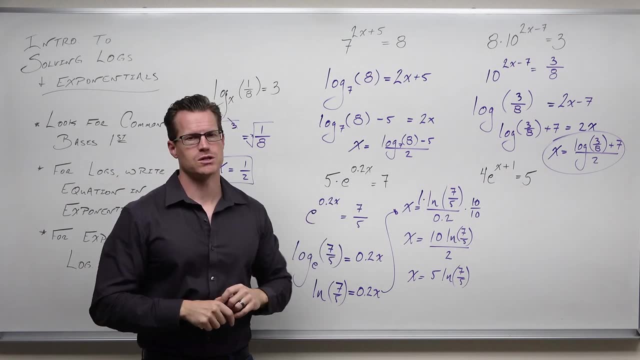 want to do your numerator and parentheses first. So parentheses, log 3: eighths: close the first parentheses plus 7, close the second parentheses and that will have the numerator for you and then divide by 2. And that will give you an approximation for what this number. 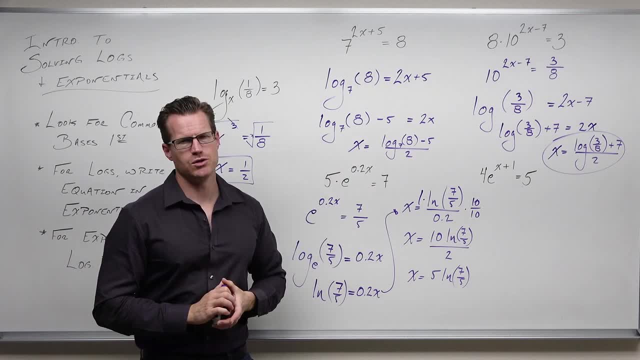 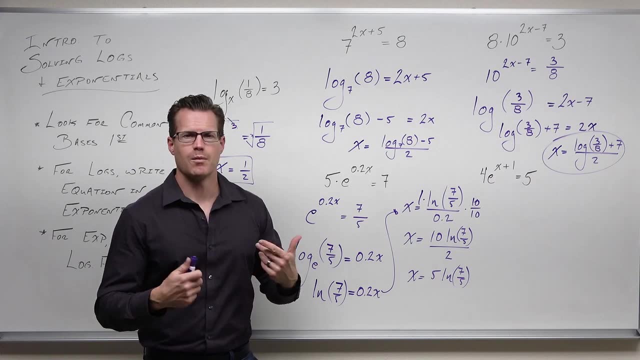 represents. Okay, last one, You really need to do it on your own. It's an exponential for sure. I'm going to kind of just scream through this thing: It's an exponential without common bases. If you have that, a logarithm is necessary. but you have to isolate your exponential first. 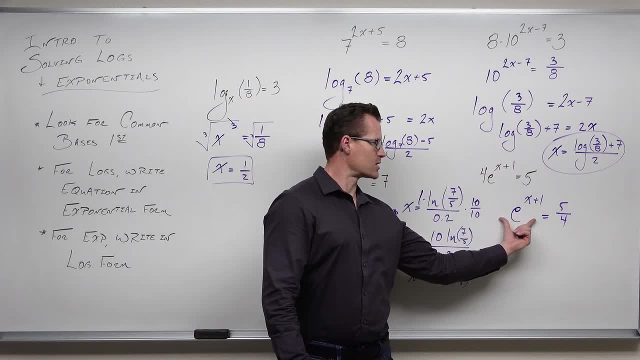 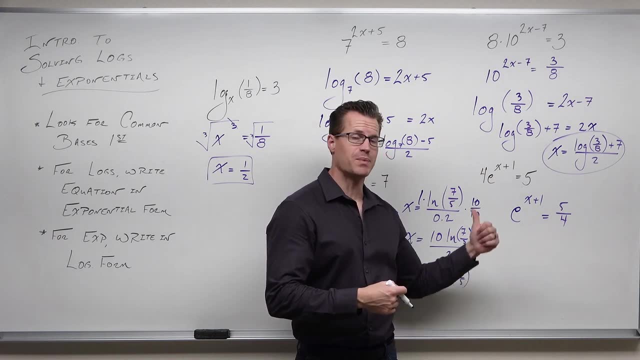 So when we divide by 4, we can easily see that that exponential is isolated. This is certainly not a common base. We're going to write this in logarithmic notation, So this exponential has a base of e. I'm going to need a logarithm with a base of e. 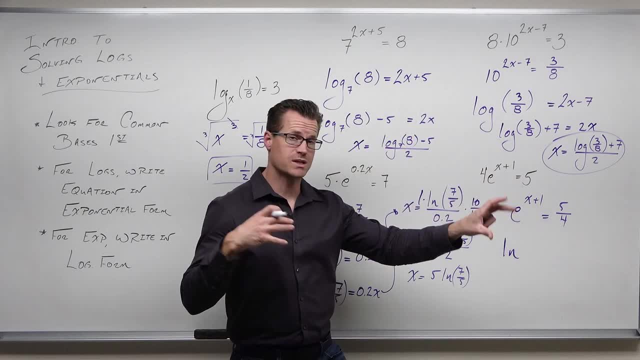 This exponential has an exponent of x plus 1.. Logarithms separate the base in the form of a logarithm from the base of e. So this exponential has an exponent of x plus 1.. Logarithms separate the base of an exponent of x plus 1.. Logarithms separate the base in the form of a logarithm from. 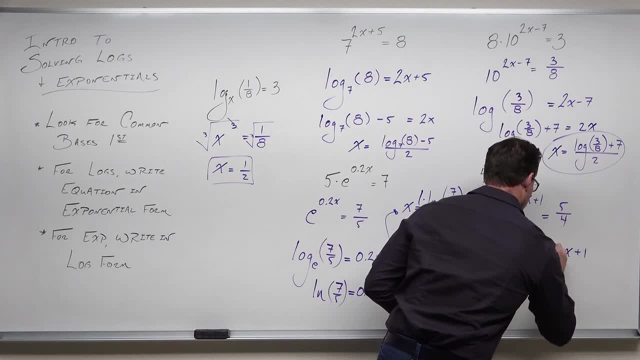 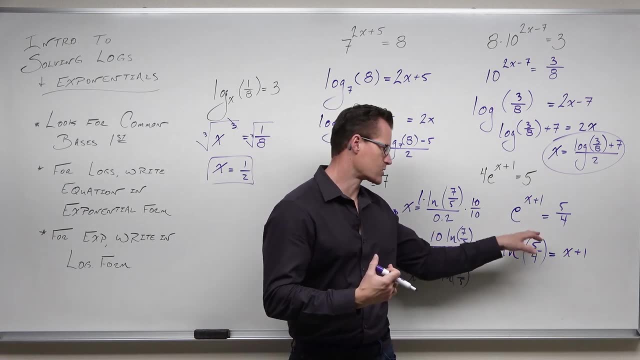 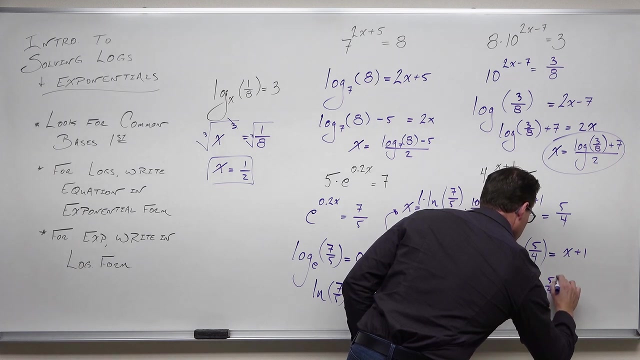 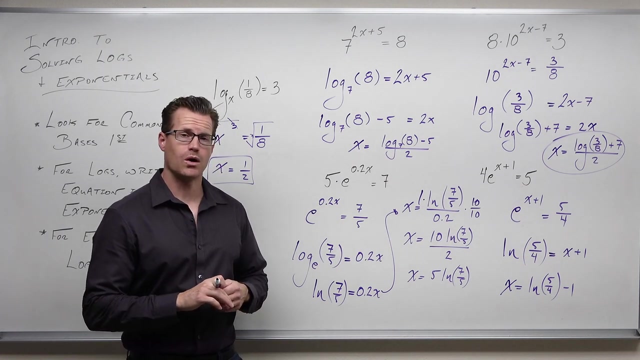 that exponent of x plus 1. And use as the argument of the logarithm whatever this exponential is equal to. After that we can solve for the variable and solve our exponential. So if we subtract 1, we're done. That's what's called an exact solution. Your calculator will also. 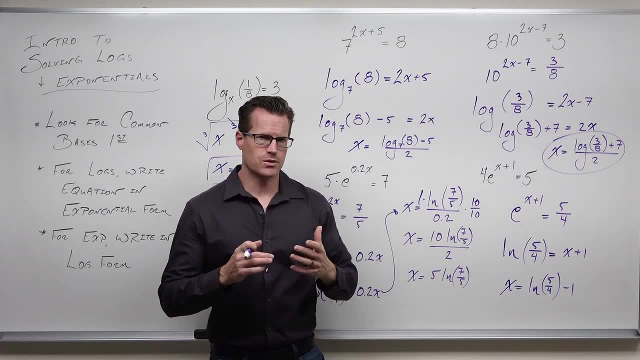 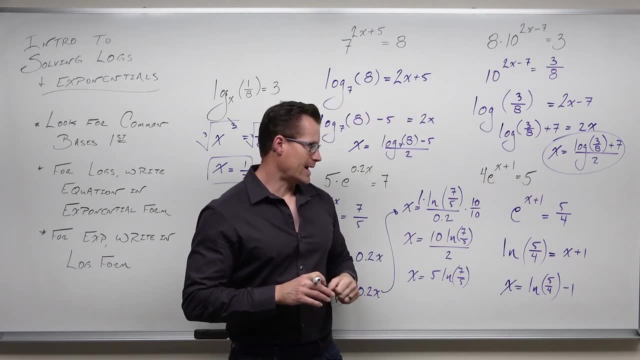 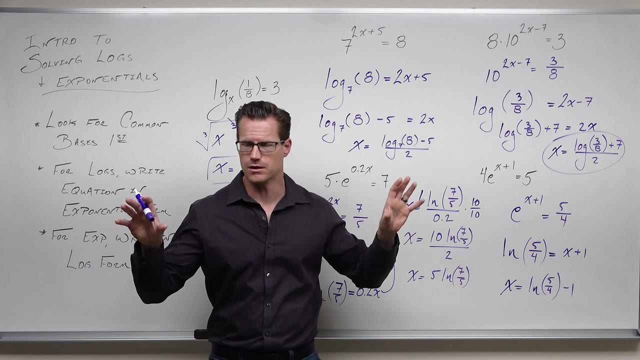 approximate this, which is why I wanted to give you these two, to show you that your calculator, that button that says log on it, represents a common log. that's what this is. that ln represents a log with a base of e. they're very, very, very common in our, our math. going on in the future. 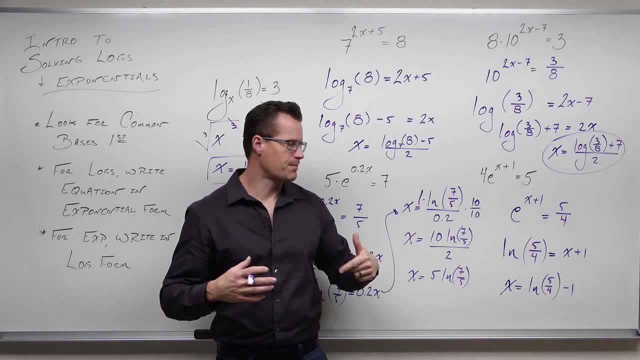 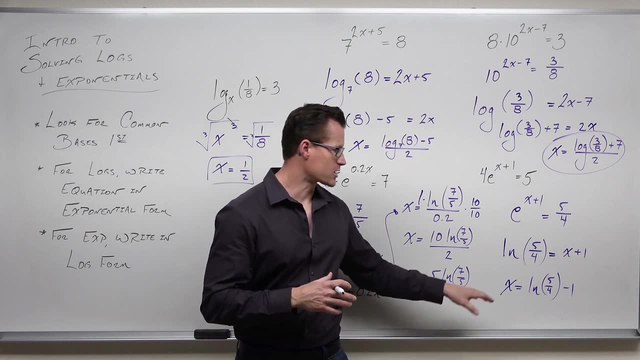 we have so many lns so you can approximate that by pressing ln and you're going to see the parentheses. put five fourths, close the parentheses, subtract one and it'll give you a decimal approximation for that exact solution. i hope this video has made sense. i hope that you're. 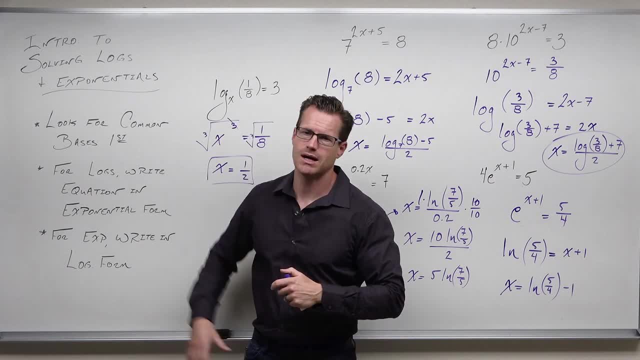 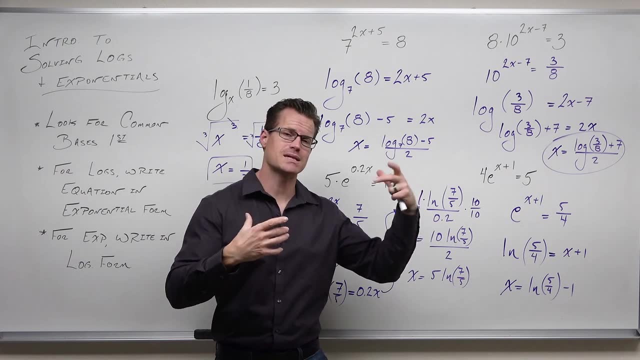 understanding like man we would. we'd certainly go through this process every time with logarithms. if you've got two logarithms of the same base, it becomes pretty easy. you set your insides equal. we're going to see that a little bit. if you have two exponentials and you can write the same base, 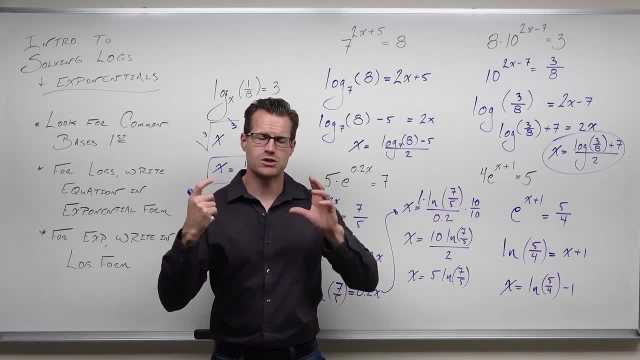 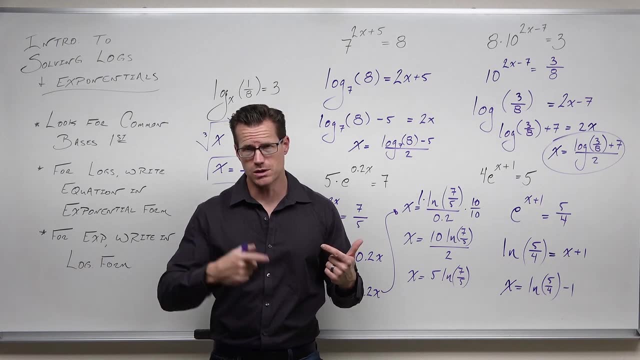 we've already done that. we model it with a couple examples a little bit earlier. you set your exponents equal. they're pretty easy to solve, but without those two very special cases it is going to require you to use an exponential to solve logarithms. you just take your logarithm, isolate. 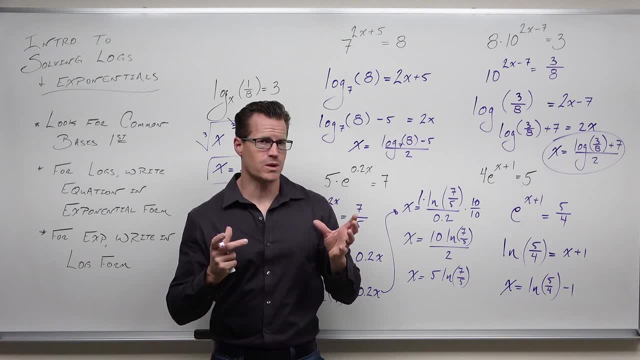 it and then use an exponential to represent the situation. put your exponent and your base back together and equal it to your argument. it'll solve very nicely. if you have an exponential, you're going to need a logarithm. there's a few ways i can show you how to get there, but in general,